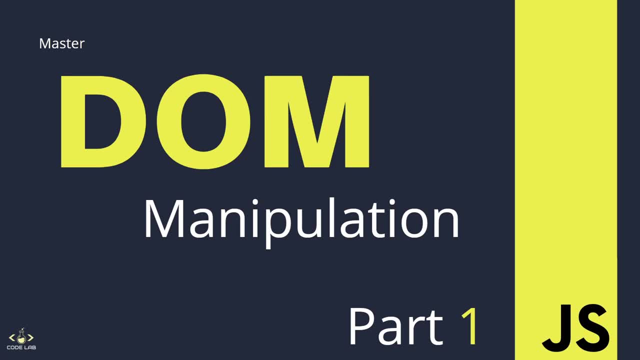 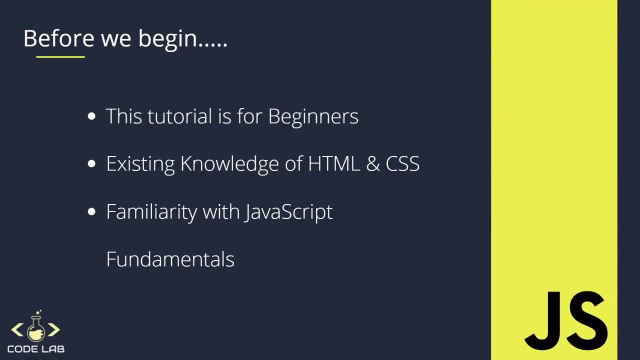 and in the second video we're going to be using everything we learned in this video and applying it to practical examples ranging from beginner to master level. So just before we begin, we're just going to take a look at a few prerequisites. So this two-part tutorial is primarily for beginners. so if you've never heard about the DOM, or maybe you're a little familiar with it- 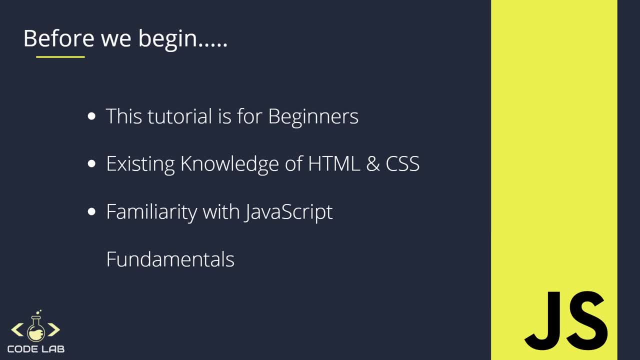 but don't know how to utilize and apply it. this tutorial is for you Now. in order to effectively understand the DOM and how it relates to working with the web, it's necessary to have an existing knowledge of HTML and CSS, and I have crash courses on both of those if you want to check this out. 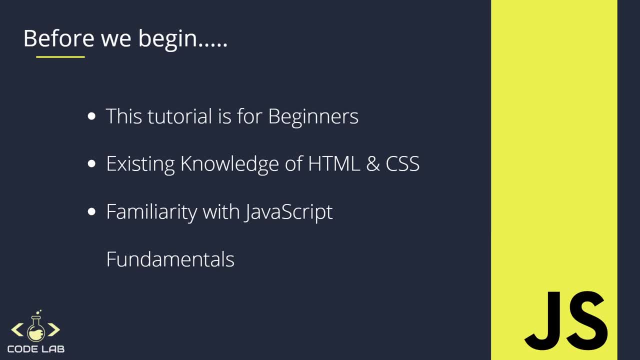 before you start this tutorial. It's also super beneficial to have a familiarity with fundamental JavaScript, so the syntax and the code structure. If you guys want to learn about fundamentals of JavaScript, check out my JavaScript crash course, which covers the fundamentals. So there's a couple of things you'll need if you want to follow along this tutorial. 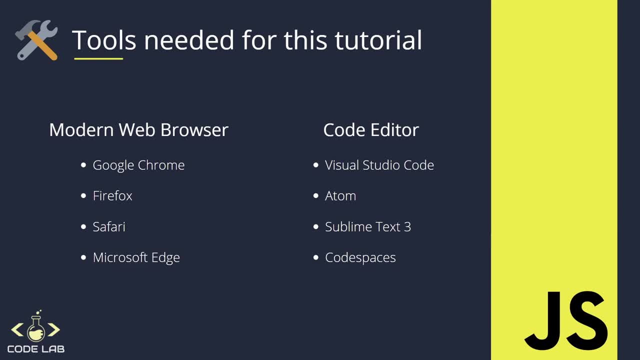 You're going to need a web browser and a code editor. Now, these are all the options you can use, and you can mix up these options if you like, but this tutorial I'm just going to be using Chrome and Visual Studio Code, but again, you guys can choose any combination you like. 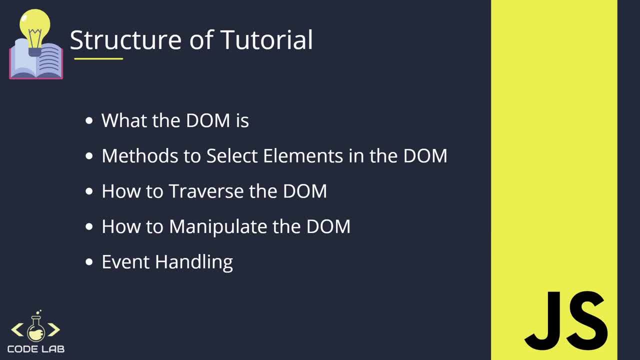 Now the structure of this tutorial. we're first going to take a look at what the DOM is. then we're going to take a look at methods to select elements in the DOM, how we can traverse the DOM, how we can manipulate the DOM. 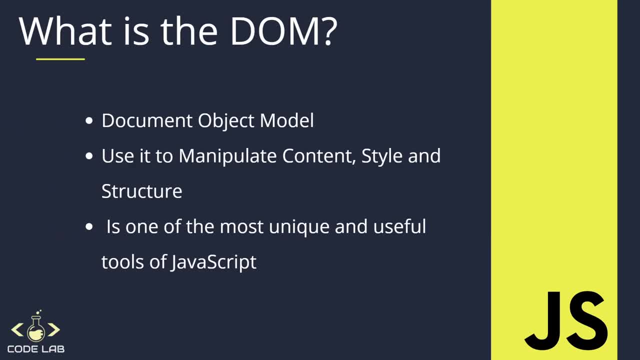 and then, finally, we're going to take a look at event handling. So we'll start this off by explaining what the DOM is. So the DOM stands for document object model. Now the document object is a built-in object that has many properties and methods that we can use to manipulate the content, the structure. 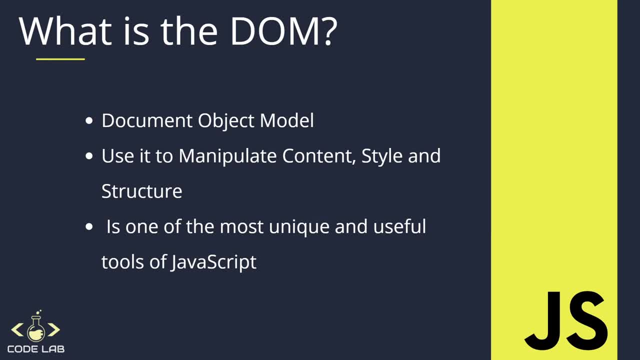 and the style of a project, And this ability to manipulate the DOM or the document object model is one of the most unique and useful abilities in JavaScript. So, almost any time a website performs an action, such as toggling a navigation menu or rotating between slideshow of images, or even displaying an error when a user attempts to submit an 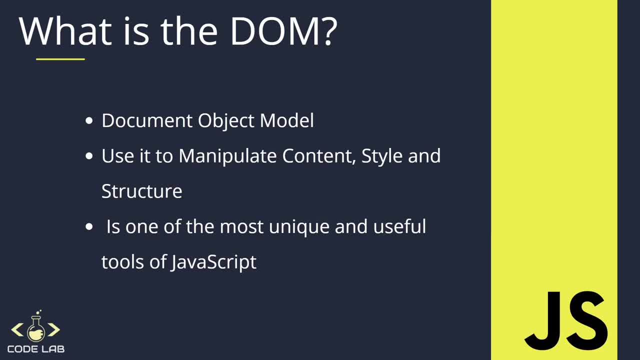 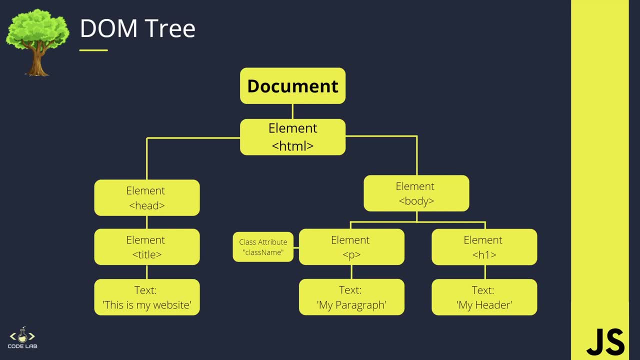 incomplete form. this is the result of JavaScript accessing and manipulating the DOM. Now, another way of thinking about the DOM and understanding how it works is thinking of it as a tree of nodes, like you can see on the screen now. So this is just a basic diagram of a DOM tree and all of its nodes. 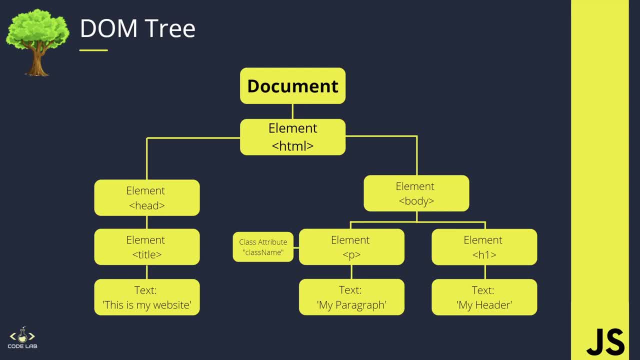 Now, everything in this diagram is a type of node: The elements, the attributes, the text content and even line breaks and comments- which we'll see a bit later on- are even considered nodes, and all of these make up the DOM tree. Now the DOM object itself is: 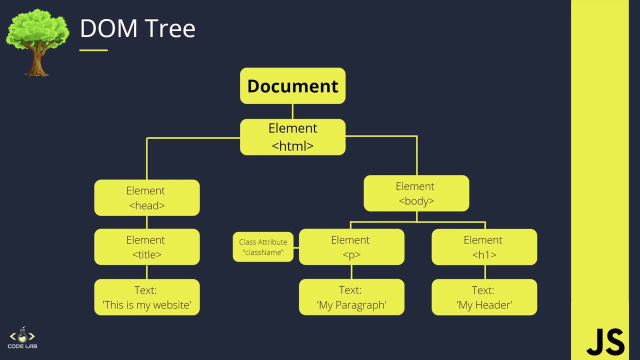 actually a property of the window object, which is the global top-level object representing a tab in the browser, And this window object has access to such information as toolbars, the height and width of the window, prompts and even alerts. But in this tutorial we're only interested in the document object. 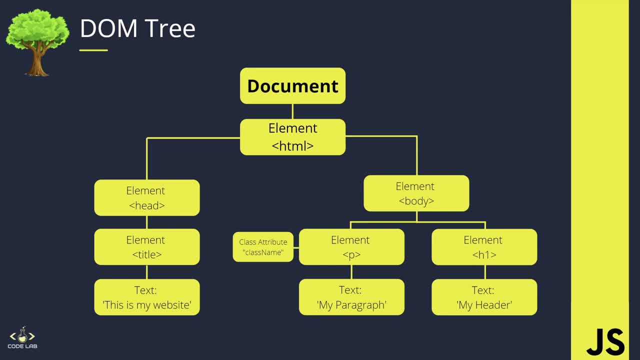 which is what is inside of the inner window and the stuff we want to manipulate. Now. another important thing to note here is that most of these nodes in this diagram have a parent-child sibling relationship. The topmost node, ie the document node here, is the root node of the DOM tree. 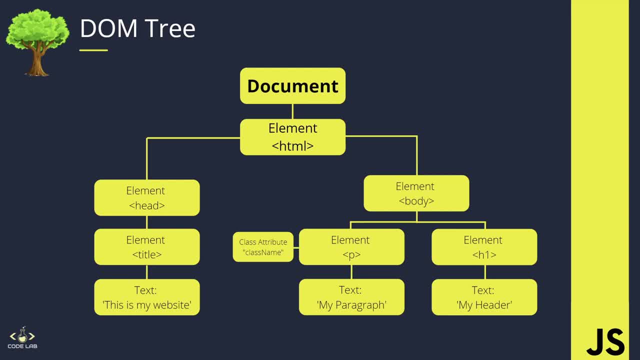 which we use to access the DOM and manipulate all of the content. Now, this document node has one child node, which is the HTML element, and the HTML element is a parent node to the head and the body elements. Now the head and body elements are what you would call siblings, since they're on the same level in the DOM tree. 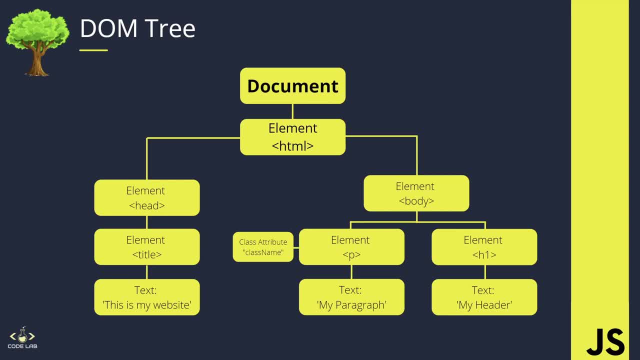 Underneath the head element, you see it has one child node, which is the title element, and the text this is my website is a child node of the title element. And these relationships are similar over the other side where the body element is the parent to the paragraph and the h1.. 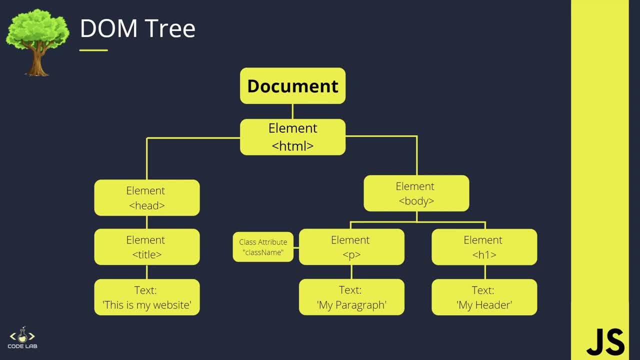 The paragraph and the h1 are siblings to each other and the text content inside each of these elements are child nodes to the paragraph and h1. So the my link and my header are child nodes to the h1 and the paragraph element. Now we can also see by the paragraph tag. we have a class attribute. 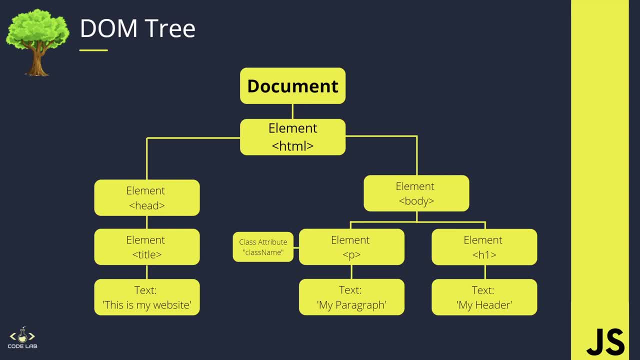 Now HTML attributes such as IDs or classes- in this case styles- etc. are also considered as nodes in the DOM hierarchy, but they don't actually participate in this parent-child sibling relationship like the other nodes do. The way they are accessed is through properties of the element node that they're contained in. 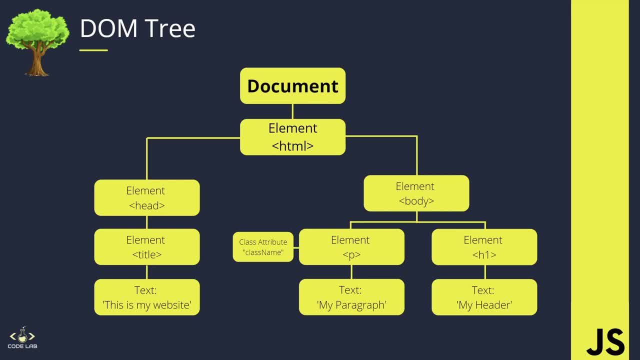 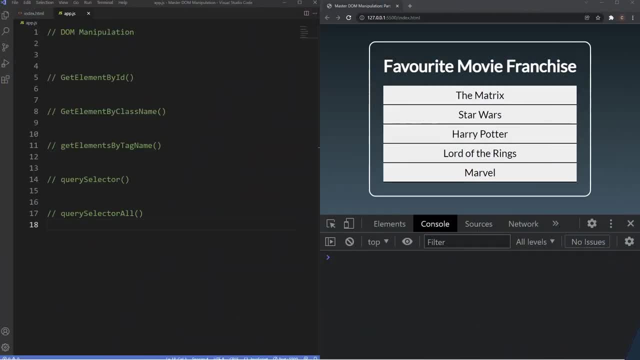 Now. often there will be times you want to move throughout the DOM, so understanding this parent-child sibling relationship is crucial to understanding how JavaScript works with HTML. I'm going to show you how to do this. Alright, guys, so now we know a little bit more about what the DOM is and learn about the DOM tree. 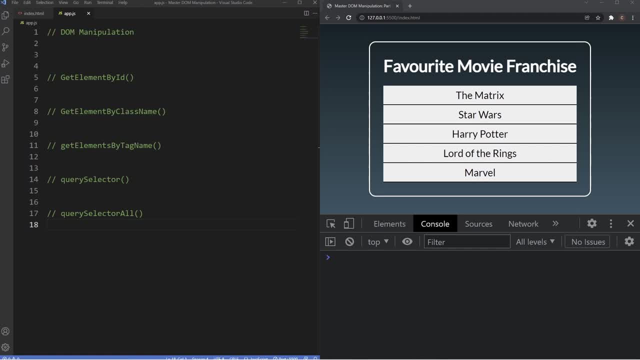 The next thing to cover in this tutorial is how to select these nodes or elements in the DOM tree for manipulation. So before we take a look at all these methods of selecting elements, let's just quickly go over the layout you see here in the browser, So in the indexhtml file. 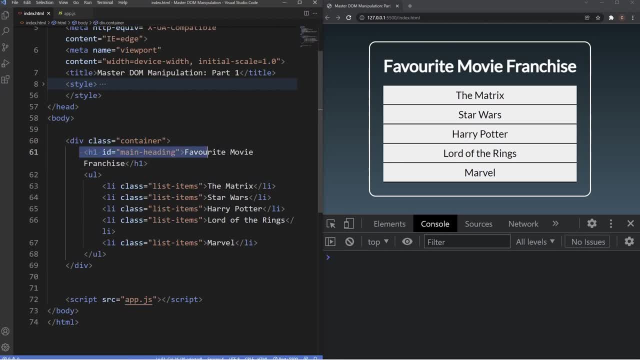 we've got a div of the class of container. Inside of that we've got a heading which has the ID of main heading and then the text of favorite movie franchise. Underneath that we have a ul tag which has a five list item Inside of it and then each of these list items have a class of list items. So super creative now. 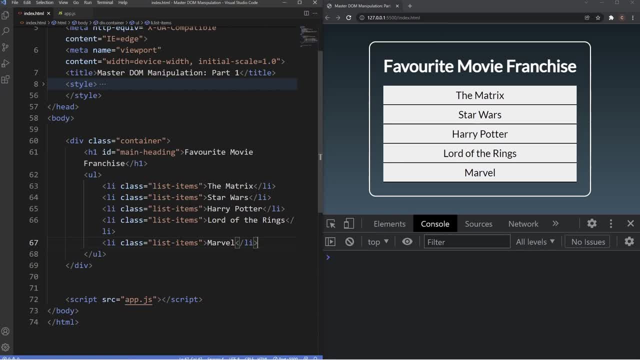 this is what we're going to be working on when we're looking at selecting and styling, traversing and Manipulating for the rest of this tutorial, and then, underneath that, we have a script tag Which has the attribute of source, and this is just linked to the appjs file. 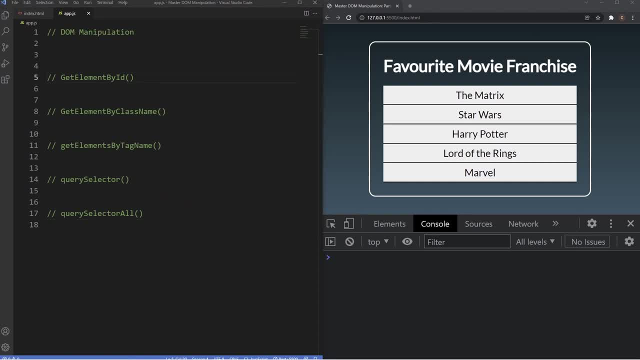 So again, guys, in order to be able to manipulate an element in the DOM tree, We first have to select that particular element. now, luckily for us, There's several ways we can do this, and the five major ways Of selecting the elements are the ones you see on the screen now. 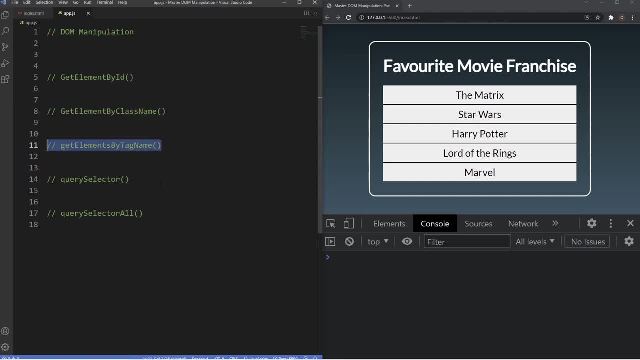 So we've got get element by ID, get element by class name, tag name, query selector and query selector. all Now. some of these methods are pretty self-explanatory, but we're going to go over each of them one by one now. 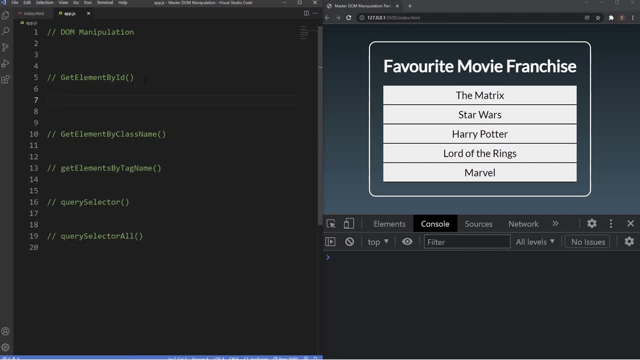 So the first one we're going to go over is get element by ID and, as you probably guessed, you can select an element using this method by its unique ID. and this is the easiest way to find a HTML element inside the DOM tree because, as we know from CSS, the ID attribute is used for some. 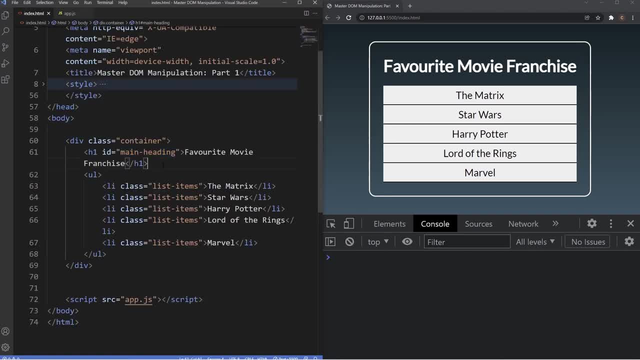 unique. now, if we remember back to the HTML file, you can see that we've got the h1 here, which you see in the browser has the ID of main heading. so this is the element we're going to be selecting. so first we need to select the document. 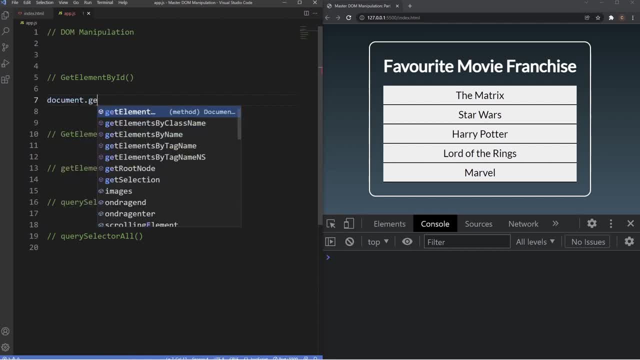 object model, which is just simply document. then get the method of get element by ID. single quote marks- really important that you include those- and then we're just going to grab the ID which is main heading. close that off. now what we can do with this selection is actually place it inside a variable. so 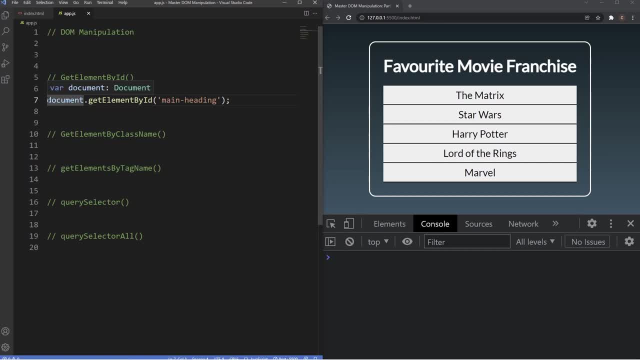 we can manipulate it. so we're gonna go at the front here and just say const title and we'll set this to the ID of main heading. and if we log this into the console now, so we're just looking title, you see, it shows up on the console now. 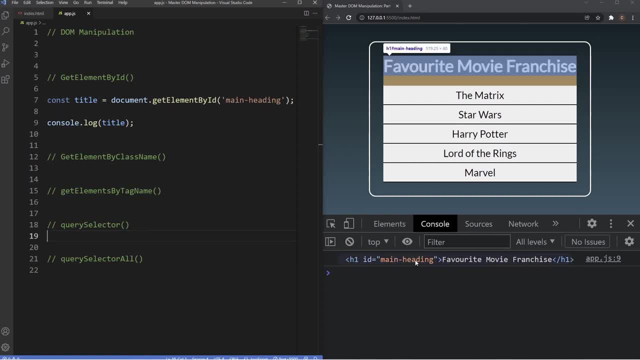 and if I hover over this you can see it highlights in the browser there. so you know, now we've selected this element and then what we can do from here is now select that variable we just created for the element and we can add stars to the element. manipulates attributes, traverse the. 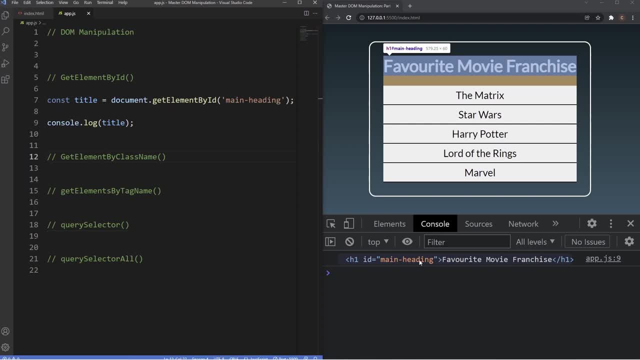 element, and then we can add the element to the element, and then we can add the element. so all of that good stuff which we'll be looking at in just a moment now. next, we have the element by class name. again quite self-explanatory, this method. 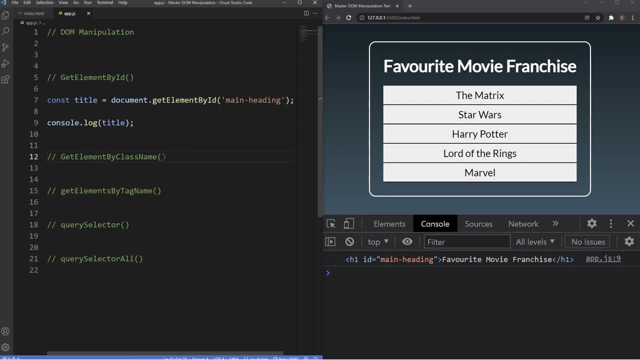 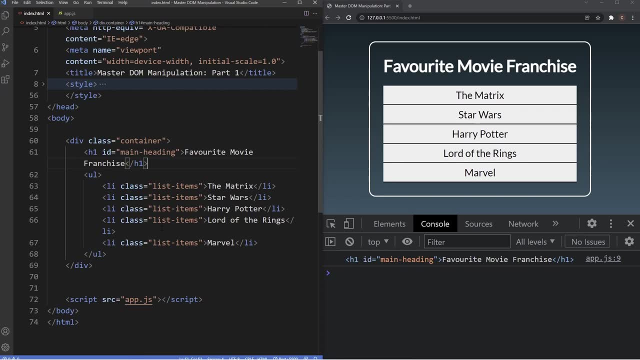 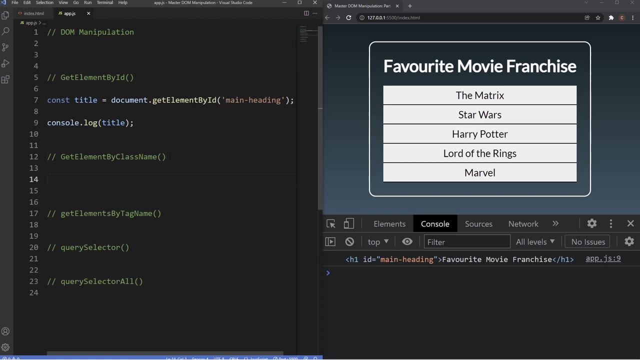 returns a collection of all the elements in the document with that specified class name. so, for example, in our HTML file here you can see all of our list items have that really creative class name of list items. so we can select all of these using the get element by class name method. so we'll do the same thing. 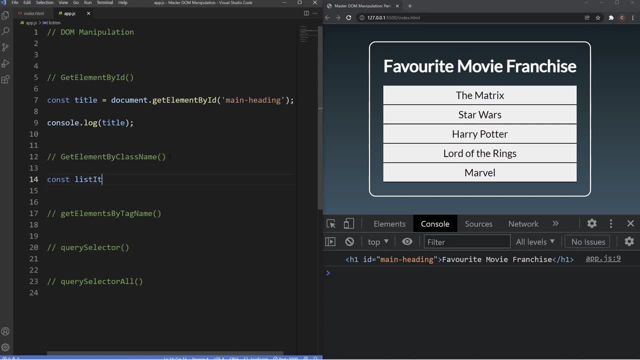 we'll put it inside a variable, we'll just say list item and we'll set it to the document. we'll say get element by class name, put single quote marks in there, and then we'll just say list items. I think it's items, yes, items. and then we'll just log this in the console so we know we've selected. 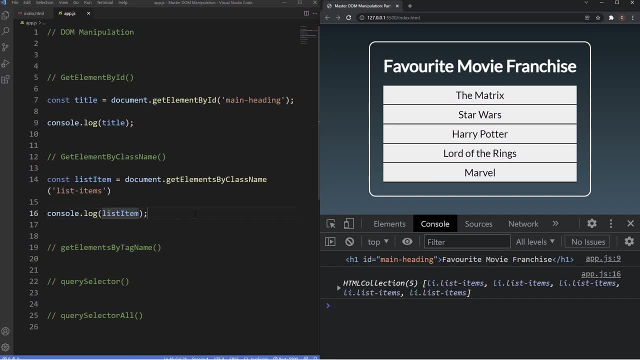 that element or these elements and, as you can see, using the method of get elements by class name, we've now selected all of those elements. now this method actually returns an array, like object, of all the child elements which have all the given class names. so if we open this up, you can see it's indexed and they're in the order that. 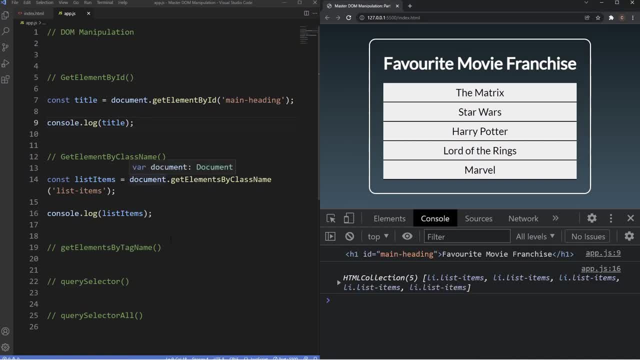 they are in the HTML file. now, the next method here, which is get element by tag name, is pretty similar to the get element by class name, in that it accepts a tag name and returns all of the elements of that specified tag name in the order in which they appear in a document. so again returning an array. 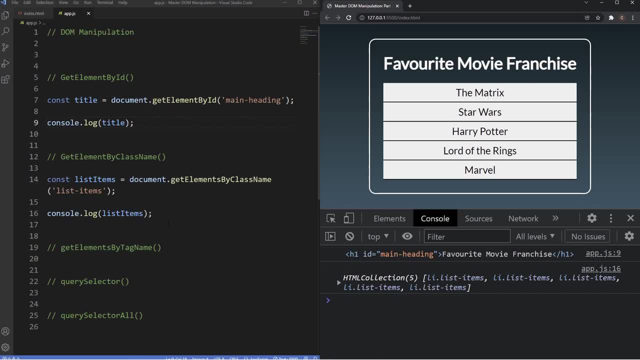 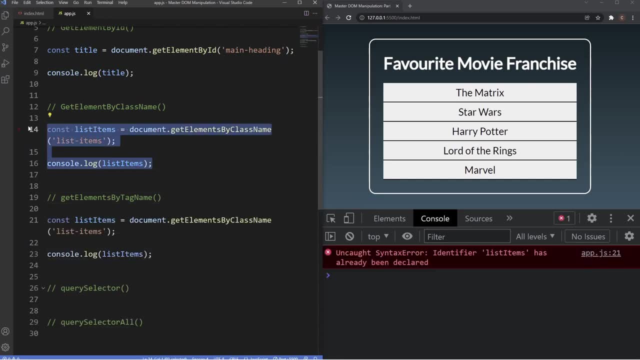 like object for all the child elements with the given tag name. so for this example, all I'm going to do is just copy and paste the name example, comment this out and then we just say tag name. and because the list items are list items, we just type in li. and if we take a look at the console now, 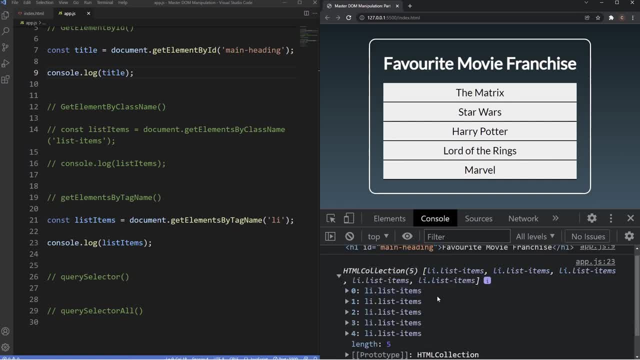 you can see it's got that HTML collection of all the five list items and they're all indexed in the order that they appear in the HTML file. so you can see this method is pretty similar to the get element by class name method. now the query selected. 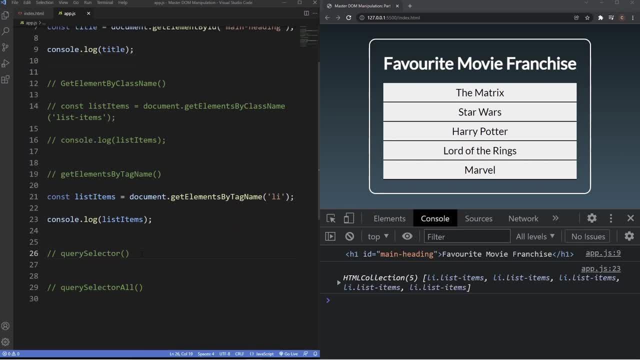 method that you see here is used to select one item, or the first item that matches the selector it's given. so if you have multiple items with the same class, name or the same ID or even the same tag, it will select the first one it comes across. so the beauty of this method, as you probably just 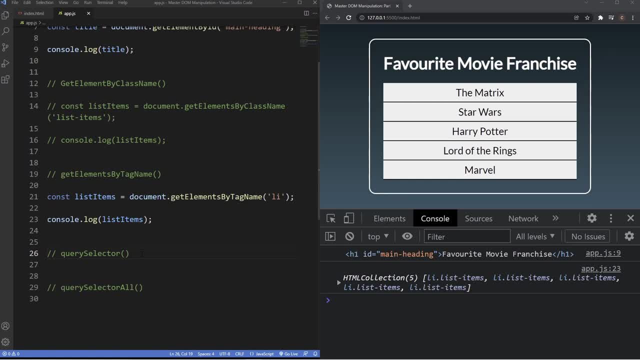 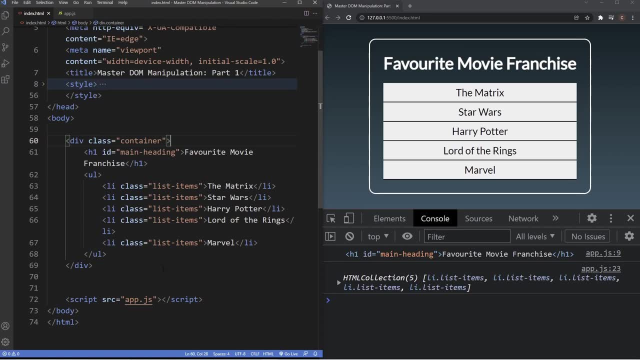 guessed is that it can accept all CSS style selectors, again, allowing it to select it by its tag or its class or even its ID, so we can actually use this method to actually grab any element in our HTML file here. so what I'm going to do is use it to grab the div of the class of 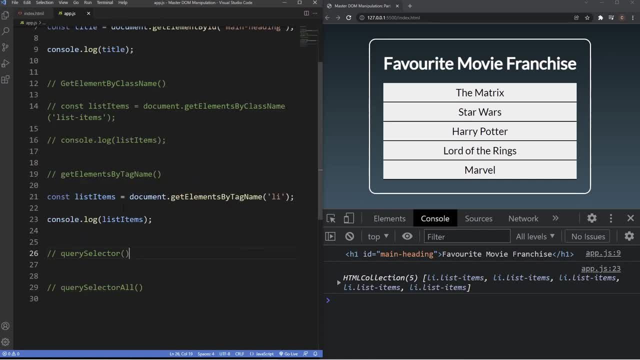 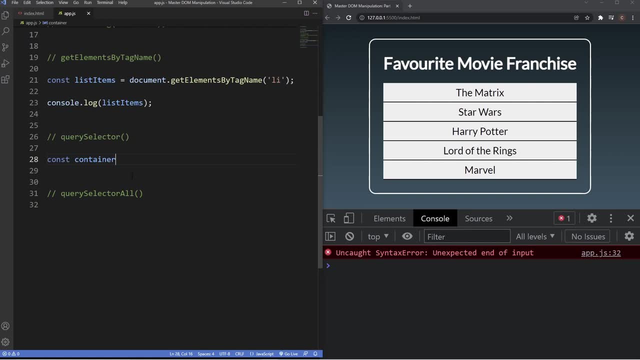 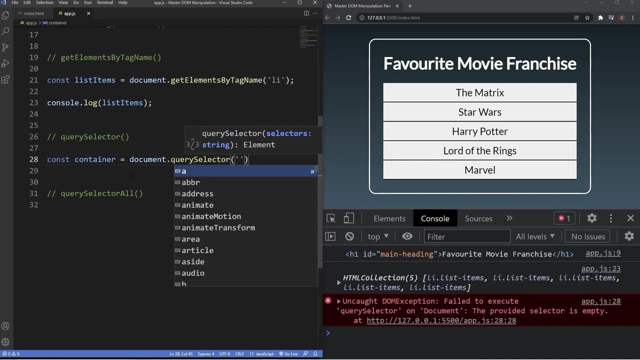 container which is acting as a container for the rest of the content. so, uh, we'll just go on the new document and we'll create a variable and we'll keep it super creative and call it container and we'll grab the document and then grab the query selector method and again, with this method we can 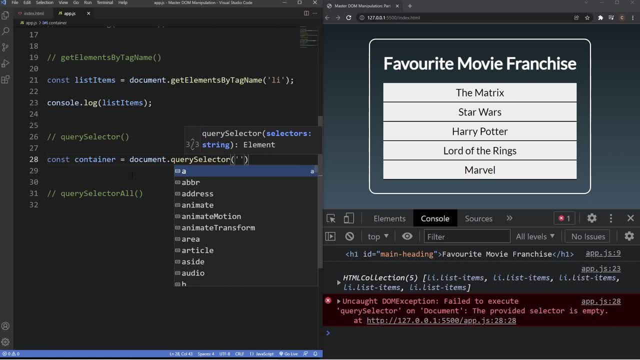 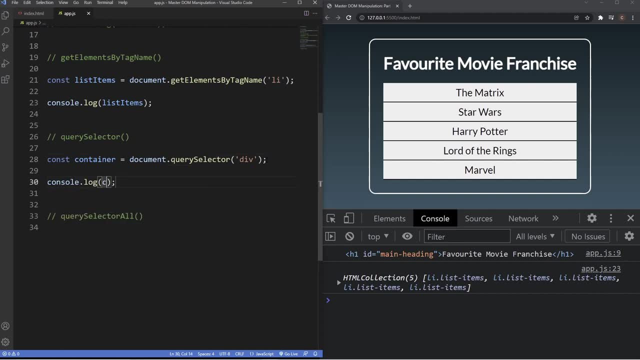 grab the div tag, or we can grab the class name or, if had an ID attribute, we can grab that. instead, what we'll do is grab the div tag and then just log this into the console so we know it's working and, as you can see in the console now, using the query selector method, we've selected that div of. 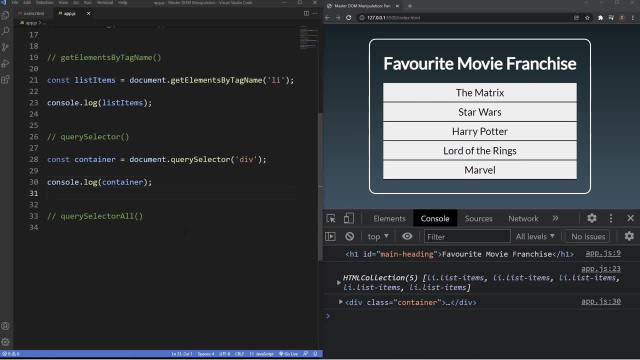 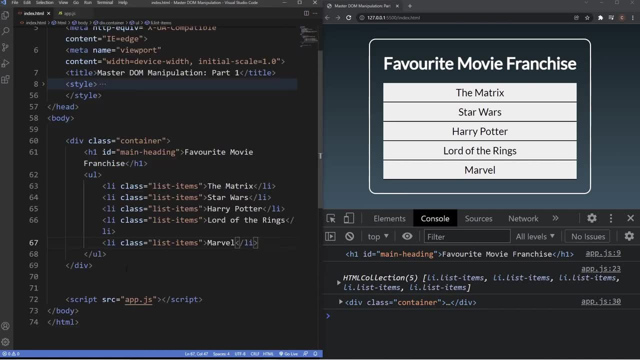 container. now, as I just mentioned, when we're using the query selector, it selects the first item that matches the selector. it's given which, in this case, is the div. now, if we go into the indexhtml file and we use several more divs again, it's only going to select this first div here if 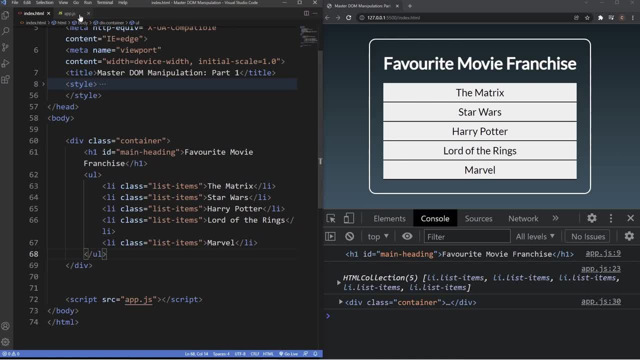 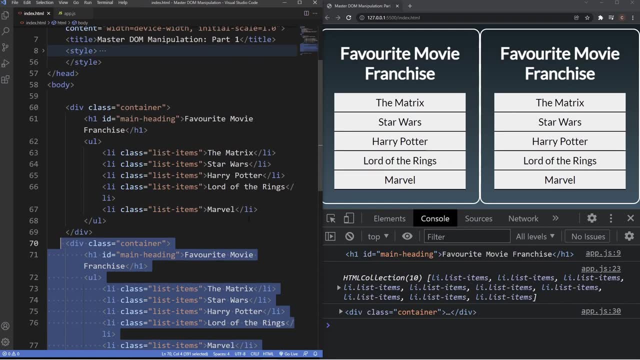 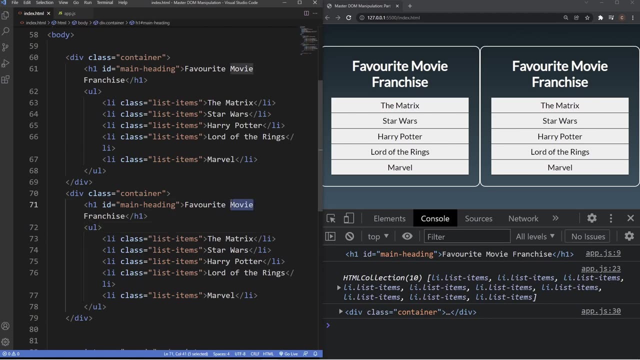 we had more divs in this example and we're going to select them all. we then use the query selector all instead. so, uh, what I'm going to do actually is just duplicate this one more time, just zoom out a bit. uh, just going to change a bit of the word in here. so favorite sports, and I'm not going to. 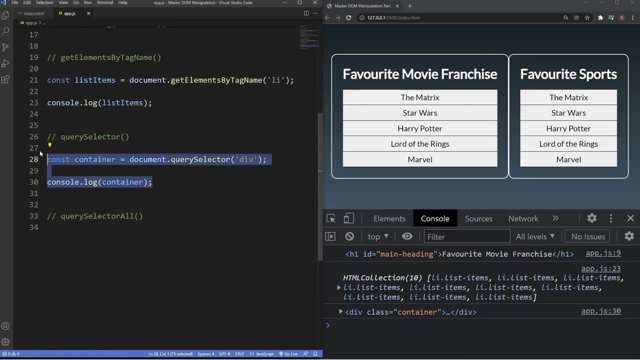 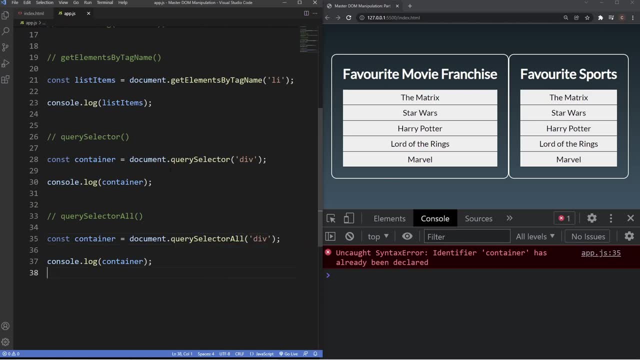 bother changing the names here, but just to show you guys that it selects all of them, I'm just going to copy and paste this, but instead of query selector we're going to say query selector all, and then comment this out and quickly just comment all these out, so we can only see. 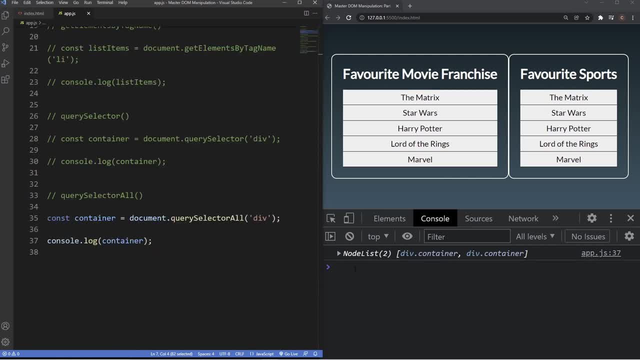 that variable there and if you take a look at the console now, you can see that this method returns a node list of collections of all the matching elements that matches that specific CSS selector, which in this case is a div, so similar to the get by tag name and get by class name, where 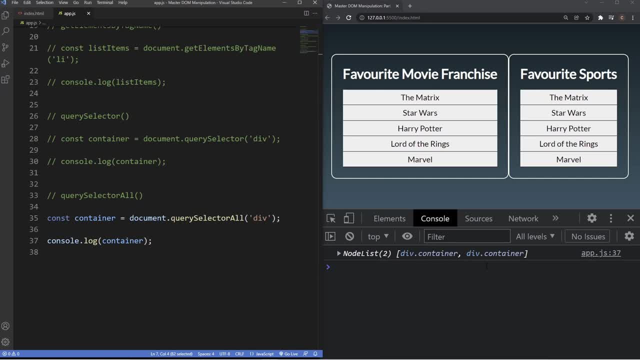 we get a HTML collection in this method, we get a node list and, as you can see, it's selected both of the containers because, unlike the query selector with query select at all, it's selecting all of the divs in the indexhtml file. so that's how we can select elements with the query selector. 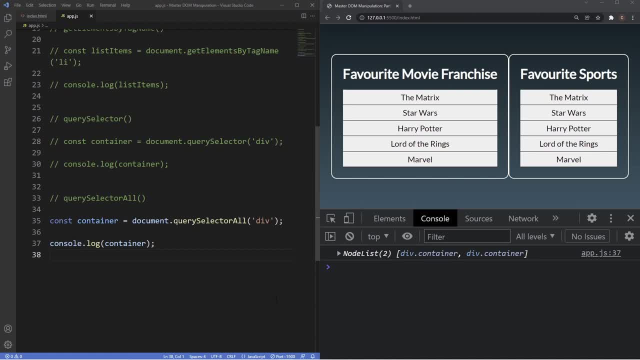 and the query selector all method. so, to quickly summarize this section, when you need to select a element, you have five different options to choose from, five different ways of essentially doing the same thing, which is selecting an element or elements. personally, I primarily use query selector and query select at all, because these methods select elements through CSS selection and I 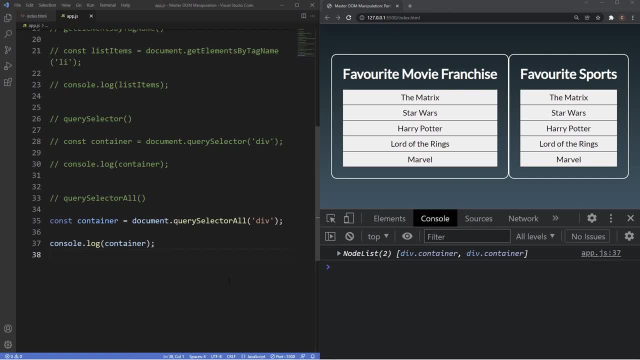 primarily use this to select IDs and classes, mainly because these CSS selectors provide a really powerful and efficient way of selecting HTML documents, especially IDs, because you likely understand that elements shouldn't have the same ID, that the ID is a unique identifier of the element. so, with that in mind, selecting the element with its ID is a safe bet, because you 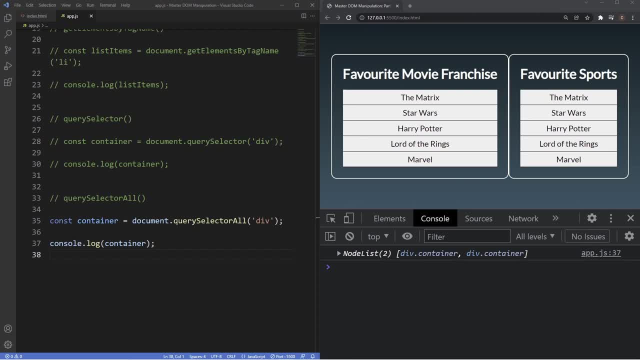 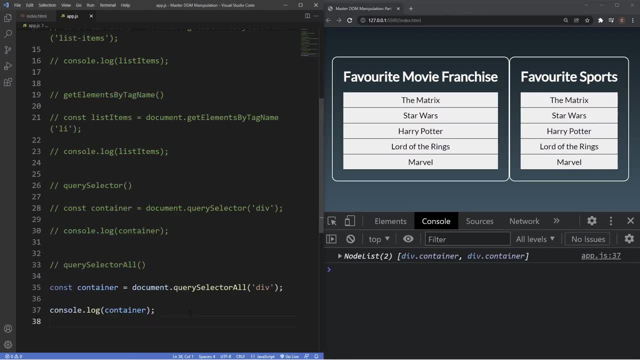 wouldn't go and apply a manipulation to different elements, unless perhaps that's what you want to achieve. in that case, the query select all method and the class selector is what I typically use. so now we know all the different methods that we can use to select an element in the DOM tree. we 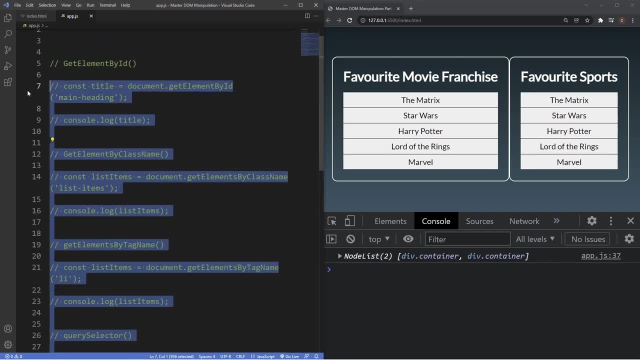 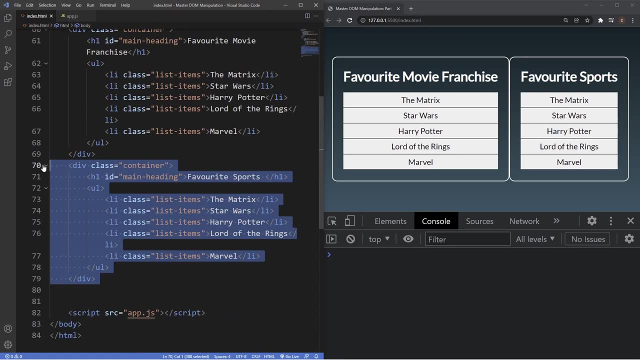 could finally start doing some manipulating now. so, firstly, what we'll do is just get rid of all of this content here and then head in the indexhtml file and just get rid of the second container, because we don't really need it. so let's start things off by taking a look at how we can change. 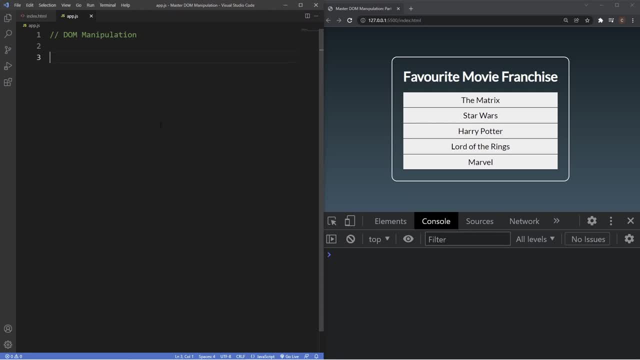 the styling of an element. so if you are familiar with CSS and CSS properties, we have a way we can access these properties in JavaScript. so the first thing we'll do is just select this main heading which we have in our indexhtml file here, which is just the title of the container. 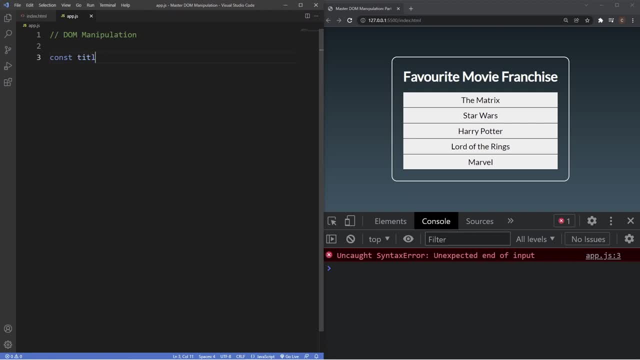 so we're going to put that in a variable and we'll call this variable title and then document query selector method and we'll grab the ID of this element, which is main heading. oh need to put these in uh single quote marks and then let's just log this in the console so we know this variable is working. 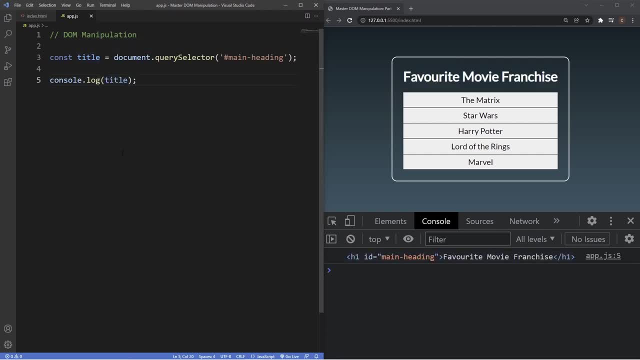 and, as you can see, now we've selected this element and stored inside the variable of title. so what we can do now is actually manipulate the styling of this element and change it around using CSS properties. so to access CSS properties in JavaScript, we'll just first grab the variable. 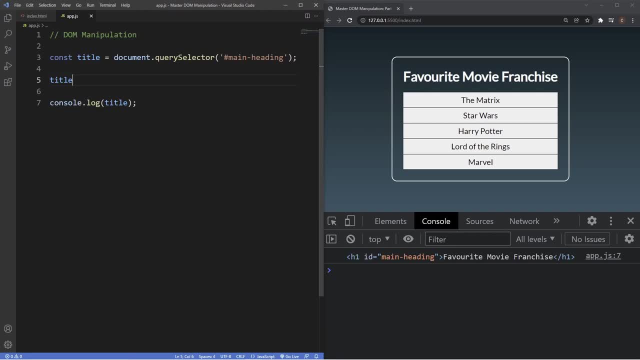 that we want to apply the style into which, in this case, is the title or the main heading, and then we simply type in the style property and then, after this style property, you just use um, any CSS property you want to apply to this element. so what we'll do is just change the color. 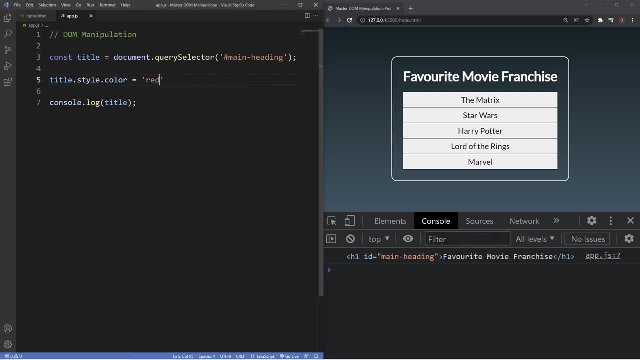 of the text, and we'll set this to- uh, let's say, red. and, as you can see in the browser now we've changed the color of the main heading from white to red using the start property and then the CSS property of color. now this type of styling is what you'd call inline styling, and there 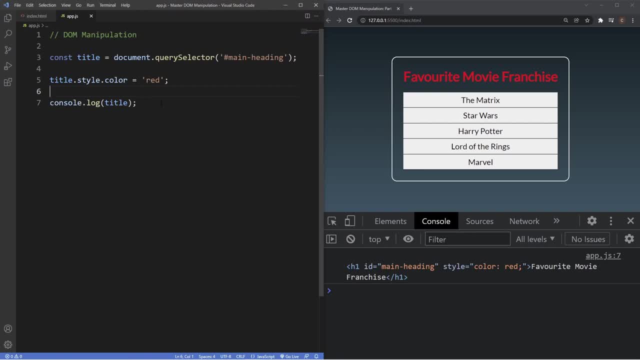 methods to style elements and with javascript, but this is probably the most direct method. now again, if you take a look on the console, you can see it's actually included the style attribute again, because this is actually done through inline styling. now it's important to know this because 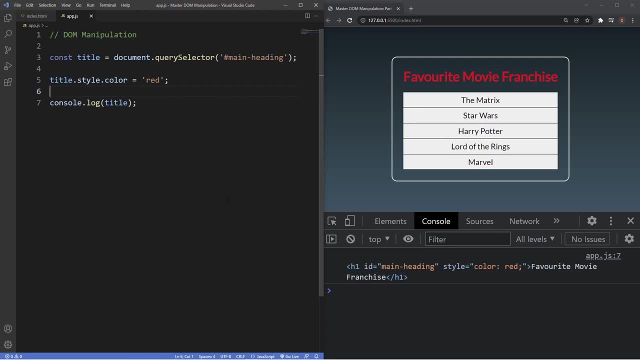 with inline styling. this actually only works on a single element. if i tried, let's say, applying it to all of the list items here, this wouldn't actually work, so just going to demonstrate that to you guys. so let's uh, create another variable and we'll call it list items and we'll 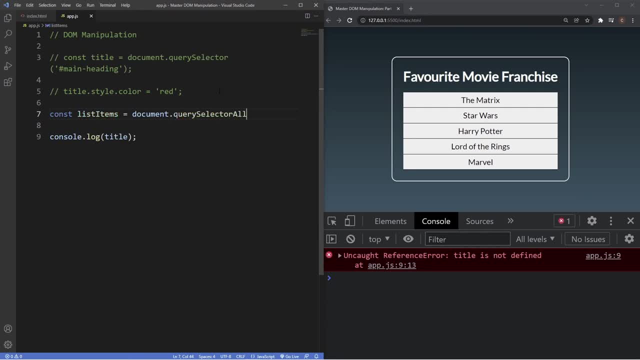 grab all of those list items with query selector. all they will have. they all have a class of list items and then let's just log in here list items. so you see, now in the console we've selected all of those list items. now let's try and use the 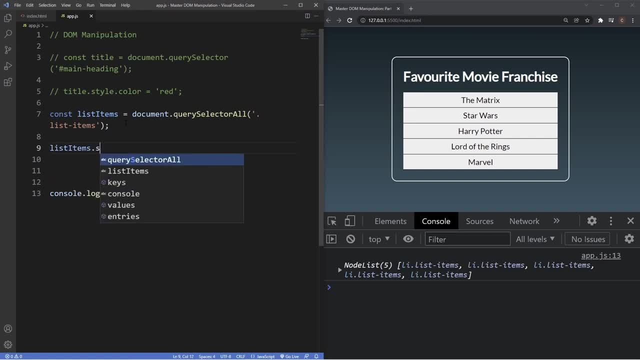 style property again on these list items and see if it works. so say style, let's say let's try and change the color again, or let's actually do the font size, and just quickly, guys. um, i wanted to mention that it's important to remember while using the style property. css properties are: 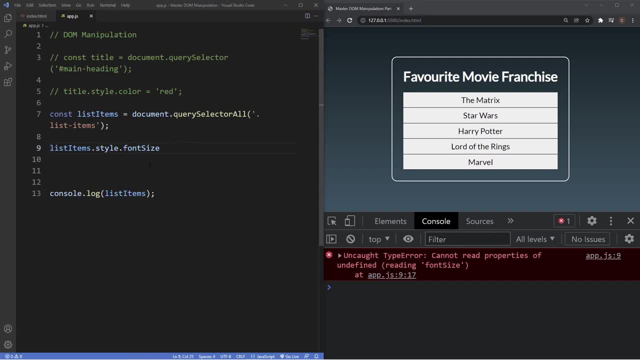 written in camel case and not with a more standard snake case which has the dash. so the camel case is essentially just a capsule letter. to begin the second word and any subsequent word is just a capital letter. to begin the second word and any subsequent word is just a capital letter. 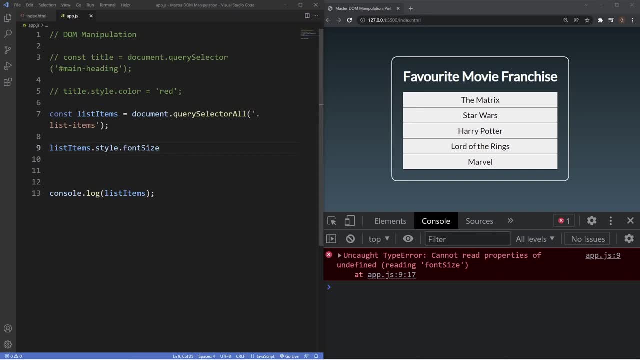 in the name or method or even a property font size. in css would be written like this, but in javascript we'll use camel case. so, um, just so you guys are aware of that. now again back to what we were talking about, if i try changing all of the um the font size of these list items here, so let's. 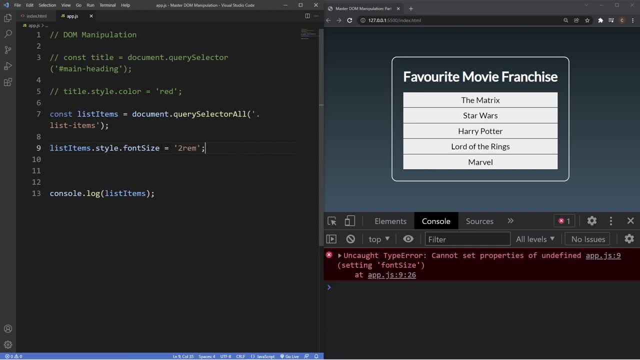 say to about 2rem. you can see this isn't actually working because it's trying to apply an inline style to five different list items, which wouldn't work if we actually wanted to apply this styling to all of the list items. we need to loop through the list items first, so just to show you, guys, how. 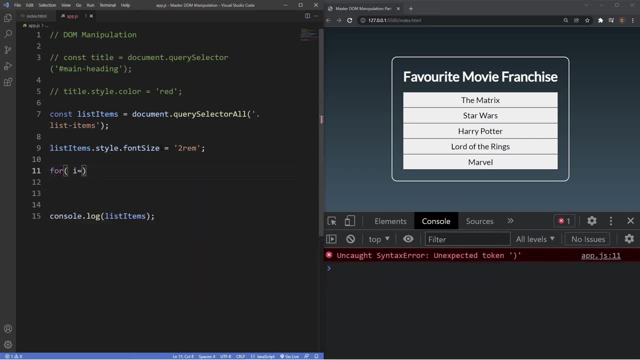 that would work. uh, we'll say i equals zero, and then, uh, we'll say i is less than the list items dot length, which just gives us the amount of list items inside of our um ul here, which is five. and then we want to say we want this to increment by one. 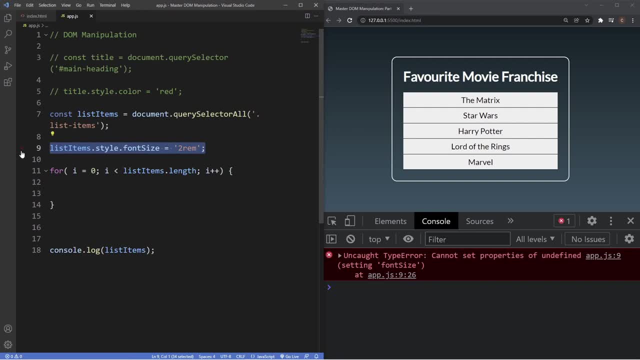 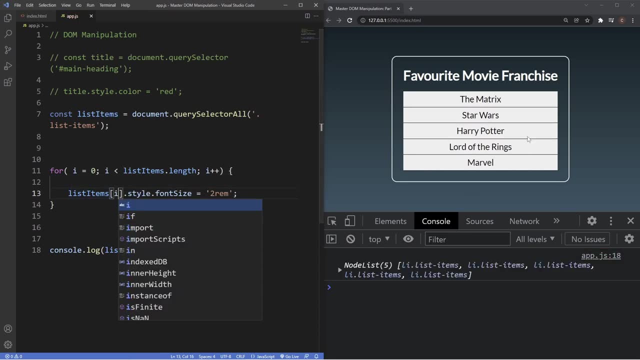 each time, and then what we do now is just apply this and put it inside of our for loop, and then we just need to index the i and, as you can see now, it was quite subtle, so let's just make it a bit bigger. you can see all of the list items now have that styling because it's been looped. 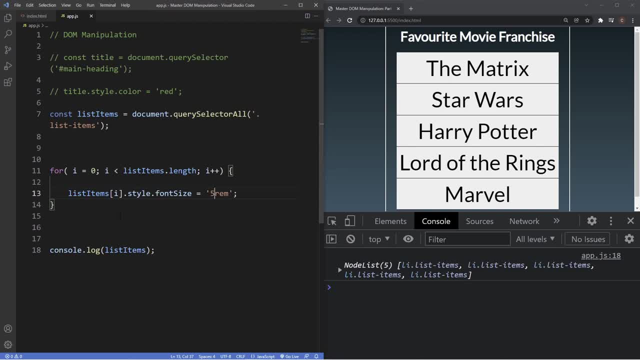 through using the for loop. so that's how we can apply inline style into elements using the style property or multiple elements if we loop through them. and the next thing i want to take a look at is creating elements. so what i'm going to do is just comment all the way through the list items. 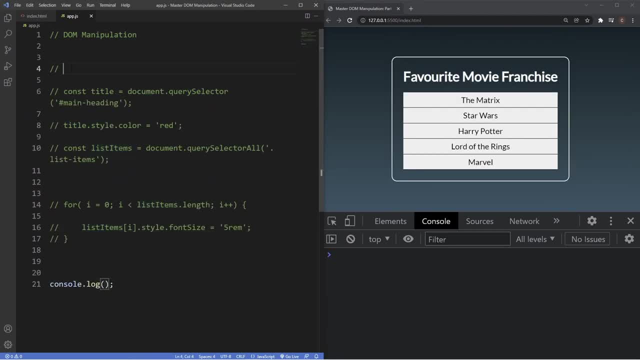 if we ever have any. oh, okay, so, and then we stop on some block over here. here's the rest of the elements already good, so i'm going to get rid of that. display elements. uh, just tear all of this out first. get rid of, uh, the list items there. i'm just going to put a comment here for styling. 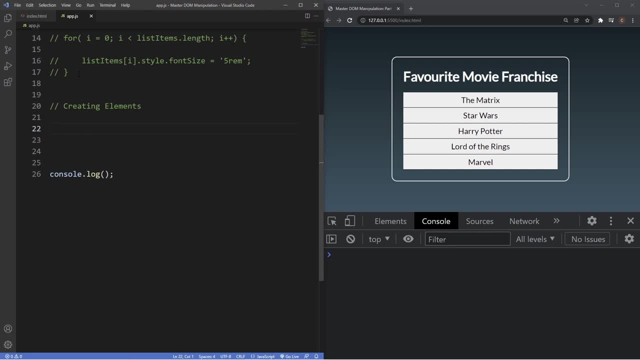 elements, and then now we'll do one for creating elements. so again, another really cool thing about dom manipulation is that we can create elements from our javascript file here, and we do that with a simple method, really, of the container. what we need to do first is just create a variable for the unordered list, because we need 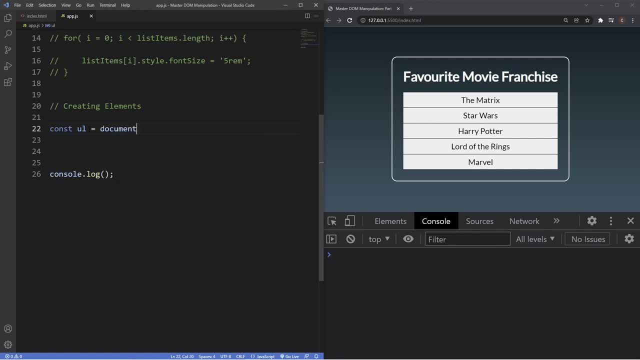 to enter this on order list. so we'll say: document query selector, grab the URL, and then we'll do now is use the create elements method to create another list item. so we'll just use another variable here- document create element- and we'll create a list item. now this isn't actually going. 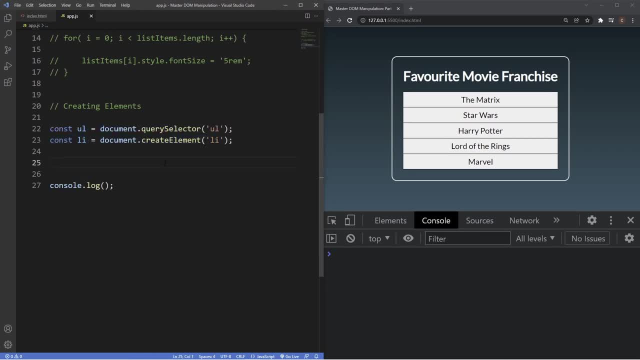 to do anything at the moment. this element we've just created in this variable here needs to be inserted into our document, and the way we can add elements inside of the document is using the append method. so what we'll do is first grab the URL, because we want to append this list item inside. 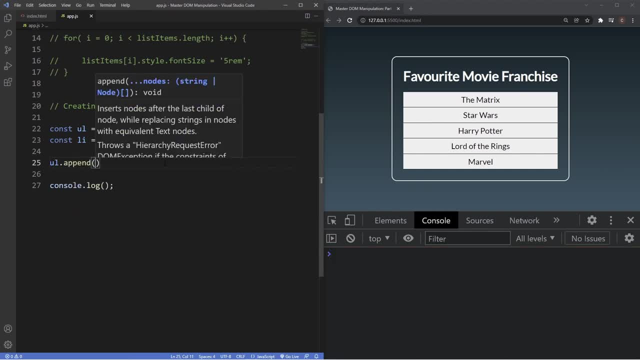 of this URL and then we grab the append method and the element we want to add is this one here we want to append, which is the variable of li, which, again, is just this list item. now, you won't be able to see it currently at the moment, but if we take a look at the document here and if we open, 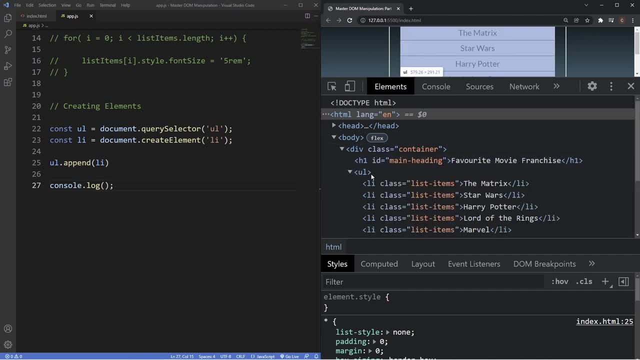 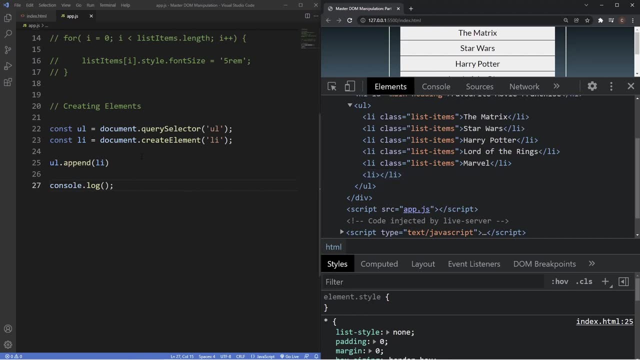 this up and then open up the div of the class of container. open up the URL. you can see there's an extra list item inside of this URL now because we've inserted this element now using the append method. now what we can do from here is add some content inside of our list item. so I'm just going. 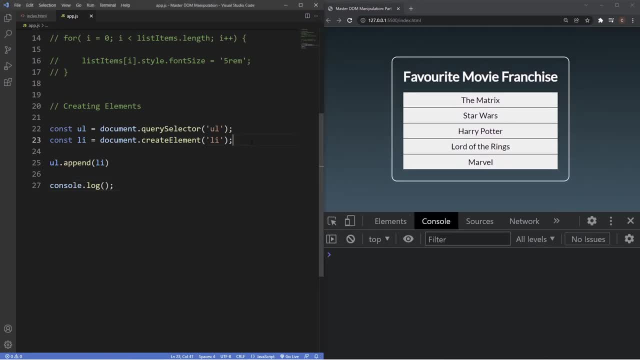 to bring this back down. come back in the console. I'm just going to put a comment here for adding elements and then after this we're just going to say, um, modifying the text. now we don't really need this console log anymore. so there are several ways. 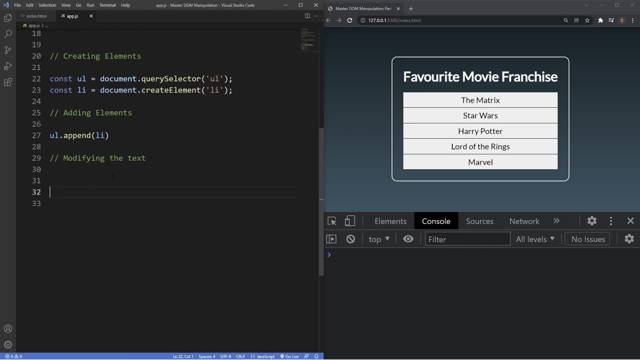 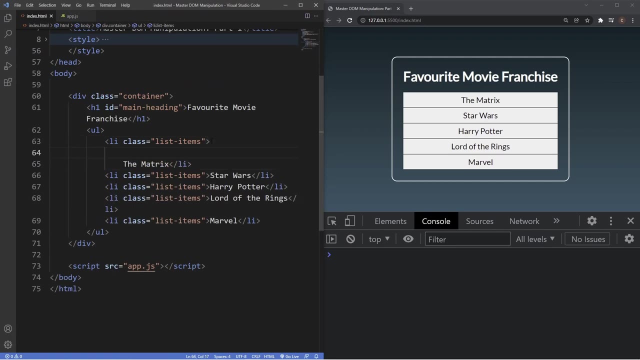 we can include text or modify text in our HTML, and those ways are in a text, text content and in a HTML. now there is a difference between three. so to demonstrate those differences, I'm just going to put another HTML tag inside of the first list item here. so I'm just going to put a span. 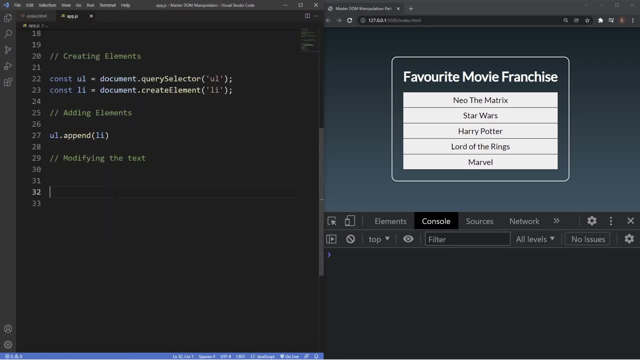 I'm going to put Neo, because that's relevant to the matrix, and then I'm just going to create another variable to grab that element there. so we're going to say first list item, so that to the document and say query selector, and then we'll grab that list item. 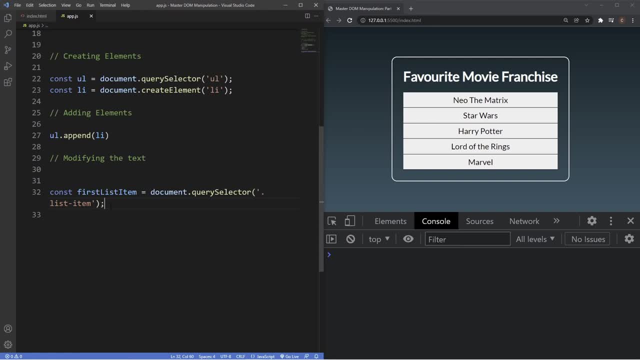 and then I'm just going to grab the console log- again actually- and put in here first list item. oh, forgot an s. so there's our first list item. now what I'm going to do here is include in our text first, so it just displays the text. duplicate this a couple more times. 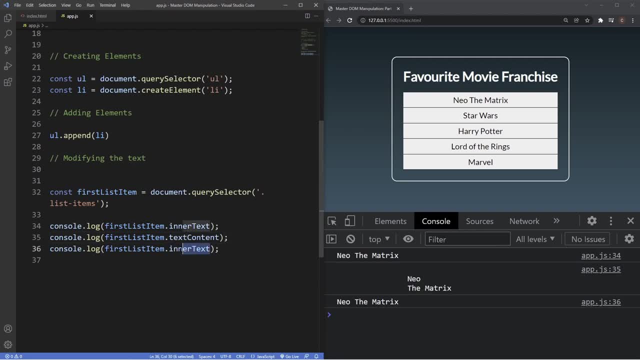 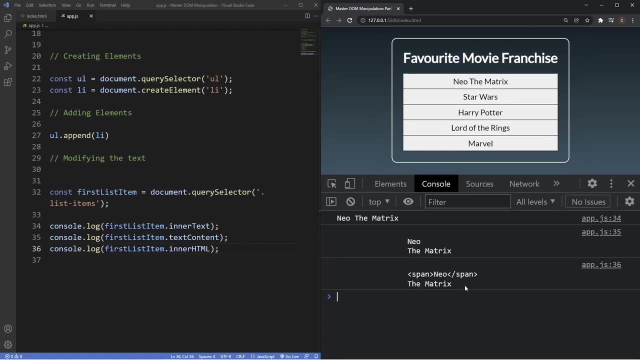 going to grab text content and then also grab in html. so if i just pull this up a bit more now, if you take a look at the console, you can clearly see the differences between the three now, and that is essentially just the way they're displayed. so within a text here you can see we're simply 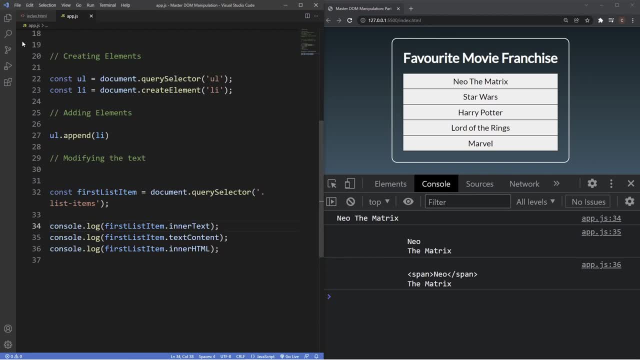 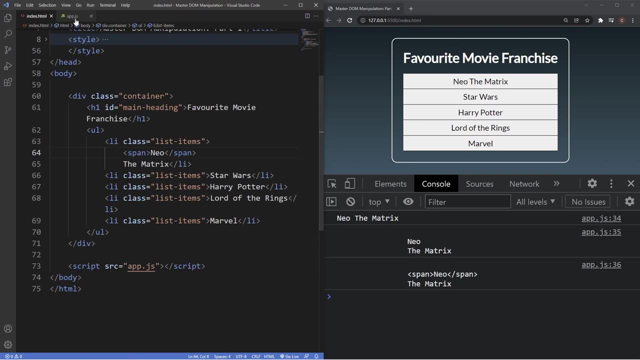 getting the visible text contained inside that node with text content. you see, it's actually being displayed the same way it is in the html file. so it's got all those indents and it's jumping onto a new line and with inner html, a similar sort of thing with the indents and 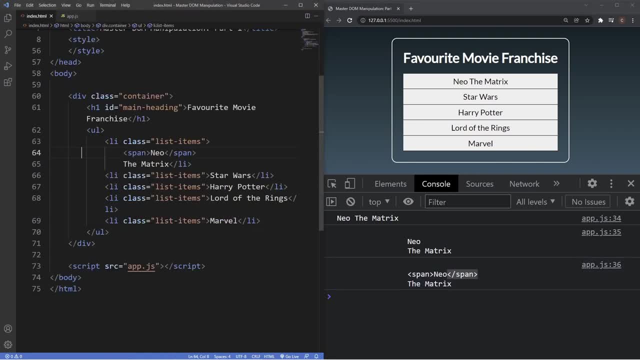 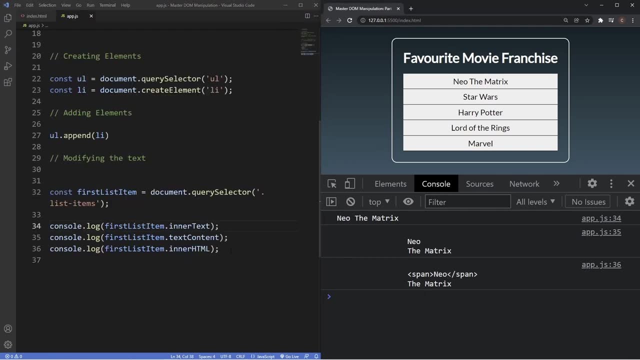 jumping on new lines, but it's also showing the tags, so showing us the span tags inside of our html here. so again, that's pretty much the differences between the three. now, another thing here is that within a html there is a bit of a danger using inner html, and that's mainly 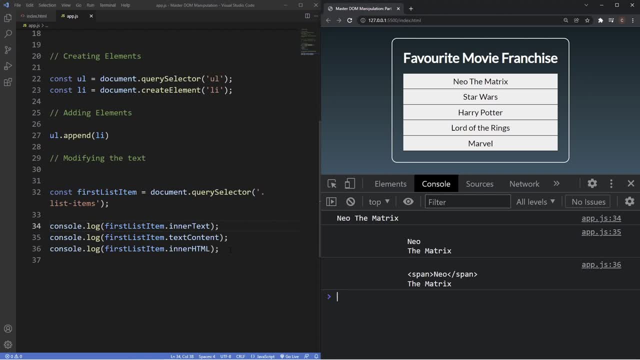 it's security issues. you don't really want user input to be displayed in the inner html, because this actually allows the user to control the javascript and the html on your web page, which obviously has its um problems there. so in most cases you're just going to use inner text, so let's go ahead and use that. 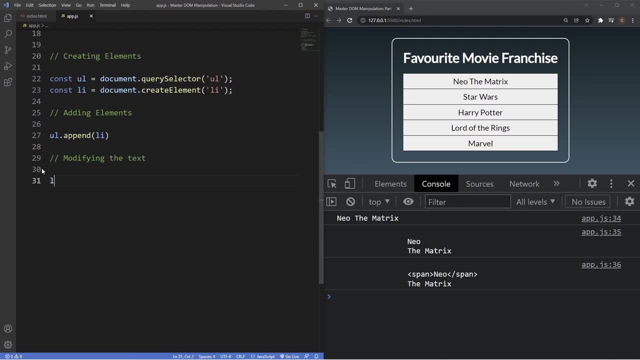 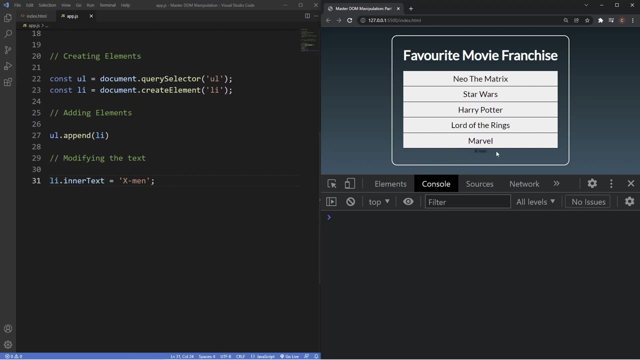 and implement that in our list item that we created. so we're just going to grab the li grab in a text and we're going to set this to equal, let's say, x-men, which is another franchise. if you take a look at the browser now, you can see that text has been included inside of our list item. 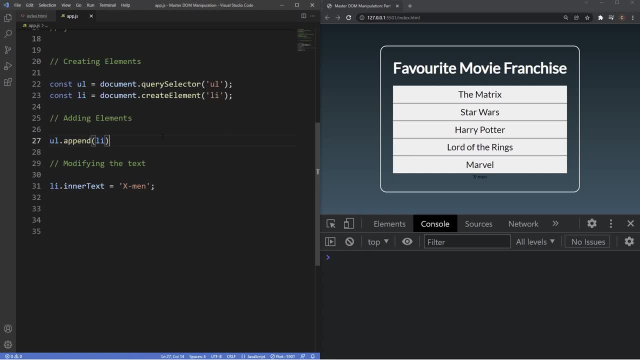 now. all right, guys. so we've created our list item here, we've added it into the ul using the append method, and we've also given it some text. the next thing i want to do now is make our list item look like the rest of the list items. so to do that, we're going to need to learn how to modify and manipulate. 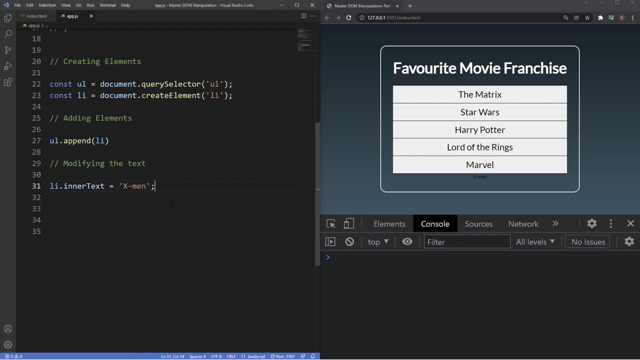 in elements, attributes or classes. luckily for us, javascript provides several methods and properties for adding, removing or changing a html- elements, attributes or classes. so we're going to go underneath here and just put a comment of modifying attributes and classes, and the first method we're going to take a look at is the set element. 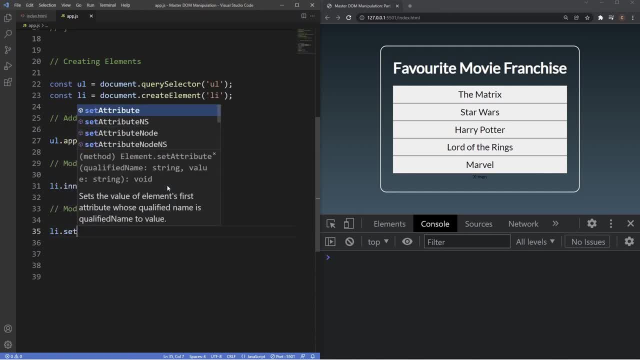 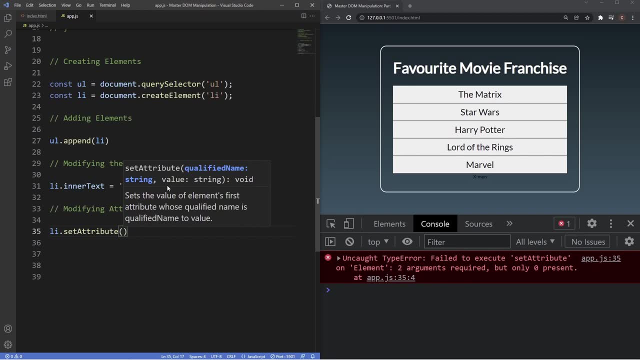 attribute method. so we'll grab our list item and we'll say set attribute and, as you probably guessed- because it's pretty self-explanatory- what it does is set an attribute to our specified element, which in this case is our list item. so for this attribute you need to include two values. the first is the. 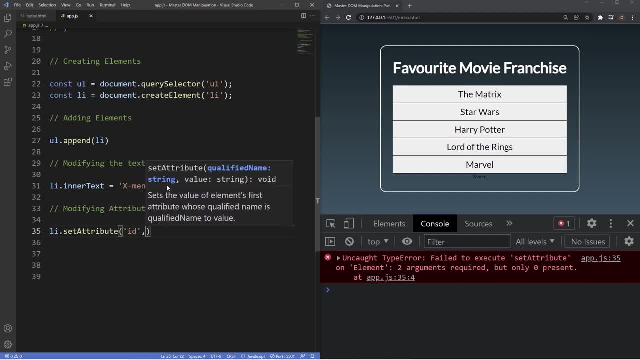 attribute you want to set, which we'll just put an id, and then the second is the name you want to give that attribute. so we'll just give this attribute, let's say, let's give it the id of main heading and, as you can see in the browser now, because we've given this list item the same, 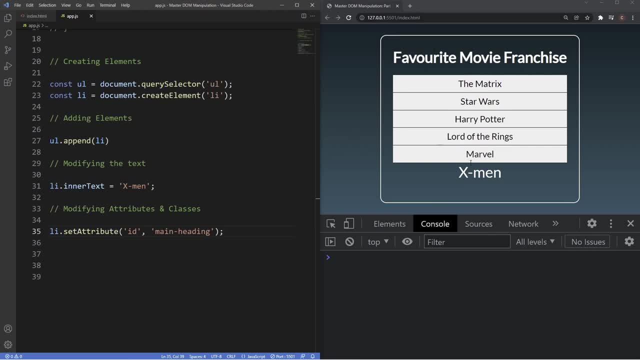 id as our main heading here, which is main heading, you can see it's got the exact same styling. so, as you can see, the set attribute method is quite powerful. now the next method i want to take a look at is how we can actually remove this attribute. so we'll go underneath here and we'll 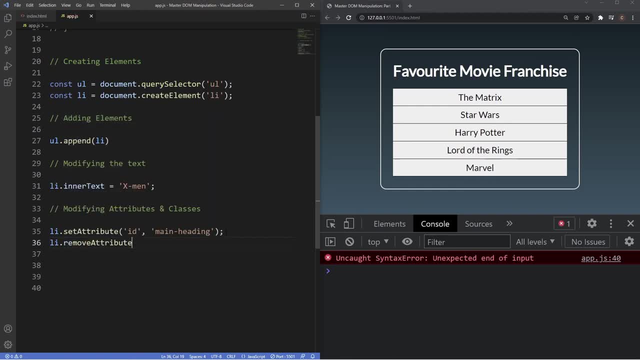 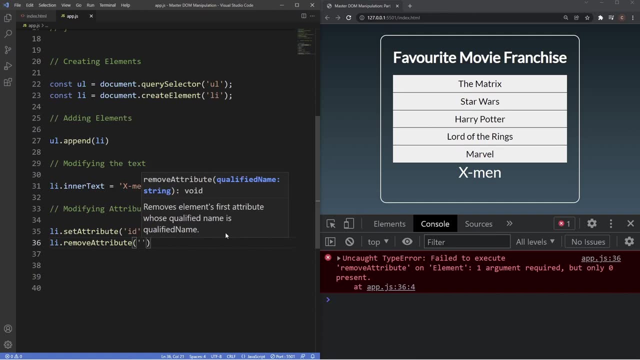 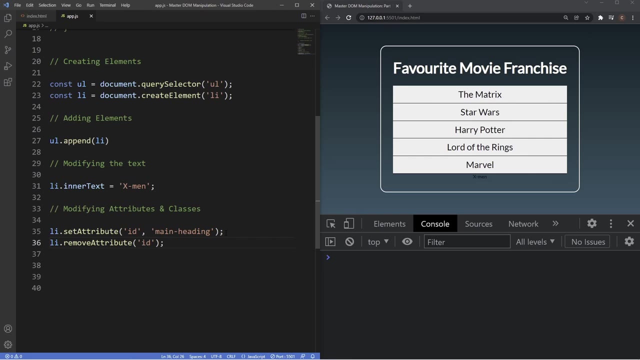 say li dot, remove attribute- again pretty self-explanatory. so let's say we want to remove the id from our list item there. all we put in here is just id: close that off. and you can see. now it's reverted back to its default styling and doesn't have that style in that the main heading does. now there's also a way. 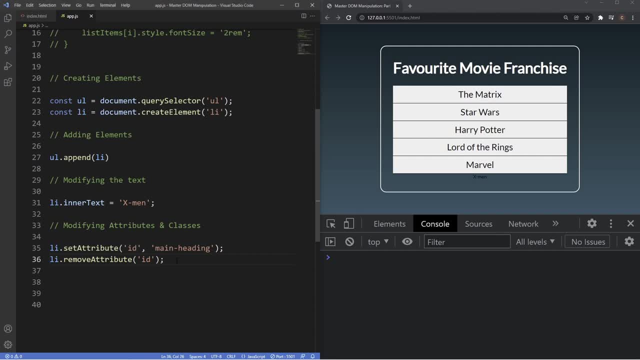 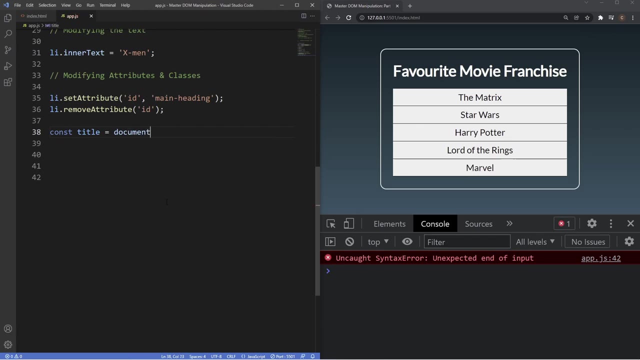 we can access attributes in javascript, so which follows a similar sort of method. so we'll say: let's say we want to get the attribute of our main heading here. what we need to do is first let's just create a variable for it, so const, and we'll say: title equals document dot query. 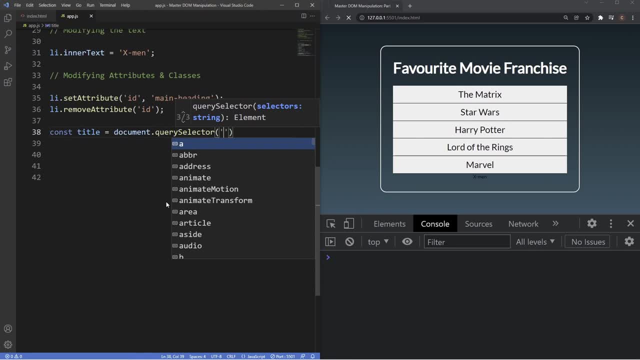 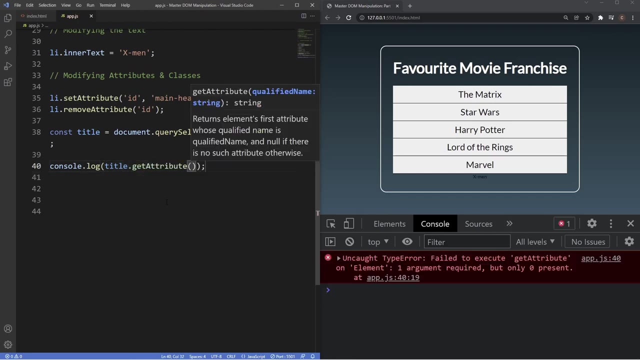 selected and then grab the main heading and then let's just log this in the console. so we'll say: title dot, get attribute. that we want is the id and, as you can see in the console now, it's given us main heading, which is the id associated with our main heading here. so that's how we can deal with attributes here. let's 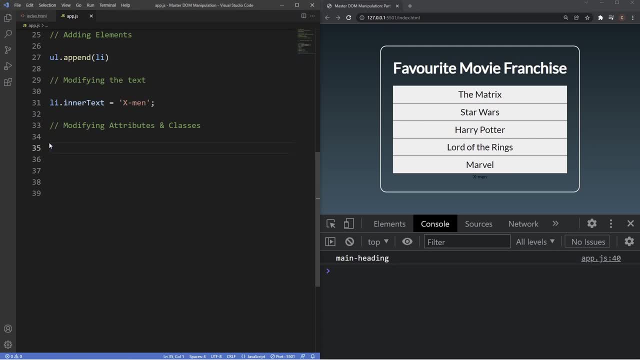 take a look at how we can deal with classes. so i'll just get rid of the this and we'll grab our list item again, and then we'll use the property of class list. now this class list property has quite a few methods we can utilize, and the first one we'll take a look at is 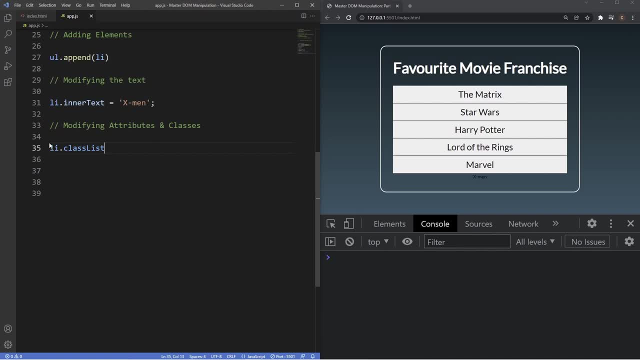 how we can use the add method, which of course will just add a class to our list item. so we'll say dot add, so let's say list items and, as you can see, when we add that class now our last list item here is the exact same styling as the other list items because again we've added the same class as. 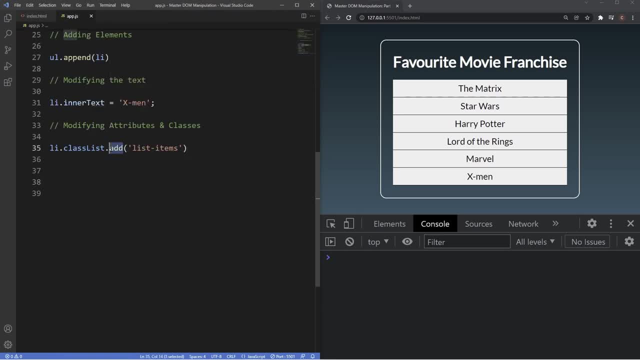 the rest of the list item. so we can just add a class to our list item, and then we'll just add a class to our list item. now what we can also do here is remove this. so we'll say remove, and again it will just revert back to its default styling, because of course we've removed that class now. 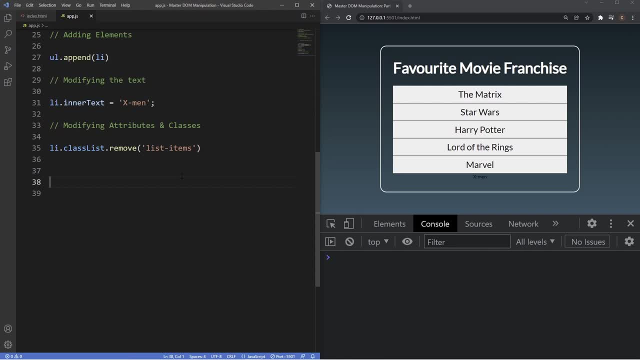 now, another thing we can find out is whether an element has that specific class. so i'm just going to log the list item into the console here, class list, and we'll use the method of contains and we're going to find out if it contains list items. and, as you can see, it's returning us false because 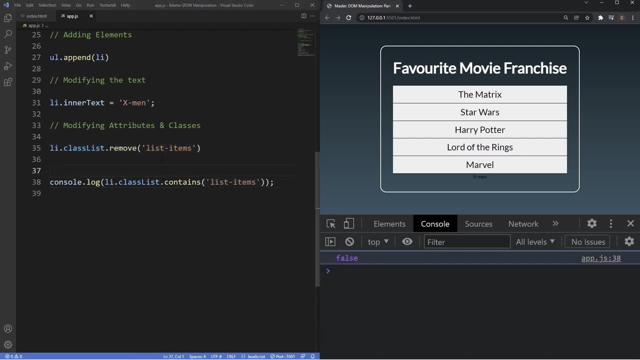 we've removed that class now up here, so it's giving us false if we change this method to add instead. you see, now it's returning us true because of course our list item here now does contain this class here. so that's how we can modify attributes and classes in the dom, of course. 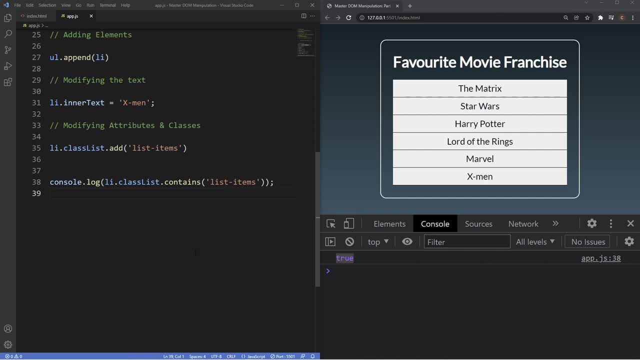 the dom has many more methods than this, but these are just some of the core methods you'll likely need to use now. there is still one method left to use, and that's how we can remove an element, and the method to remove an element- or our list item in this case, is a pretty simple method to 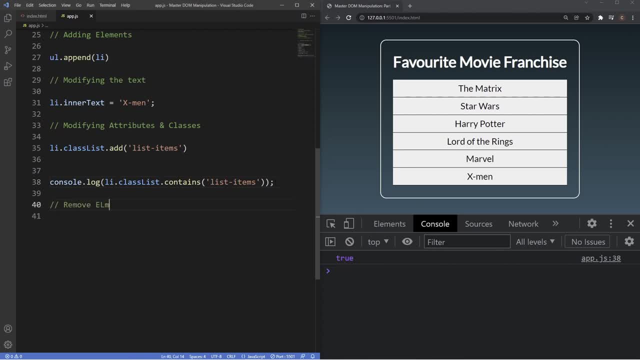 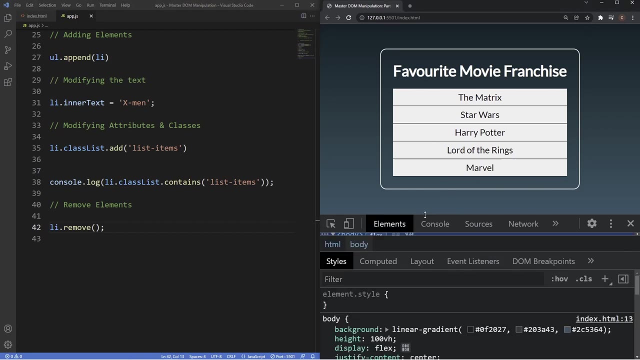 remember. we'll just put in here first: remove elements. so all we need is the remove method. so we'll say li dot, remove, and if you take a look at the console now you can see that the list item has been removed. and if we just open up all of the 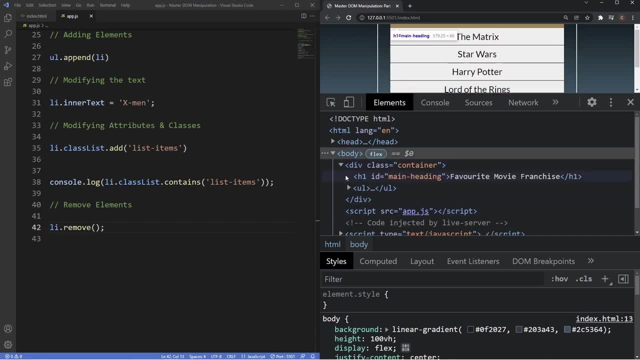 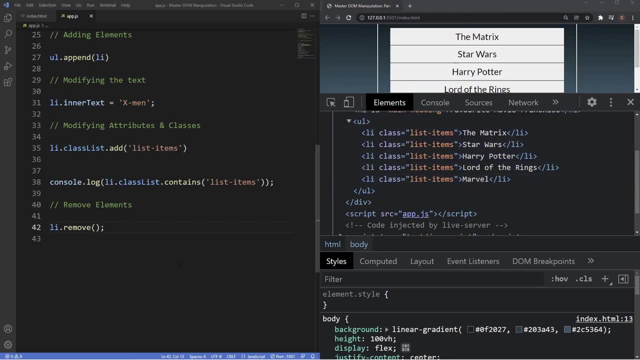 elements, and we'll open up the div here and open up our ul. you can see that list item is no longer there. so we've learned quite a bit about the dom now. we've learned how to access elements in the dom. we've also learned how to create, add, modify style and remove elements in the dom too. the next: 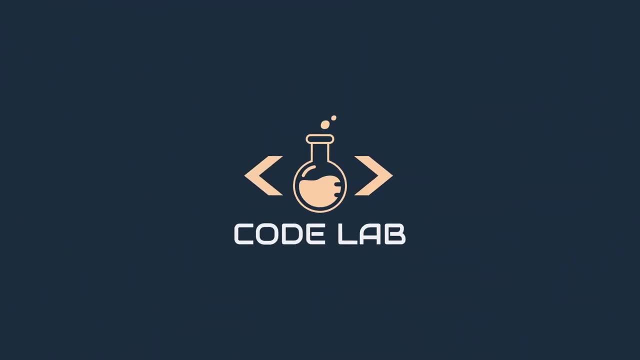 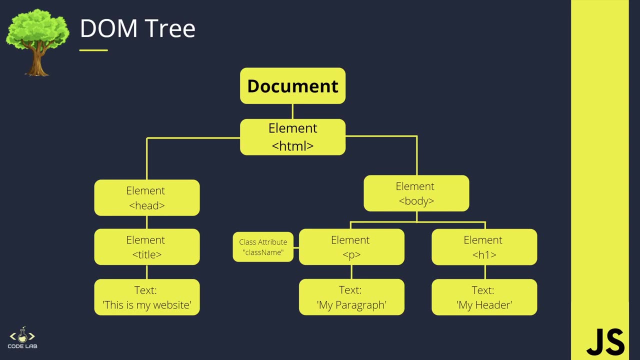 thing i want to take a look at is how we can navigate the dom. so i'm just going to bring you guys back to the slide which we looked at at the beginning of this video, where we have a really basic diagram of a dom tree and all of its nodes. now, everything in this diagram you see here is a. 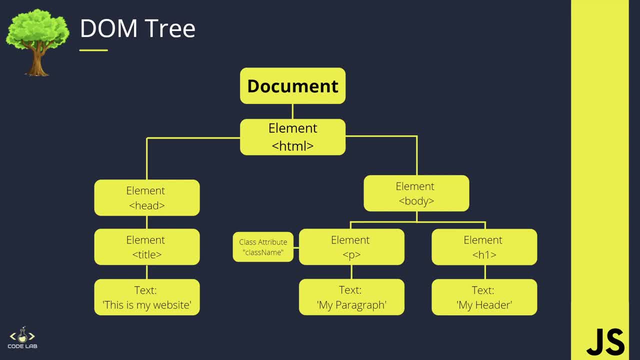 type of node, so that includes the elements, the attributes, the text content and even line breaks and comments inside the html document are considered nodes, and all these together make up the dom tree. now the dom object itself is a type of node, so we're going to take a look at that and we're going to 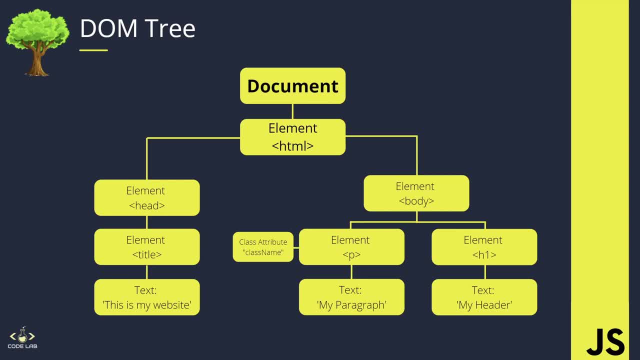 take a look at that, and we're going to take a look at that, and we're going to take a look at that- is actually a property of the window object, which is the global top level object representing the tab in the browser. the window object has access to so much information, such as the toolbar, the height. 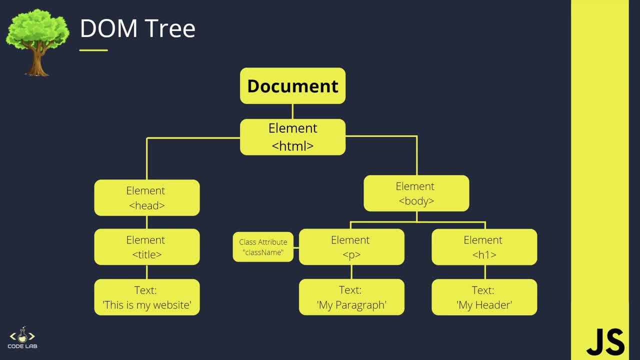 the width of the window, even things like prompts and alerts, but in this tutorial we're only interested in the document object, which is what is inside of the inner window and the stuff that we want to manipulate. now, if you also remember back to the beginning of this tutorial, most of these, 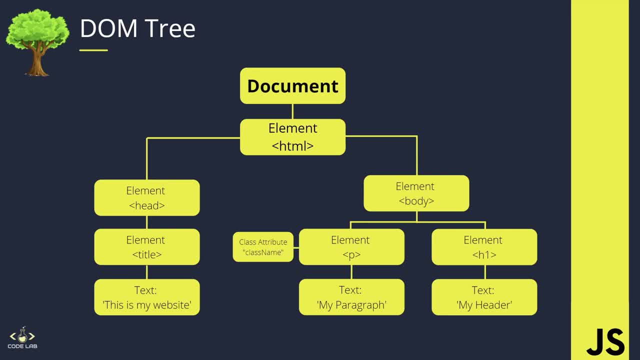 nodes in this diagram have a parent, child, sibling relationship. the topmost node, ie the document node, is the root node and the document node is the document node and the document node is the child node of the dom tree which we use to access the dom and manipulate all the content. now this: 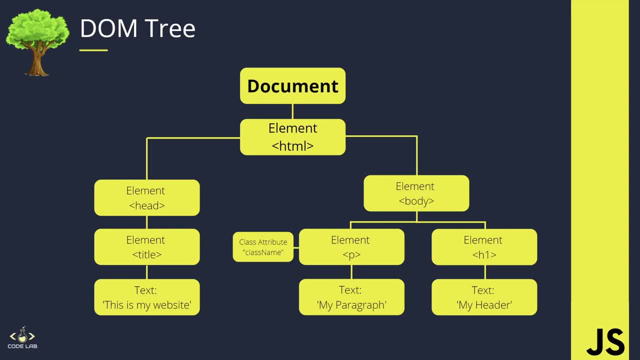 document node here has one child node, the html element. the html element is a parent node to the head and the body elements. now, the head and body elements are what you would call siblings, since they're at the same level in the dom tree. underneath the head element, you see it has a 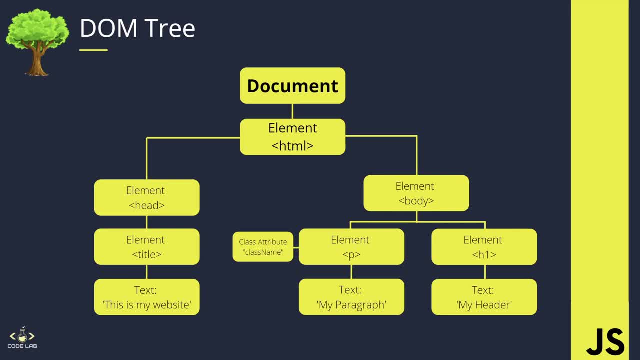 child node, which is the title element, and the text- this is my website- is a child node of the title element, and these relationships are similar over on the other side here, where the body element is parent to the paragraph and the h1. the paragraph and h1 are siblings and the text content inside. 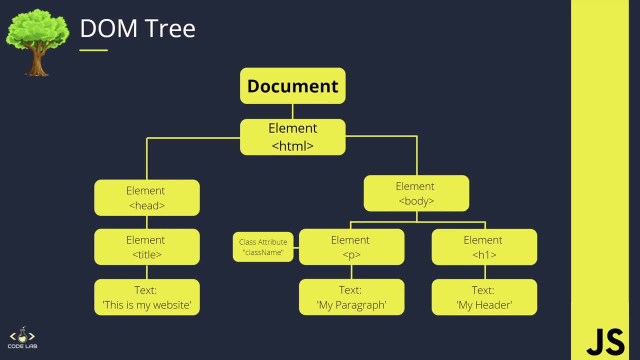 of each of these elements are child nodes, so the my link and the my header are child nodes to the h1 and the paragraph element. as you can see, here we also have a class attribute, and html attributes such as ids, styles, classes, etc. are also considered as nodes in the dom. 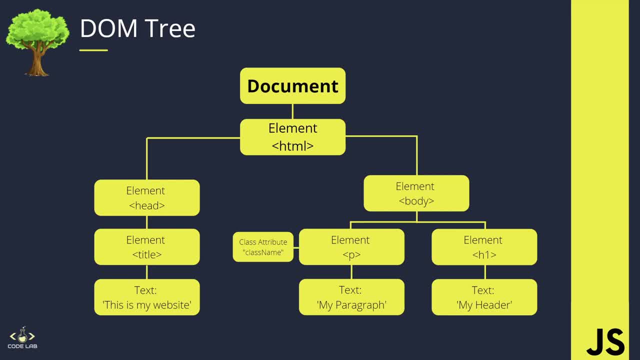 hierarchy, but they don't actually participate in the parent child relationship like other nodes do. they're accessed as properties of the element node that contains them, so they would be a property of the elements that are parent and the html element are siblings as well. more specifically, in: 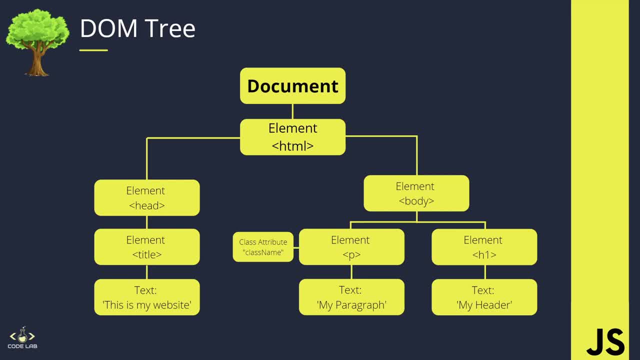 property of the paragraph tag, for example, in this diagram. Now, often there will be times where you want to move through the DOM without specifying each and every element or node beforehand. so learning how to traverse the DOM tree is essential to understanding how to work with JavaScript and HTML. So let's head back into VS Code now and look at the different ways we can. 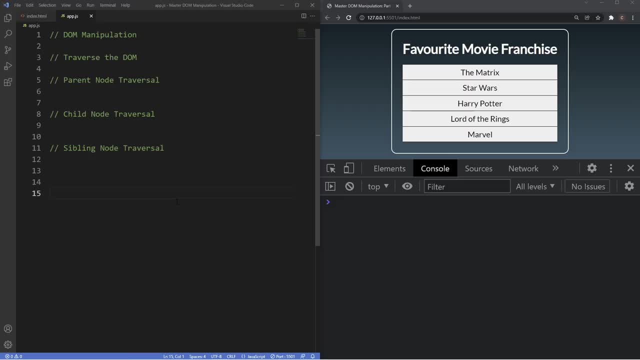 traverse the DOM, Alright, guys. so it's pretty drilled in now that we're aware that the DOM is full of different types of nodes which have parent-child-sibling relationships. and if we just head into the HTML file here just to see this in action, you can see that the HTML element 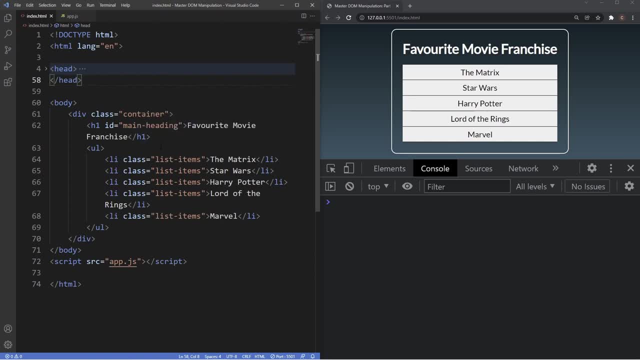 is the parent of the head and body element, and the body element is the parent to the div, but not the H1 here or the UL, since these are two levels down from the body. Now, the H1 and the UL are what you would call siblings, because they're on the same level. so what we're going to do here is use this. 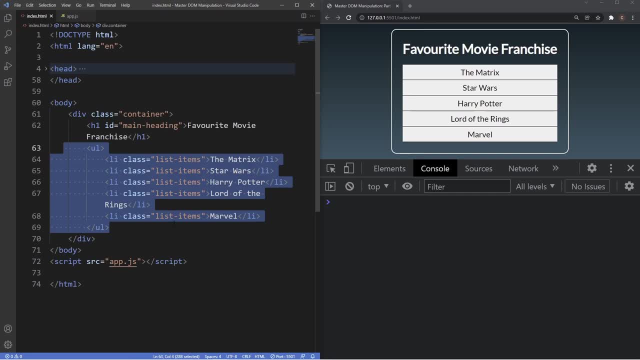 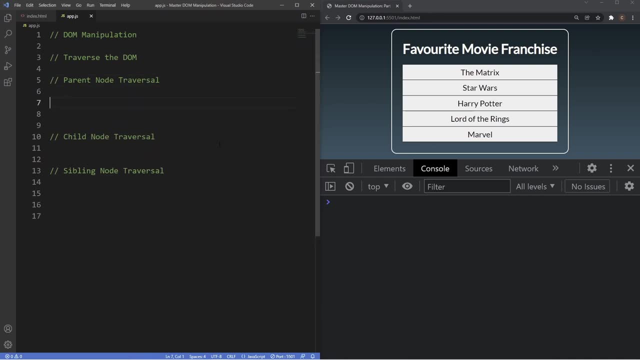 UL and traverse upwards in the DOM and find out what the parent of the UL is and also the grandparent. So we'll head back into the appjs file and go underneath parent- no traversal- and let's just first create a variable to grab that UL. so we'll say let UL equals document dot query. 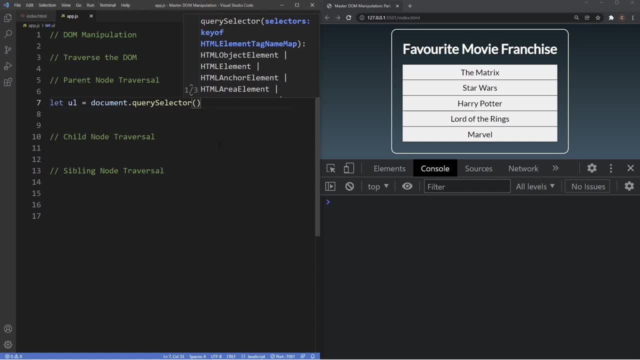 selector and then grab the UL and then just log this in the console. So we've got our UL there and you can see it hovers over it. and, as we know, nodes in the DOM are referred to as parents, children or siblings, depending on the relationship to other nodes. Now the parent of any node is: 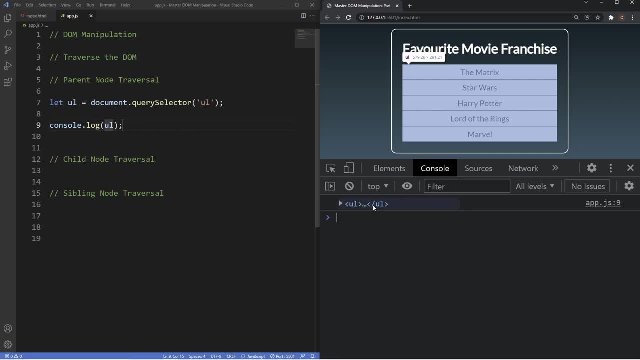 the node that is one level above it or closer to the document in the DOM hierarchy. so to find out the parent node here we have two options. so the first option is parent node, duplicate this and we also have parent element and, as you can see in the console now we're getting the div or the. 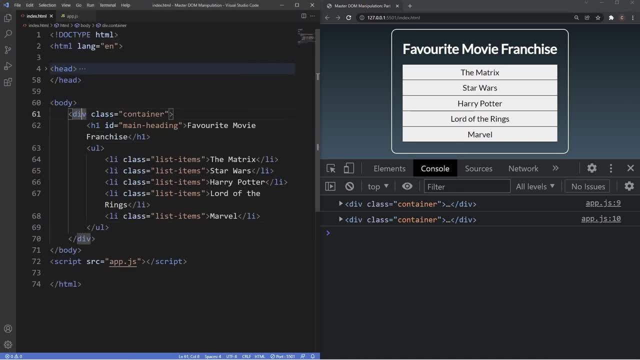 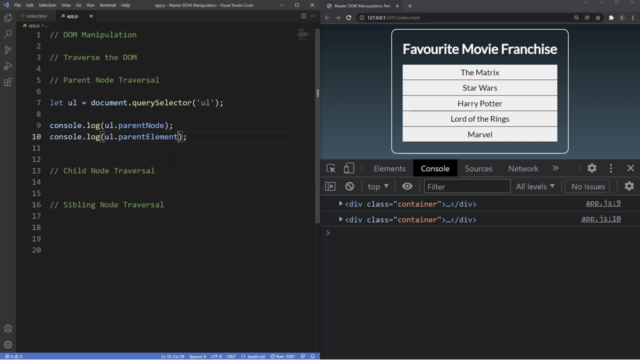 class of container because this is the parent of the UL here. Now say we wanted to actually traverse upwards again and find out the grandparent of the UL. all we need to do is double down by chaining together. so after parent node we just write parent node again and we'll do the same thing with parent. 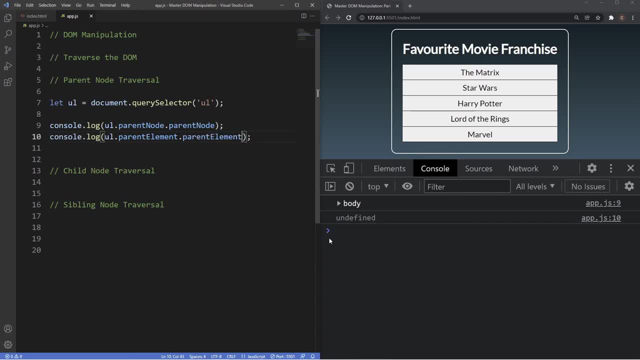 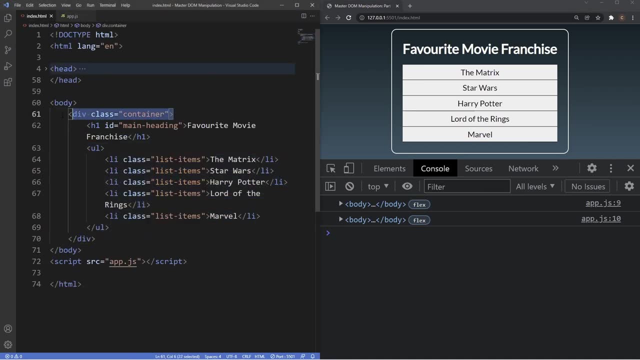 element. As you can see, now in the console we're getting the output of body because two levels up from the UL here first is a container and then the body. so, as you can see, what we've done here is managed to traverse up the DOM tree from the UL to figure out what the grandparent is. so it's. 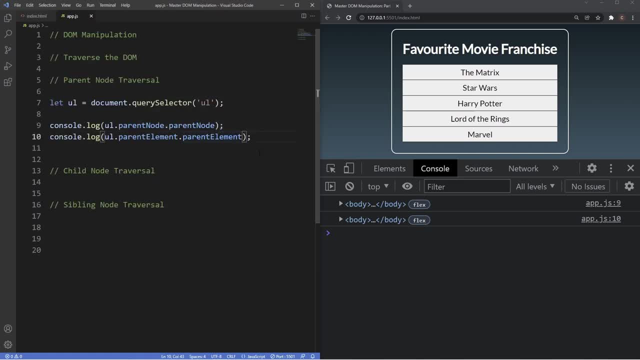 really useful to know these kind of properties. Now you may be wondering what the difference is between these two, and it will make more sense if we just do a little bit of a test on the UL. So we're going to go ahead and do that. We're going to go ahead and do a test on the UL and we're going 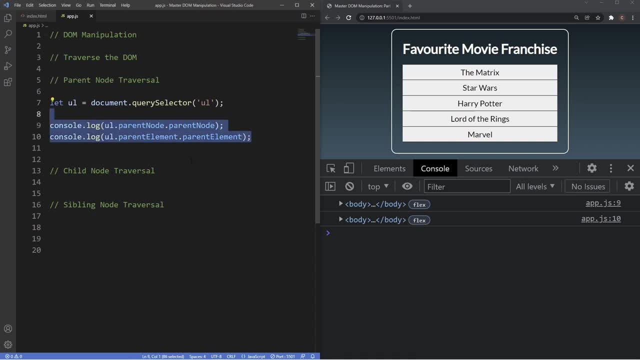 to do a test on the DOM tree and we're going to go ahead and do a test on the UL and we're going to when we take a look at how we can traverse child nodes in just a moment. but basically the clue is in the name. so you can see, here we have parent element and parent node and we know that elements 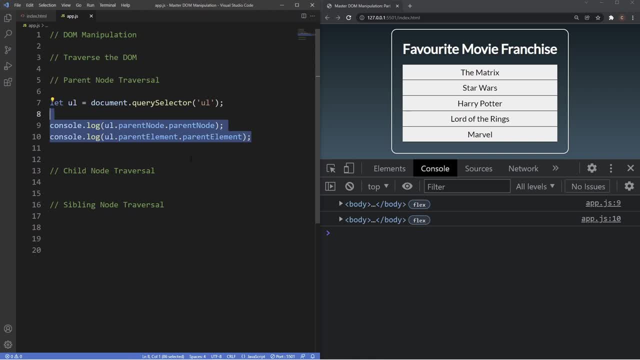 are a type of node, and this is where it can confuse people because, as we know, notes can be text, it can be a document, um comments or even line breaks. so this distinction can help grasp the difference between the two. now, that might still confuse you guys a little bit, so i'm just 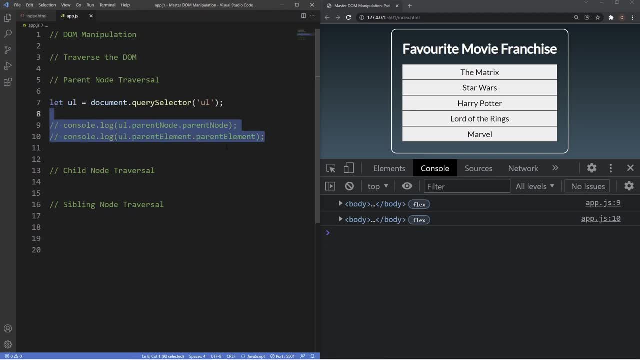 going to show you this in action. so i'm going to comment all these out and i'm just going to create a variable for our html element. so we're going to set this to document dot- document element and then i'll just log this in the console again. so we'll log in here, html, and you can see we've 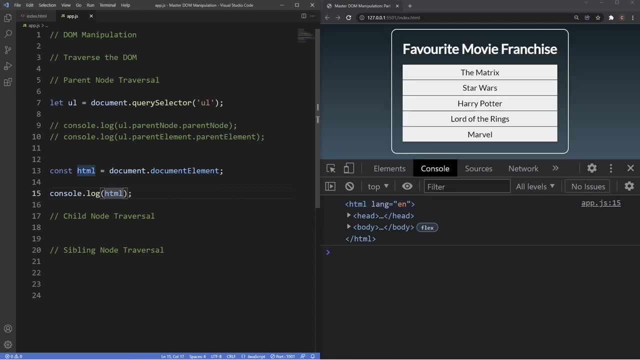 selected our html there. now i'm going to do the same thing and apply the parent node and the parent element property to this html variable. say parent node, duplicate this and we'll say parent element. and, as you can see, when we take a look at the console now, the parent element is returning us. 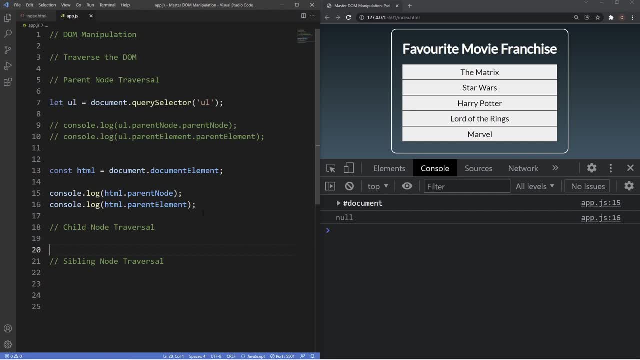 null. that's because the job of the parent element property here is to try and retrieve the parent element of the html element, ie the document node. however, the document node and an element node aren't the same type of node, hence why we're getting this null here. so the parent 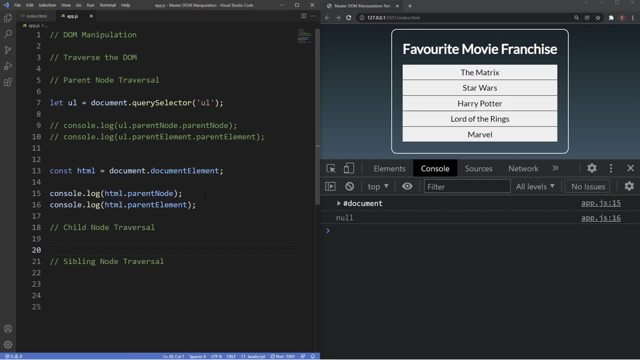 node property will try and retrieve any node regardless that type of node. so generally parent node is more commonly used when we're traversing the dom. but again, even if you use parent element you likely won't run into this problem. so that's how we can navigate upwards in the 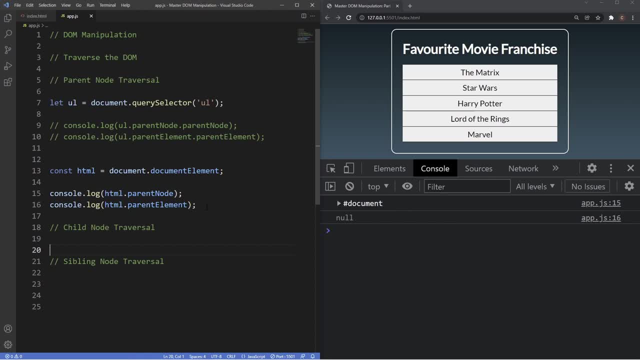 dom. so that's how we can navigate upwards in the dom. so that's how we can navigate upwards in the. let's now take a look at how we can traverse downwards in the dom by taking a look at the child node traversals in the dump tree. so for this example, we're still going to stick with the ul and 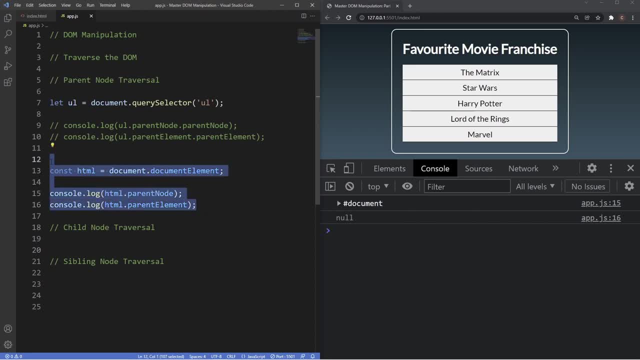 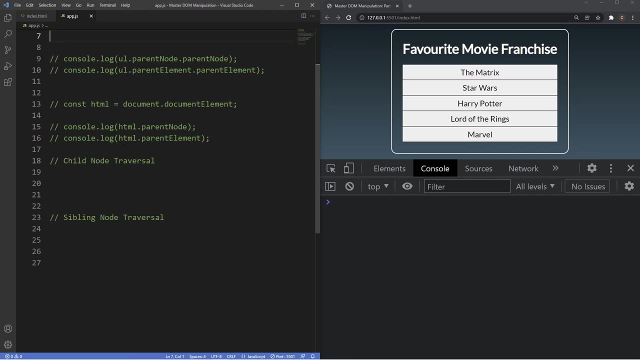 we're going to traverse downwards into the list items, so i'm just going to comment this out and then go underneath the comment. and because we're sticking with the ul here, i'm just going to put this here so we can see it and i'm just going to console login ul now, just like the property of 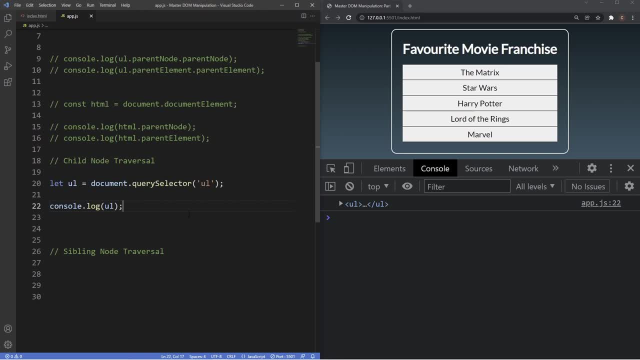 parent node and parent element. we also have child node properties and child element properties which pretty much work in the exact same way. so let's first take a look at the child nodes property and see what it gives us. so after the ul, i'm just going to type in here: child nodes you can see in the 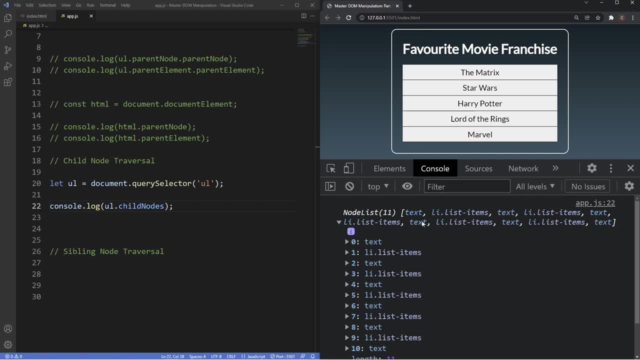 console. now it's giving us a node list and if i open this up, we get a list of every child node inside of the ul. now again, this is where the distinction between nodes and elements becomes more evident, because you might have expected this property here to give us the five list. 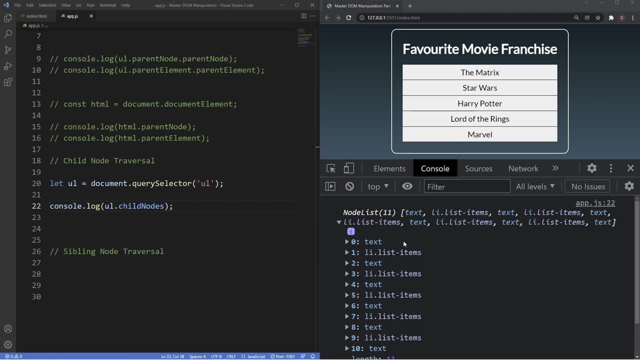 items. but, in addition to the five list items, six text nodes. this is because we actually wrote out our own html. this wasn't generated by javascript, so we're just going to go ahead and do that, and we're going to go ahead and do that, and we'll go ahead and do that, and we'll go ahead and do that. 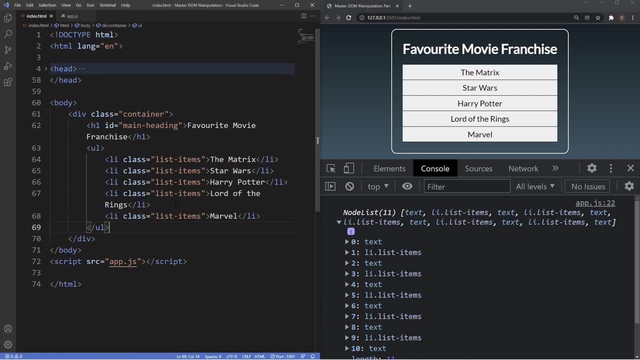 and inside of the html. here the indentation between element nodes is counted in the dom tree as text nodes. now, so just to show you guys what happens if i remove one of those indentations, so i'm just going to put this list item in the same line as the fourth one you can see now in: 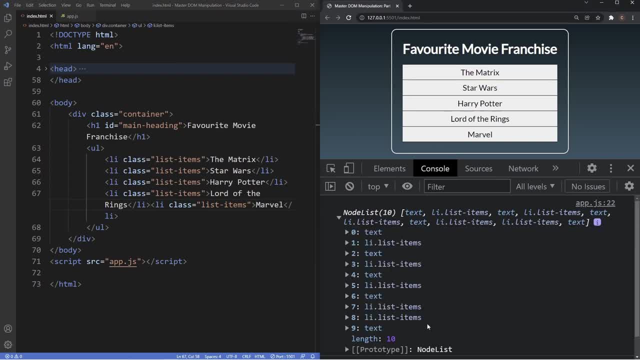 the node list it's saying 10 instead of 11 again, because indentations are counting as text nodes. so again that distinction between nodes and element nodes becomes even more evident. so what we'll do is actually just put that in another line again, so we get a node list of 11.. 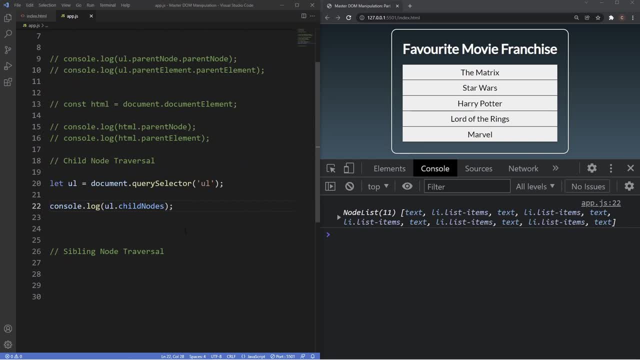 and that's going to put that in another node here, which is the first and last child. and, as you probably guessed, this just selects the first and last child node of our list here. so i'm just going to duplicate this a few more times and for this example we need to write as: 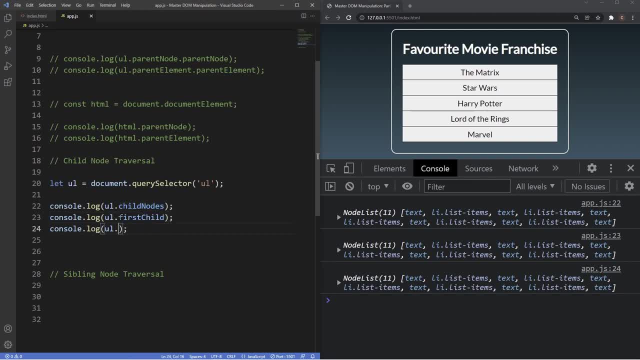 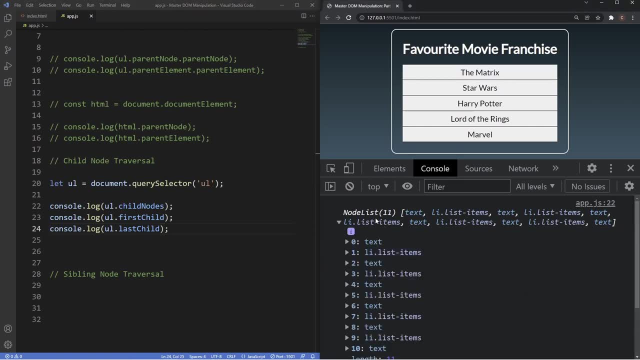 just first child and last child. and again, this is just returning as text nodes, because if we take a look at the node list here, you can see that the first index is a text node and then the last node. now, when we're using first child and last child here, which is selecting the first and last, 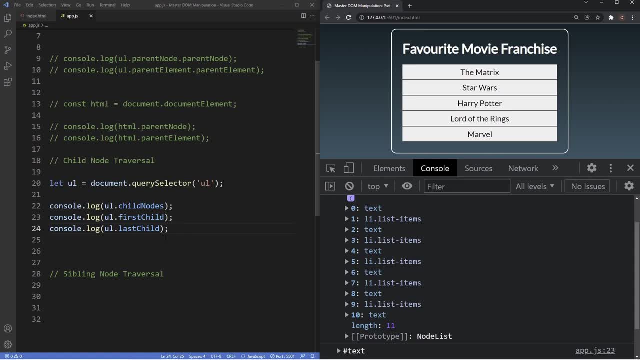 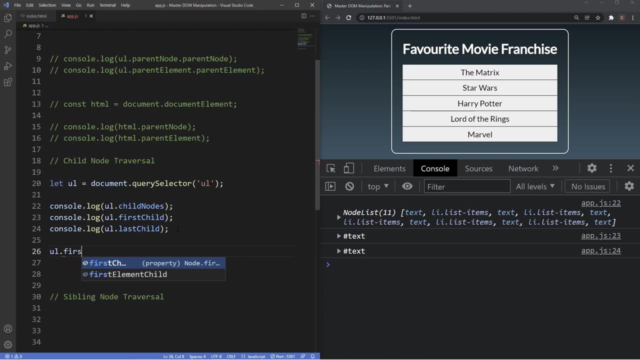 node. we need to be very mindful if we try styling element using this property. so just to show you guys what i mean: uh, if i grab the ul here and i say first child, and we're going to style first child, we'll say background color and we'll set it to, uh, let's say blue. you can see we're getting an. 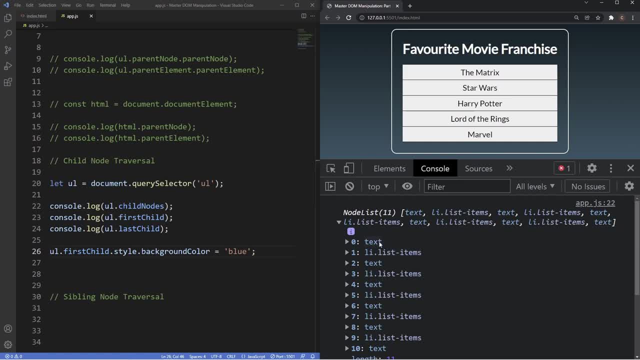 error now because the first child here is actually a text node. it's not an element now to select the node. we want to apply this style into what we can do instead of using first child here is grab the child nodes property and then take a look at the node list, and i think we wanted to apply the style. 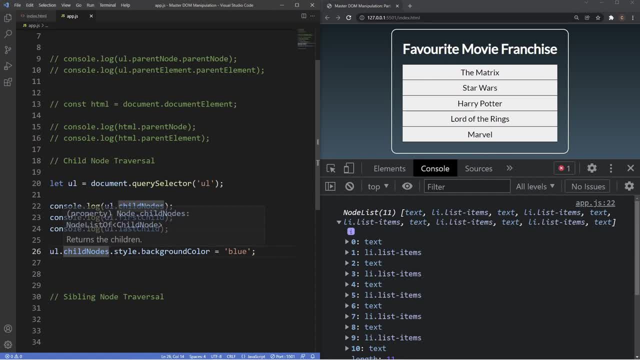 into this item, which is index that one. so we grab our square brackets, grab the first index number and if you take a look at the browser now, you can see that our first list has the background color of blue which we applied here in this styling. now again, like the parent. 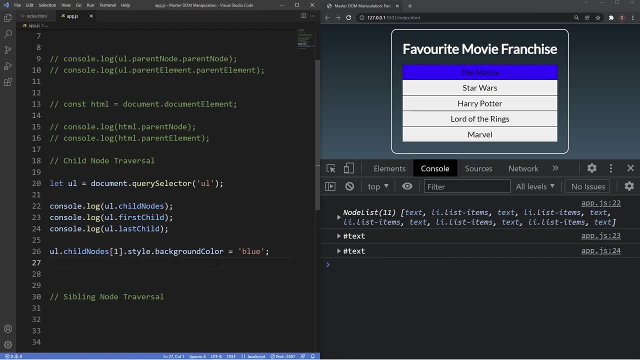 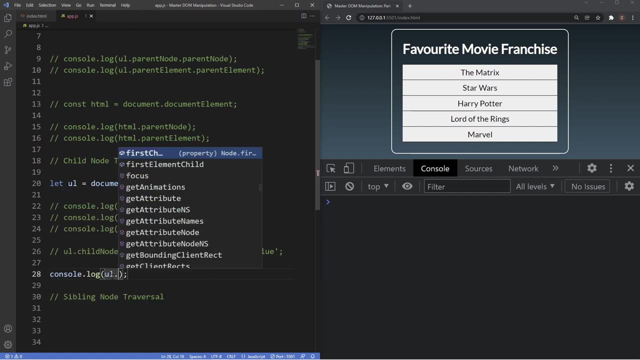 element. here. we also have the same thing for the children elements, which is only going to select the element nodes. so what we'll do is just comment all these out and we'll use that ul again and we'll log in. let's log in ul and then grab children now instead of a node list. you can see. 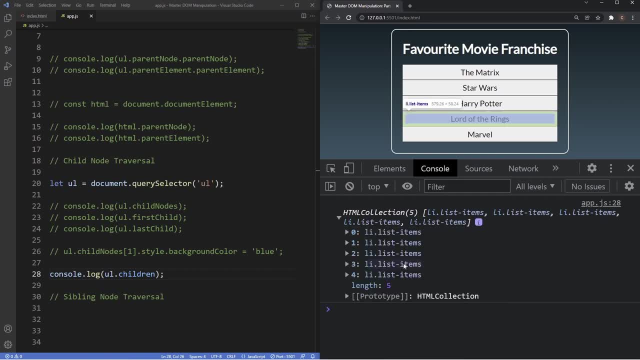 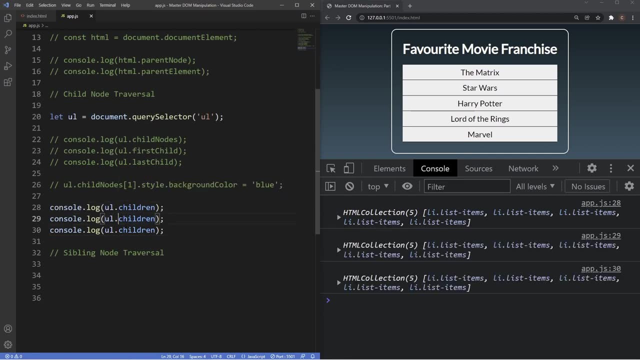 it's returning us a html collection and it says it's five, which is these five list items inside of our ul. now again, like first child and last child, we can do the exact same thing for the first child elements. so we'll say first child element. so that's how we can traverse. 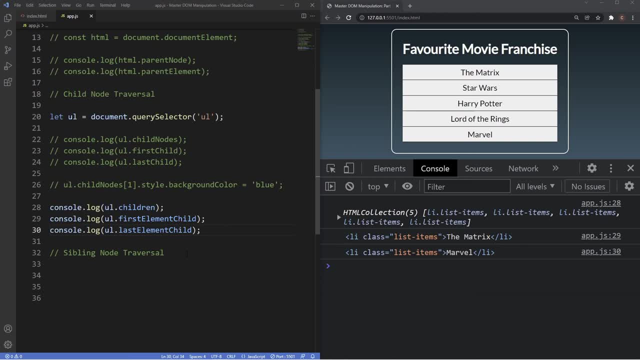 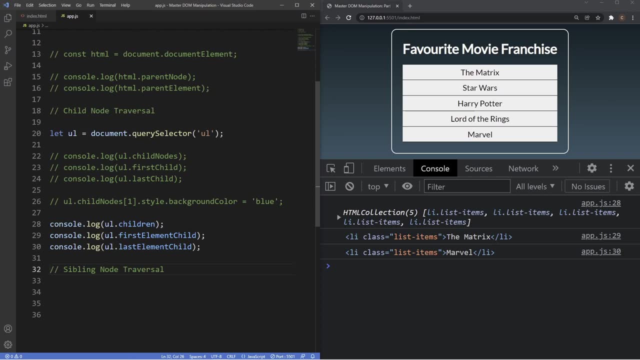 downwards into the dom using child node properties. so, lastly, now we're just going to take a sibling node traversal. so again, nodes that are siblings are nodes that are on the same tree level in the dom. so if we take a look at our html collection, we can see that we've got a child element and 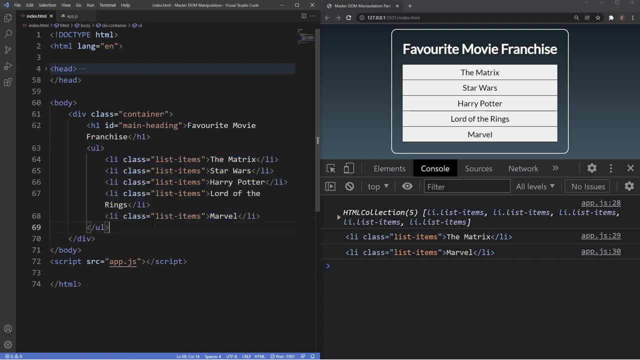 a html again. we know that the h1 and the ul are siblings to each other because they're all on the same level. now it's also important to note here that siblings don't have to be the same type of node like they are here as element nodes. if i put a text comment between the two of these, i'm just 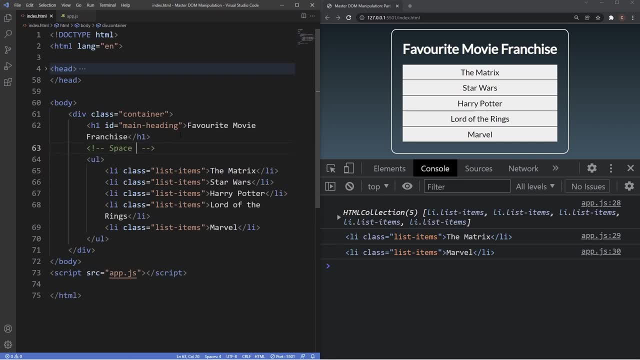 going to put in here. space between this two would classify as a sibling to the h1 and the ul, because they're all on the same level. so let's put that in a visual perspective for you guys. so i'll go back into the appjs file and i'll go underneath this comment here. 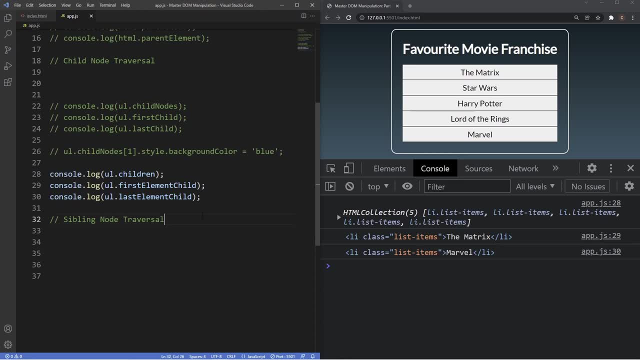 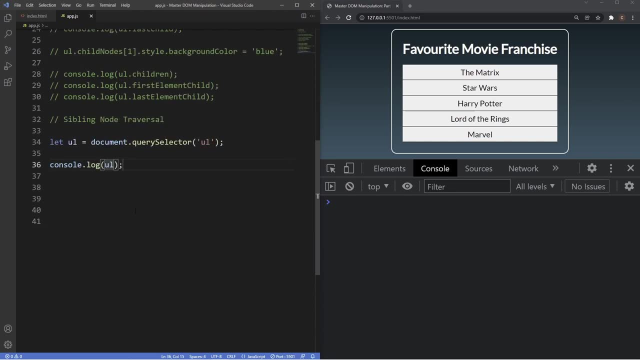 you and i'm just going to grab our ul again and comment these out and just log this into the console here, so we get our ul again. now, just like the two previous traversal properties, we have properties for nodes, which covers all the nodes, and we also have 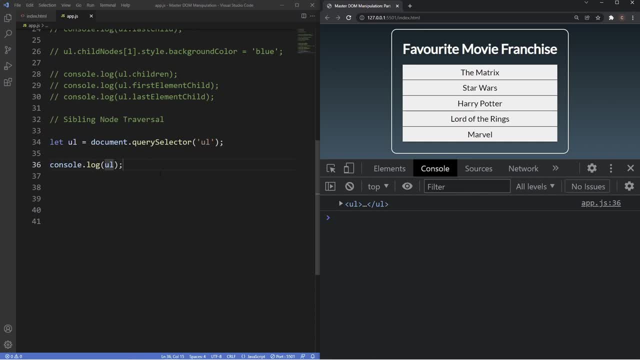 properties which just cover element nodes. so let's first take a look at how to select all types of nodes. so after the ul here we've got the previous sibling and if i duplicate this, we've also got the next sibling, and you can see in the console. now we're getting two text nodes and just to show, 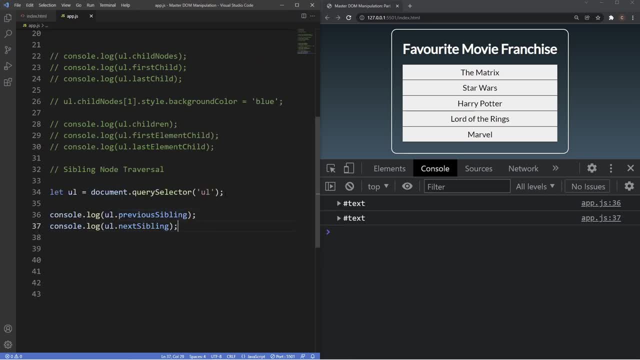 you why we're getting two text nodes. i'm just going to create another variable for our, so i'll just call this div. i'll grab the div and we want to find out all of the child nodes inside of that. oops, got div wrong. you can see. we'll open this one for this child console and then type alpha and type. 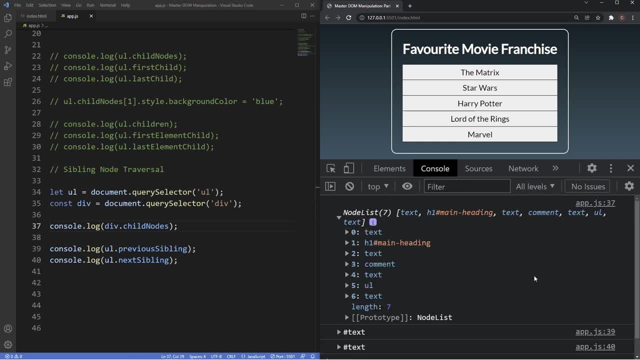 itю政府 this time, and you can see it's got urging this. so i'll just create a warning for you to leave the up now. and, as you can see, when we've used these two properties here, we've got the ul before the ul is a text node and after the ul is also a text node. so that's how these two properties here are. 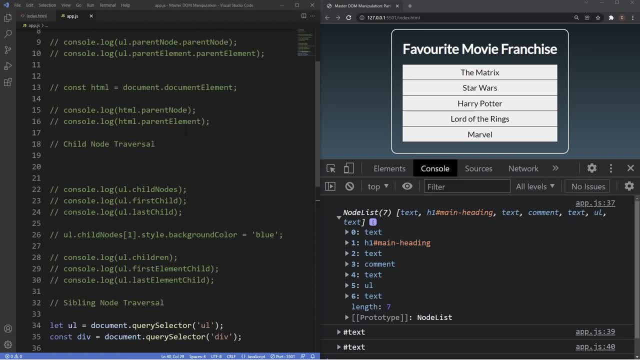 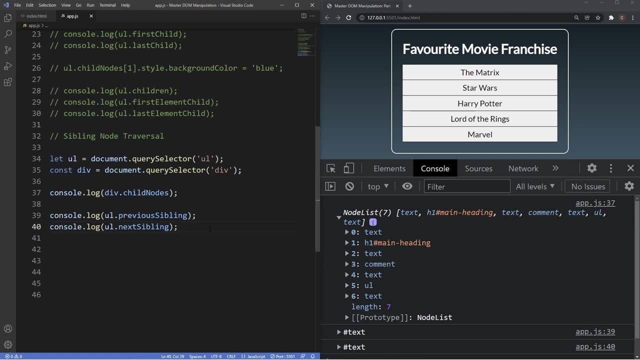 working now again, like the other properties we used beforehand, with parent element and all of these child element nodes, we have the exact same thing for sibling node traversal. so again, if you just wanted to find out the sibling element nodes, instead of using previous sibling and next sibling, 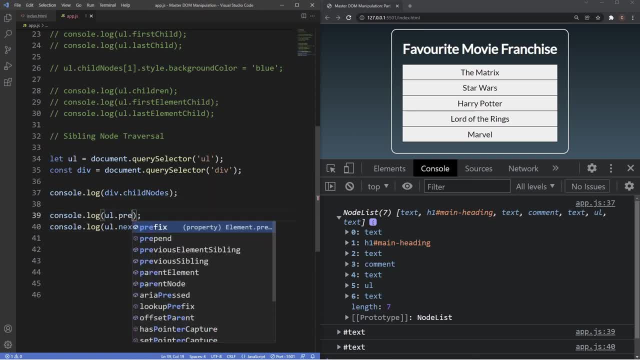 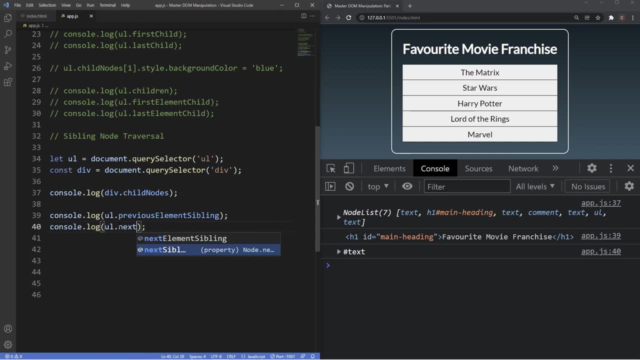 we can use the previous element sibling and we can also use next element sibling. and i'm just going to comment out this. and if you take a look at the console now, you see we're getting the h1 because this is the previous element sibling, node um. beforehand in the html. 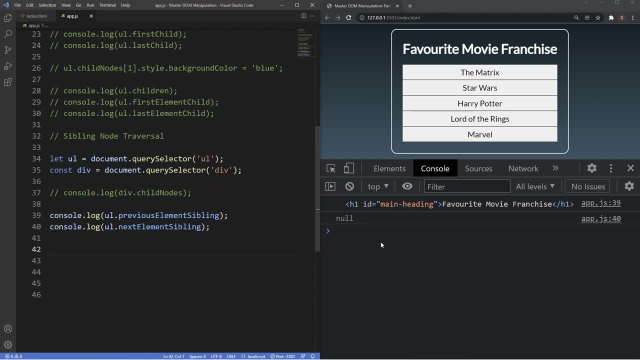 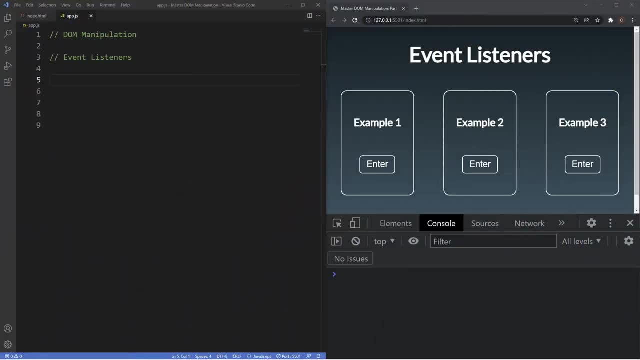 as you can see here. and then for the next element, sibling- we're getting a null because there's no element nodes after the ul. all right, guys. so we've gone through quite a bit of information now. regarding dom, we've looked at what the dom is. we've looked at how we can add elements to the dom. 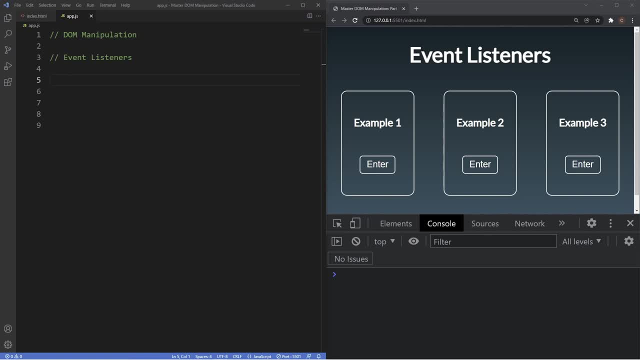 style elements in the dom, remove and modify elements in the dom, and we've just learned how we can traverse the dom. the last topic i want to cover in this tutorial is taking a look at event listeners. now, event listeners are among the most frequently used javascript structures in web. 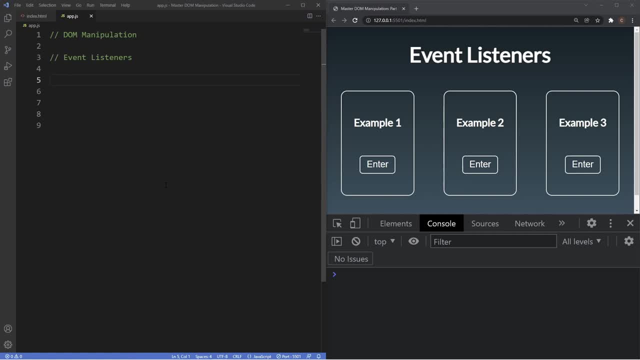 design, and what they do is basically just allows to add interactive functionality to html elements by listening to different events that take place in the dom. so here we've got a couple of events that place on the page, such as when a user presses a key, or when elements load, or when a user clicks. 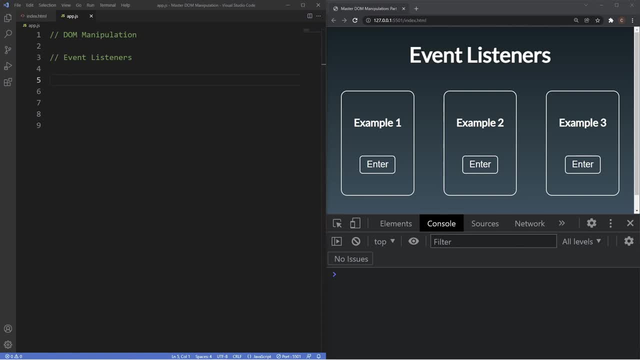 a button. now. the most common events you might listen out for are load events, touch start events, key down events, mouse over events and, of course, click events. now we'll take a look at some of these in just a moment and i will leave a link in the description if you guys want to check out all. 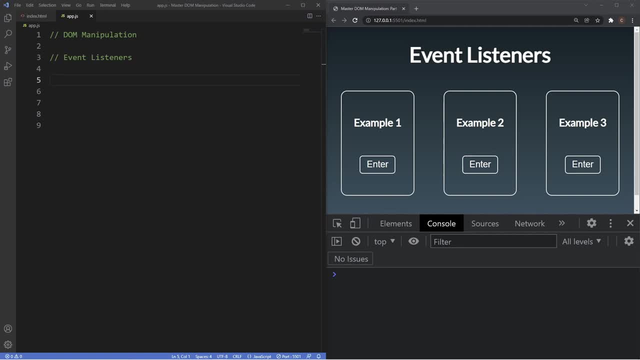 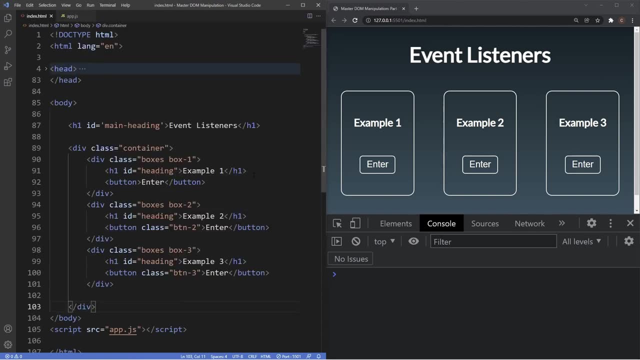 the other dumb events, but let's learn about the two most common ways we can add event listeners in our projects. now, the first way we can include an event is actually inside of our indexhtml and directly inside one of these elements. so what this event is is the global on event attribute. 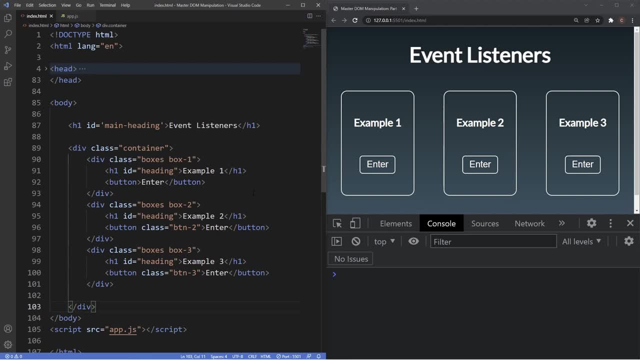 and this way of creating an event to an element works pretty much like any attribute: we insert it directly into the html element that's present on the page or the element we want to apply the event to, and then apply a one-liner script to that particular element, which in this case is going: 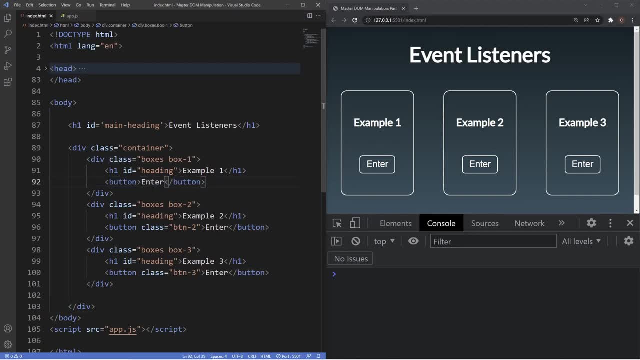 to be this button here for our first example. so we'll go inside the opening tag here like we do with any other sort of attribute, and then we include whichever event we'd like to happen. for this example, we're going to use an on click event, so 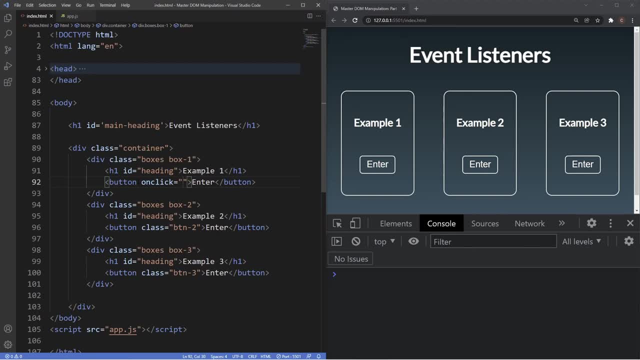 say on click. now what i want to fire off when we click on this button is just to show us an alert box that has the content of i love javascript. so we'll put in here alert and then we'll put the content of i love java script, and that's all we need to write for this. 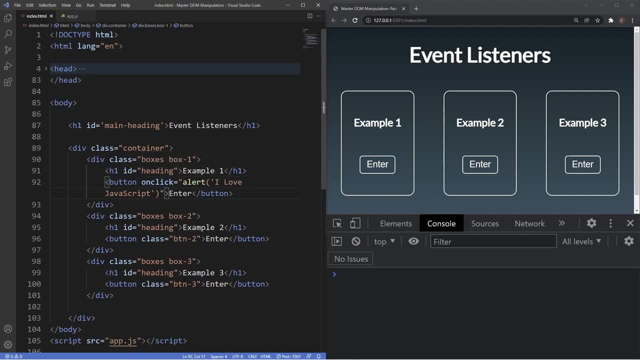 attribute. so the syntax for this, as you can see, is pretty simple. we've included the on click event attribute, so when we click on this specific button in the browser now, the event will fire off and the alert function will be executed, which will have the text of: i love javascript inside of it. 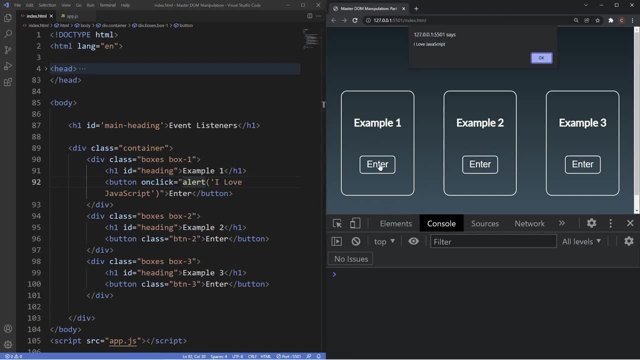 so we'll head into the browser now and i'm going to click on this button here and, as you can see, when i click on the button, the alert box pops up and it's got the content of i love javascript, which we wrote inside of this attribute here. so that's the first way we 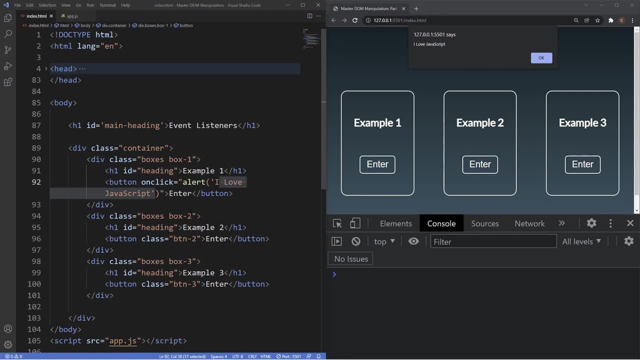 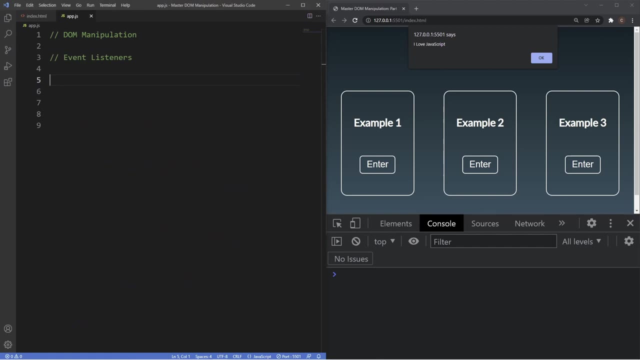 could include an event in our projects which is just direct into the html on the element we all apply the event to. so pretty simple and probably the most direct method of including an event listener inside of our projects. now the next method to create an event listener: the javascript add event listener method. so to create that we'll head back inside our appjs file. 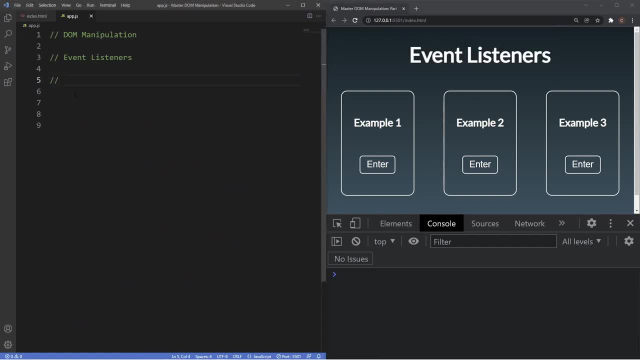 and the way this method works is first include a element that we want to apply the event listener to, so we'll just put in here element and then we use the add event listener method and then inside of here we include the type of event. in this example we'll use another click event and then 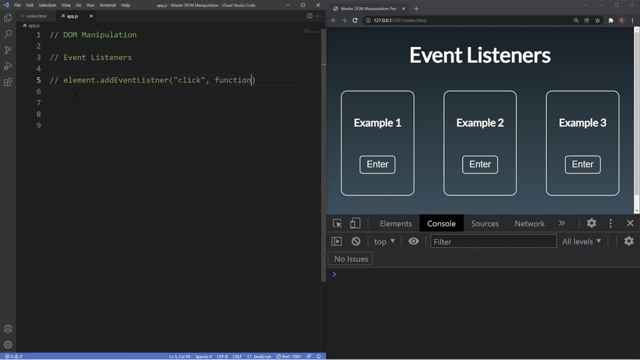 after this, the second parameter is the function we want to fire off, and then we also have an option here for a third parameter, which will take in a boolean data type. so, true or false- and this is in relation to bubbling and capturing, which we will speak about in a moment. 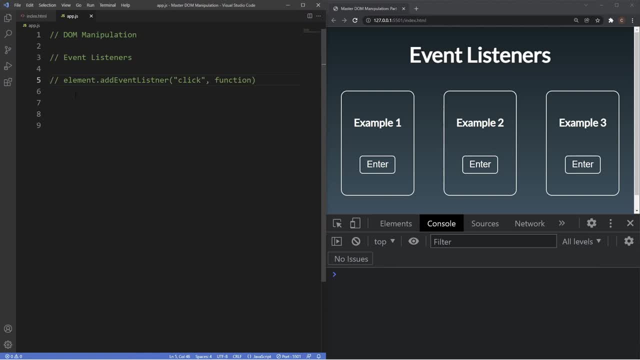 but we're not going to include that at the moment because by default it's already false. so it's not too important yet, so we'll just close it off. so that's essentially the syntax of adding an event listener using the add event listener method. so for this example we're going to use 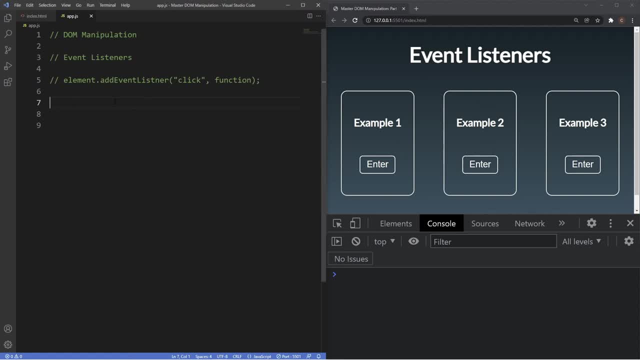 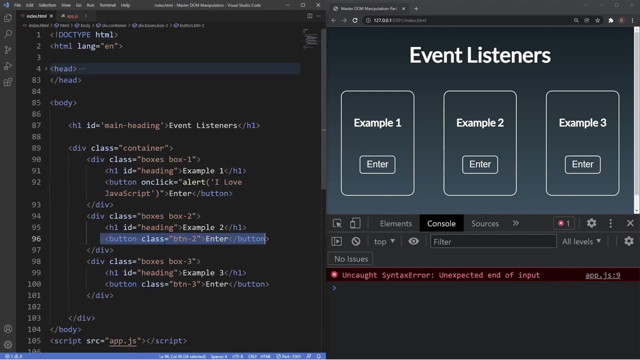 the example 2 button here and again we're going to create another alert box, um. so the first thing we want to do is create a variable for us to reference from. so we'll call it button 2, and the button 2 in the html here you can see, has a class of btn. so we're going. 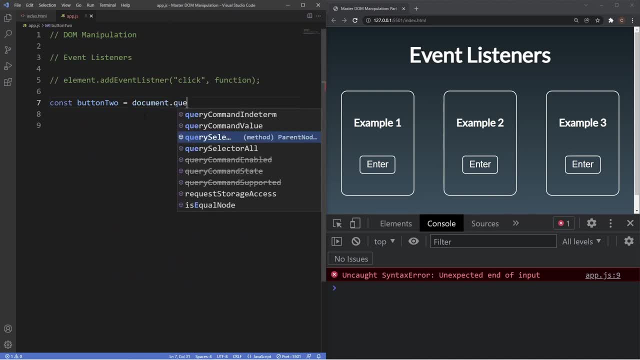 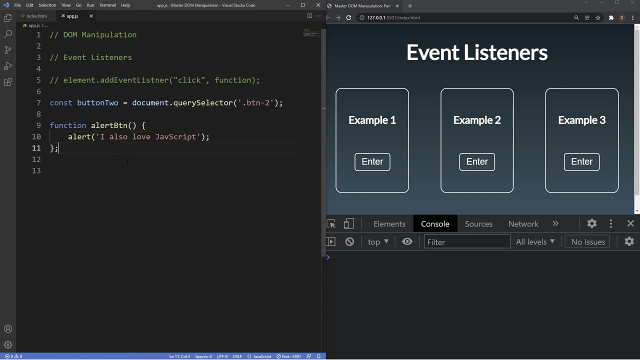 to retrieve that. so document dot query selector, and then grab the btn 2 and then first we want to create a callback function. so the function we'll call this, uh, alert btn, and inside of here we'll just put another alert box and then type in: here i also love java script- and then what we need to do now is include our 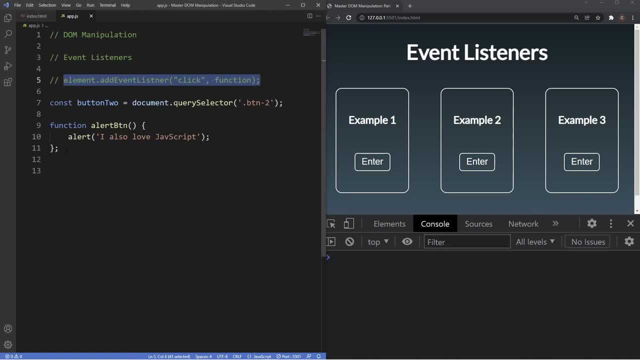 event listener. so we're just going to copy the syntax, paste it in here. the element is that button too. so we've got our out of it listening method there and then function is going to be that alert btn and we've got a little answer. oh, we've got the e in listener. 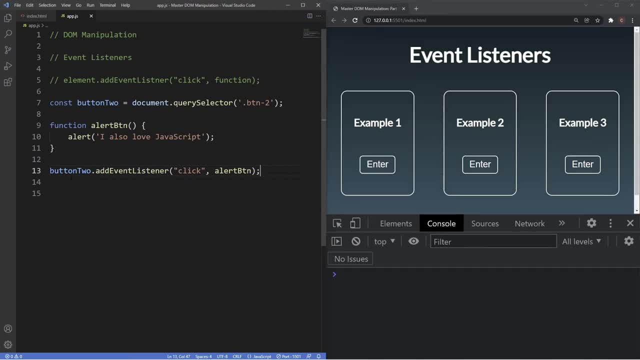 so what we've done now is included a click event on the button too, which is this button here. so when we click on this, this alert box should fire off and should appear at the top of the screen with the content again of: i also love javascript, so let's test this out and as you can see now, 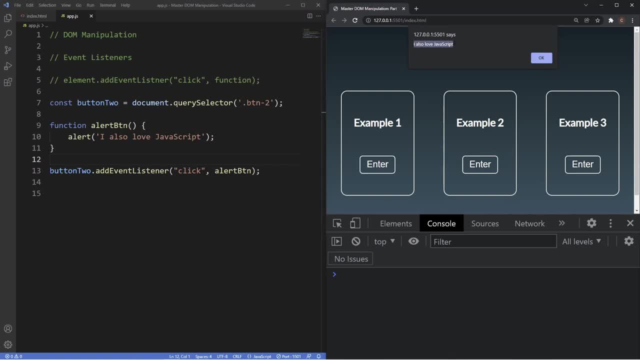 this event is working and we're getting our alert box, which has the content of: i also love javascript, so that's how we can use the add event listener method here. so let's take a look at a another example, for example three. so instead of a click event, we'll look at a mouse over event. 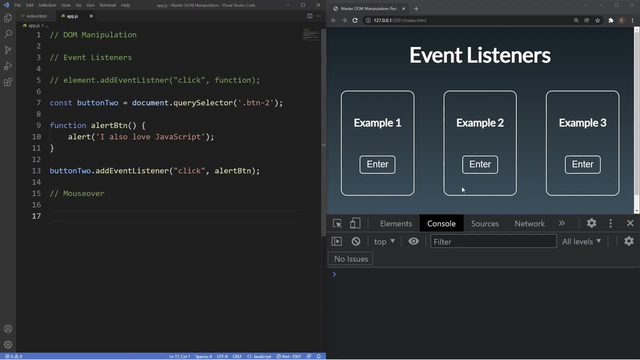 so say, mouse over here. so for this example, instead of clicking on a button here when i move the mouse over, i want the background of this whole box to change. so to do that, let's first grab- i think it's box three, so we'll create a variable for it and we'll call this variable new background color. 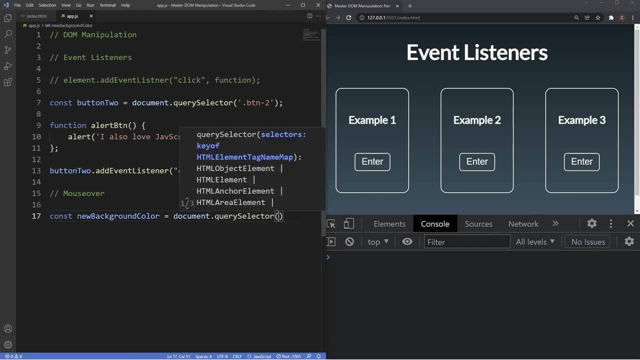 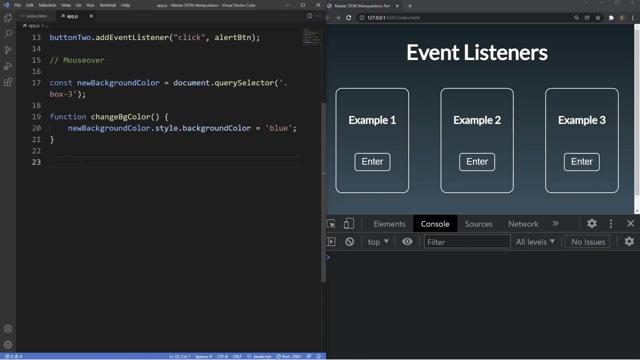 grab the box so documentquery selector, and it's box three, and then we'll first create the function. so we'll say function: change bg color. so we'll grab that variable now new background color, style, dot background color, and let's set it to the color of blue, and then we'll now include that mouse over event. 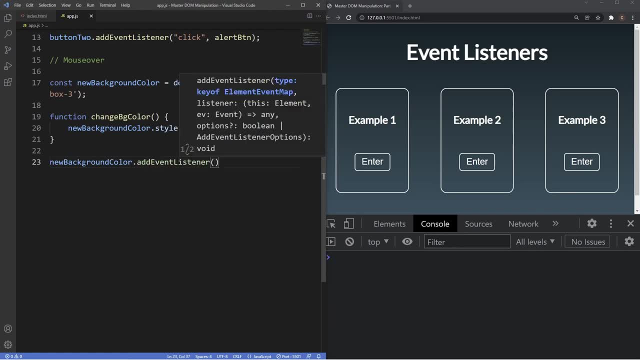 so we'll grab the variable add event listener method and we'll say: mouse over and then the function which is change bg color. so if i head over to example three, if i now move the mouse over the box here, it should change its background color to blue and, as you can see, that's working as it. 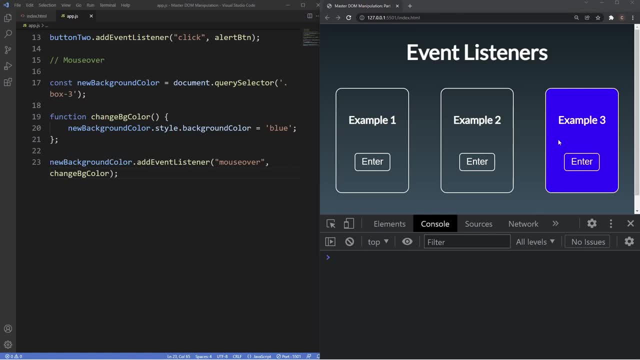 should manage to change the style of our third box using the mouse over event and the event listener method. now, generally, people do tend to use the add event listener method more than the html on event method, typically because you can apply as many event listeners to an element. 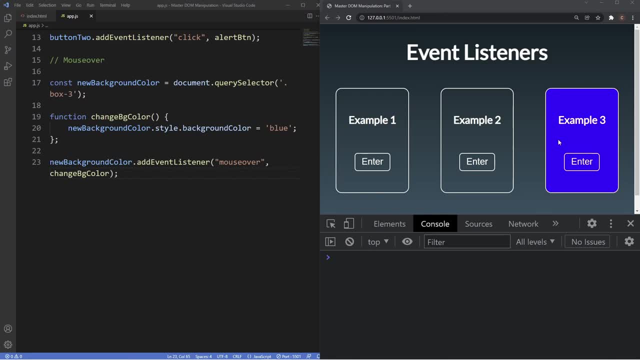 through the add event listener method, whereas with the html on event method you can only apply it once. so if you had one event already on the html element and then you try to plan another one, that new one would override the old one. but again, if you only want to apply one event, 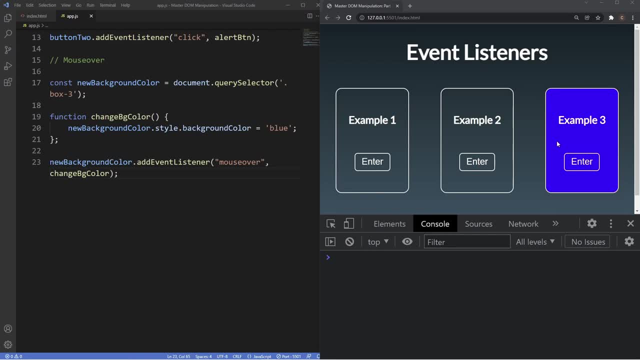 the on event method works perfectly fine. so these were some really basic example, guys, of how we can implement event listeners. we'll now take things a little step further by creating a reveal hide event, where we click a button to display some text which is originally hidden. all right, guys. so the really cool thing about event listeners is that we can combine them with. 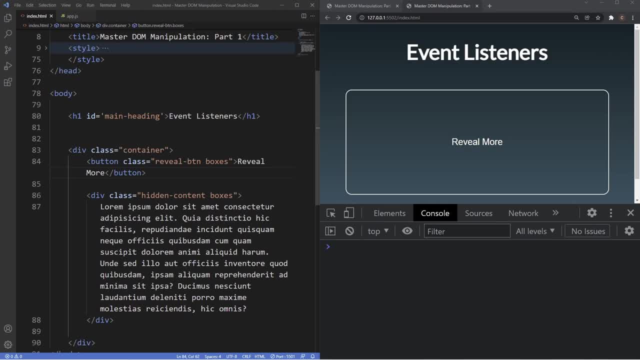 css and other javascript tools to create interactive and fun constructs, which, for this part of the tutorial, is our simple example here, where we have a button and then when i click on this button you can see it reveals more text, and if i click on the button again it hides the text. 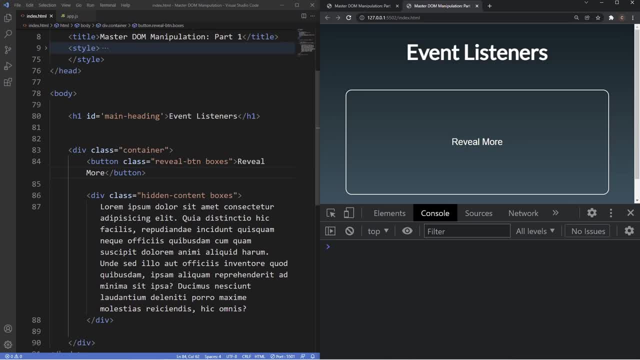 now, the html for this example is really simple. so we've got a div here with a class of container. inside of that div we've got a button element which has the class of reveal- btn, and a class of boxes which is just a general class. underneath that we have a div with a class of hidden content. 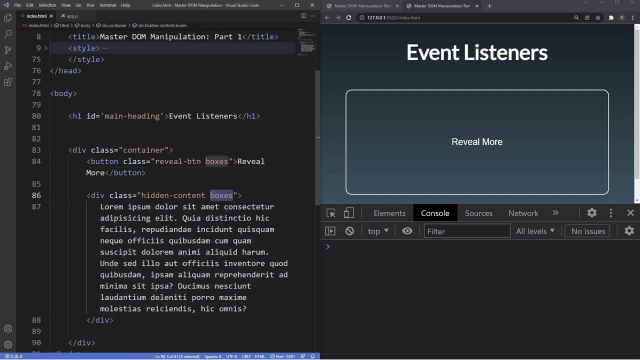 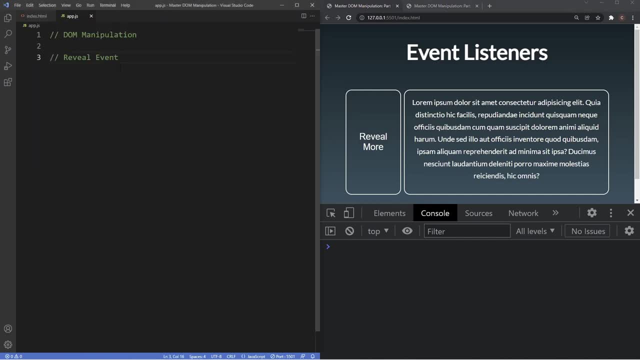 which has all of our dummy text inside of it. this also has a class of boxes, and this is what it currently looks like right now in our live content. so we're going to go ahead and create a class of live server. now, the first thing i want to do here is go in appjs file and create two constants. so 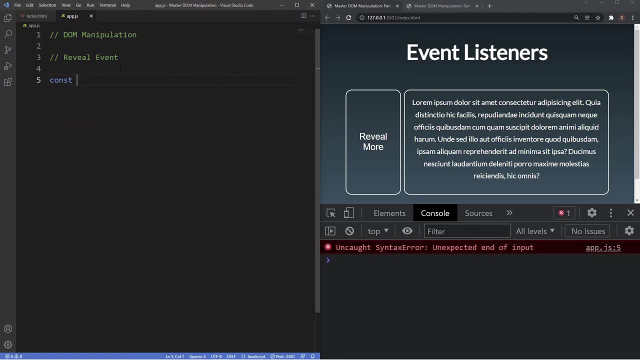 we grab those two elements. so the first one is going to be for our button. we'll just call this reveal btn and then we'll say document dot, query selector, and we'll grab that element which has a class of reveal btn. and then we want to create another. 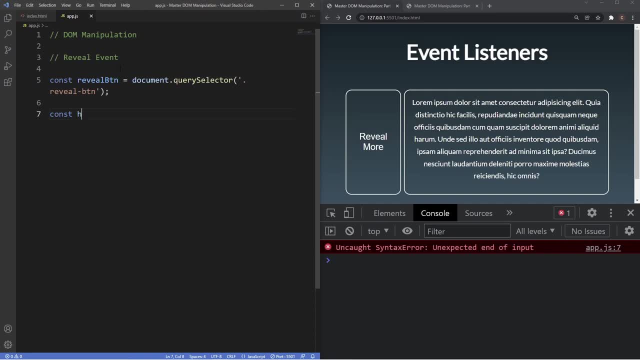 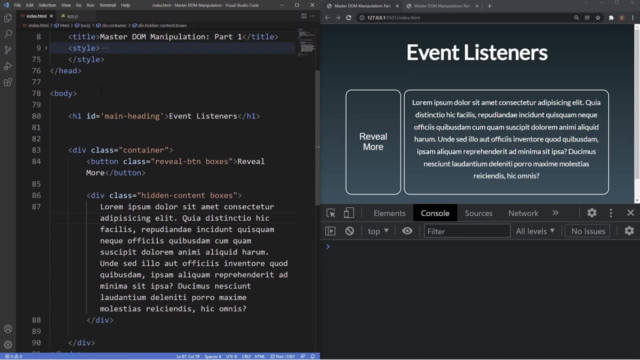 constant for our hidden section. so we'll call this- uh, let's call this- hidden content, and then document dot query selector and then grab the class of hidden content which i think. yeah, so we've got our two constants there. the next thing i want to do now: 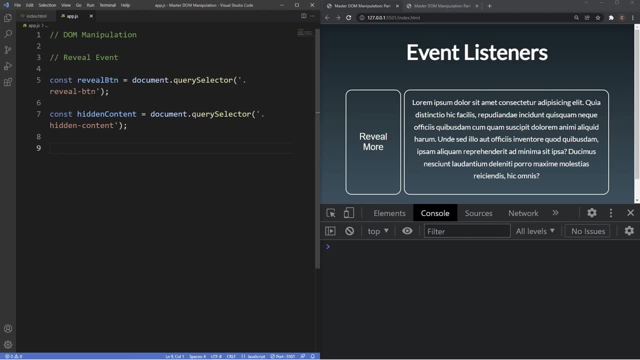 is create a callback function which will check if our hidden content here has the class of reveal btn. now i will explain this in more depth, but for now let's just create that function. so we're going to create that function. we'll call this function reveal content. 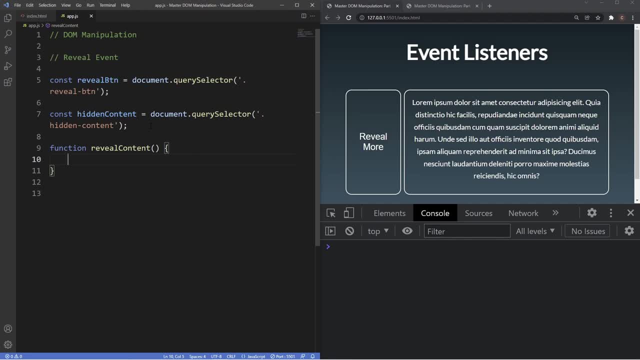 and then inside the curly braces. here we want to use an if else statement, so we'll use the if statement first. inside the brackets is our condition. so we'll say: if our hidden content grab the class list property contains class of reveal btn. so there's our condition. the code that 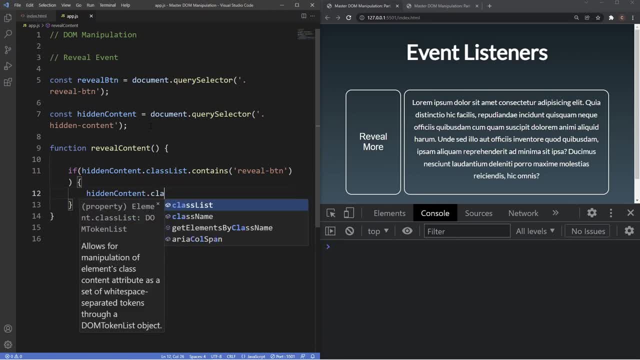 we want to execute. if this condition is true, grab the hidden content, grab the class list property and we want to actually remove this class if it does contain the class. so remove the class of reveal btn again. this will make more sense in just a moment, but we're just. 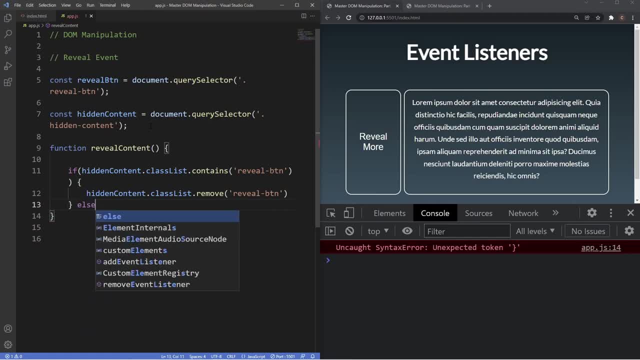 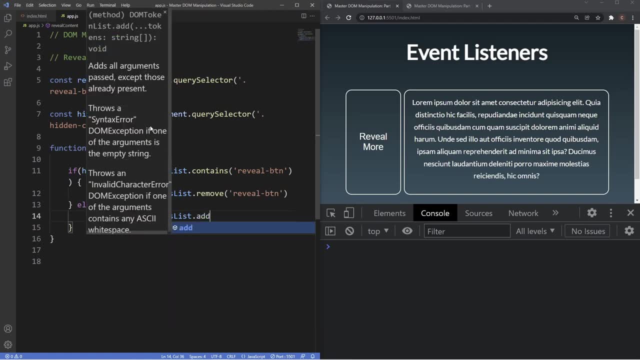 going to write this out for now. else, if it doesn't contain that class of reveal btn, then we want to grab the hidden content classes property. then we want to add that class of reveal btn now. the next thing i want to do now is include our event list now, so we want to apply the event listener on our 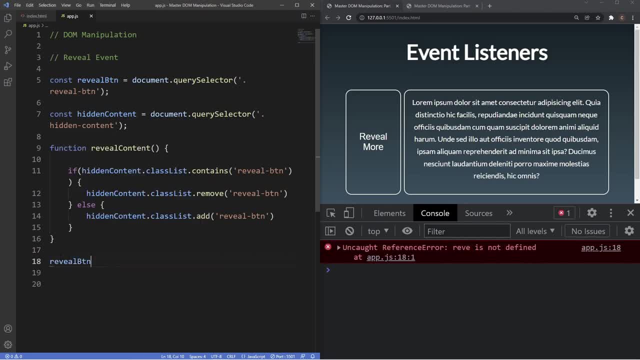 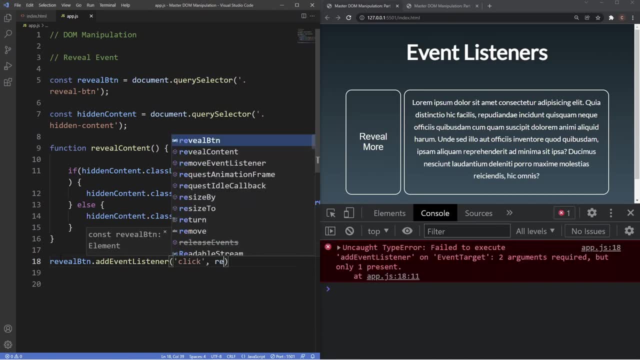 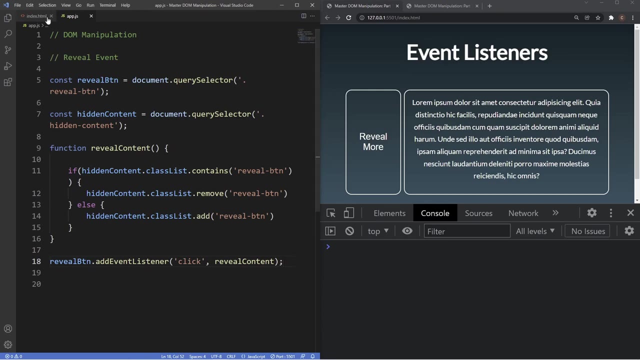 button here. so say: reveal btn. reveal btn, add event, listener, and we want to look out for a click event, and then the function we want to run off is the reveal content function we just created. and the last thing we'll do now is visually hide our div here which has the dummy text. so we'll do that inside our style sheet. so 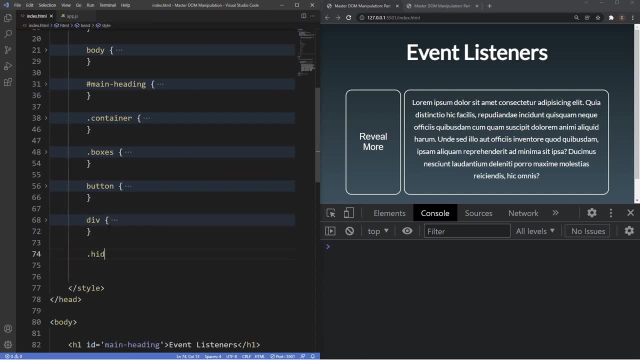 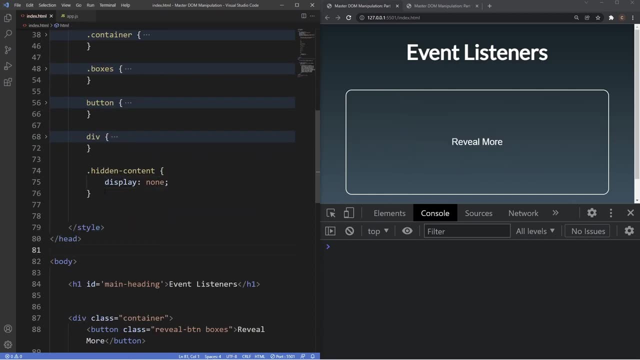 we'll go inside the internal style sheet here, grab the class of hidden content and we'll say: display none and then, when the function runs off and it does include our class of reveal btn, we want to grab the hidden content, grab the reveal btn class and then i want to display as block. so this now: 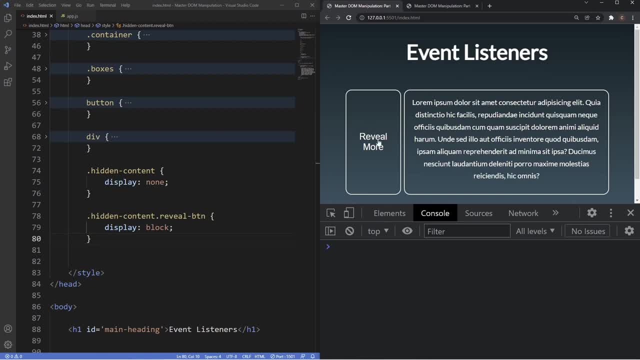 should be working. so if i click on our button you can see it reveals our paragraph. i click on the button again, it hides the content. so what we're essentially saying here is that, depending on the current state of our hidden content here, javascript will either add or remove the reveal. 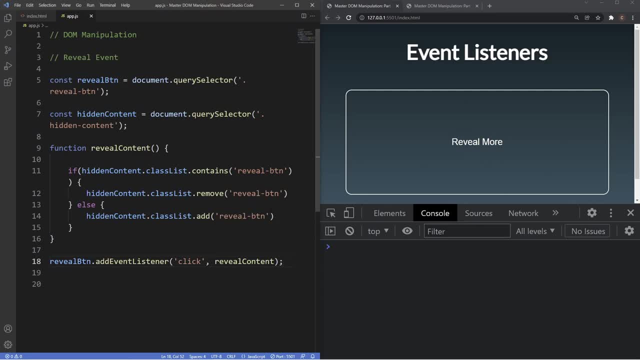 btn and then it will display as block. so this now should be working. so if i click on our button and then it will display as block, so this now should be working. so if i click on our button, btn class, so in its current state right now, this button here does not have the class of reveal btn. 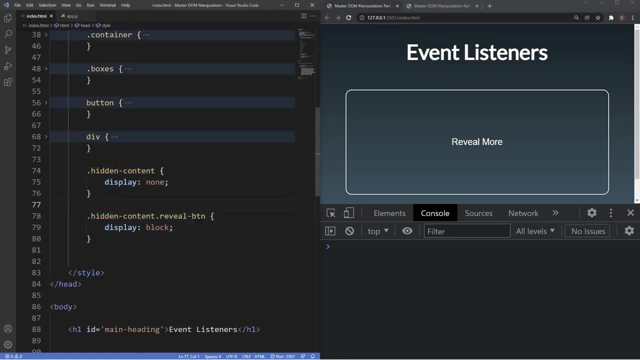 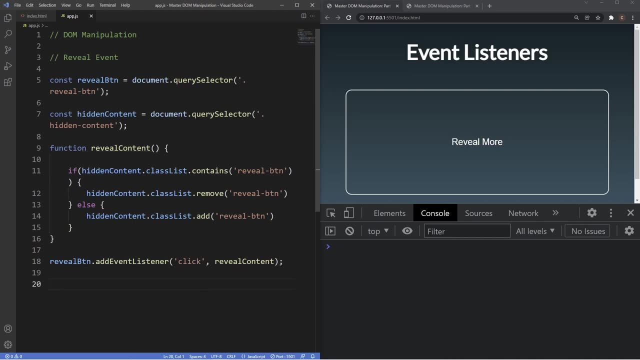 and hence why it's not displaying, because we've set this here to none. when we do click on this button, it will display as block because we've added our event listener here, which looks out for a click. it will run through this function. it will check here if it does contain the reveal btn. 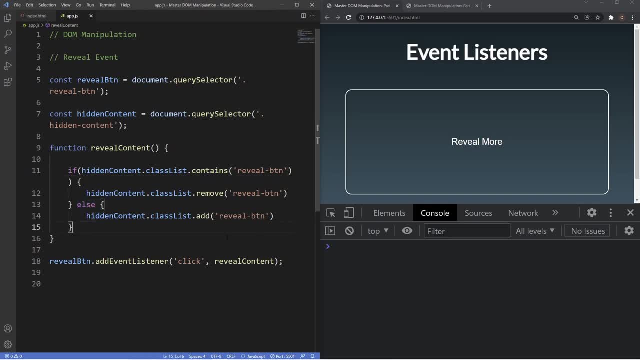 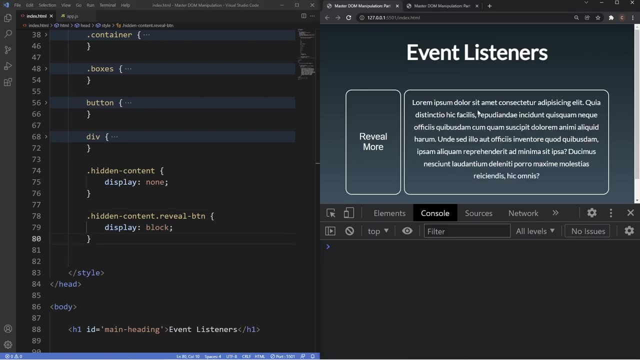 which it doesn't. so if it doesn't, we've got our else statement here which will add that class of reveal btn and because we've set it as block here, it will now display it if we click on the button. and, as you can see, it's displaying it now. and if we click on the button, it will display it now. 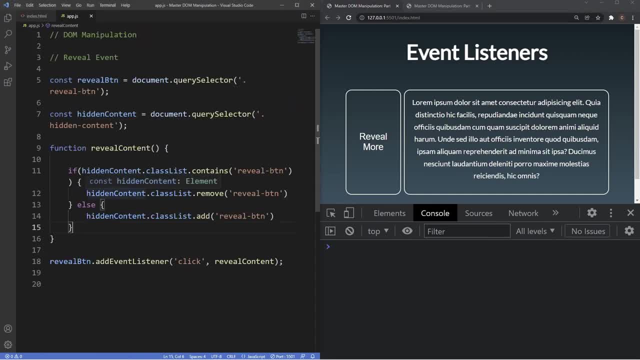 and if we click on this button again, it will run through our function here and it will first check if it contains the class of reveal btn, which it does currently in this state. so it will remove that class of btn and because in our internal style sheet here we've set the display to none, 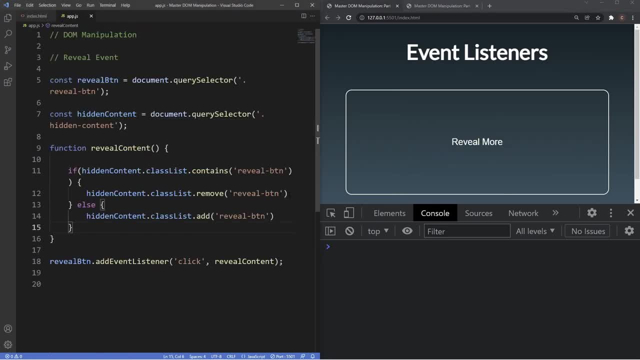 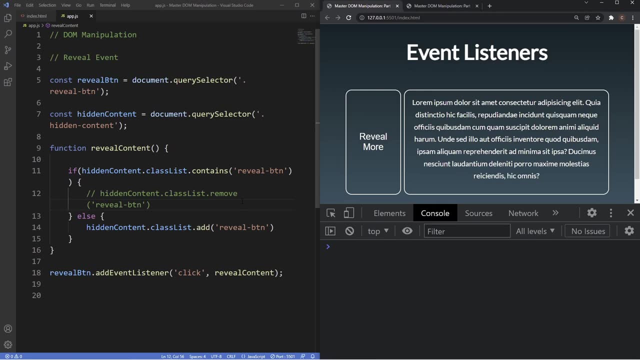 it will effectively hide our content and just show us the button here. so if i just show you guys what that looks like, if i just comment out the remove section, if i click on the button, it will display it because currently, right now, it's added the class of reveal btn. but if i click on this now, 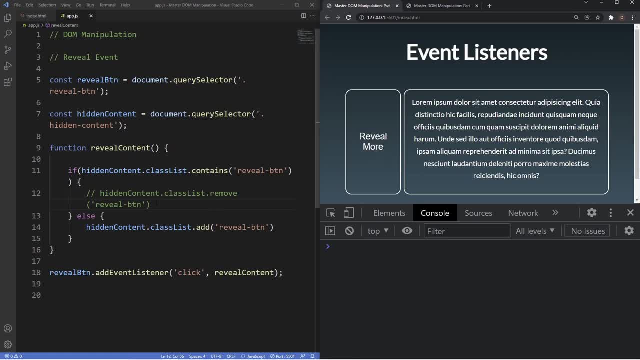 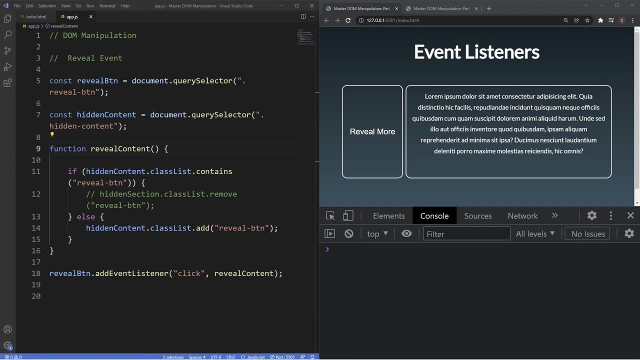 you can see, now it's still displaying the text, because in our if statement here we no longer have the ability to remove that class. so that's how we can create a really basic reveal hard functionality using event listeners, which looks pretty simple, but this technique actually can be used for many different things. 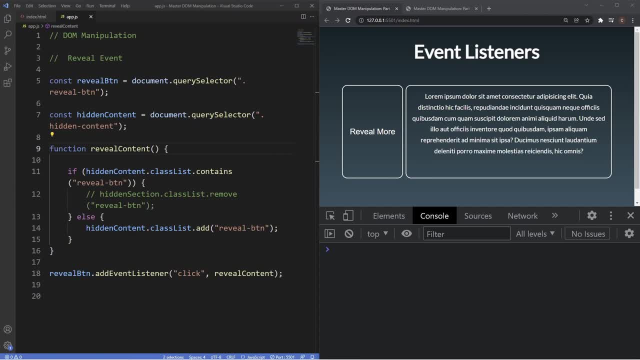 so, for instance, you can use it for things like toggling a menu on small screens, so when you see that hamburger menu, or you can display error messages with this, and many more things you can do. so, guys, that's how we can create events in javascript, how we can fire off different 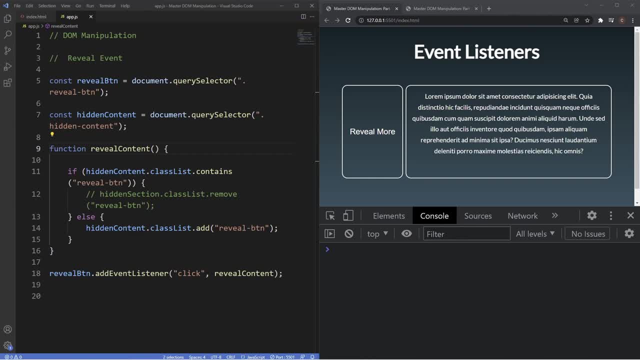 types of events. and again, there are loads of different types of events we can create and i'll leave a link in the description for you guys if you guys want to check those out now. this is actually just scratching at the surface of event listeners. there are some things lurking underneath or, more appropriately put, lurking behind the scenes. 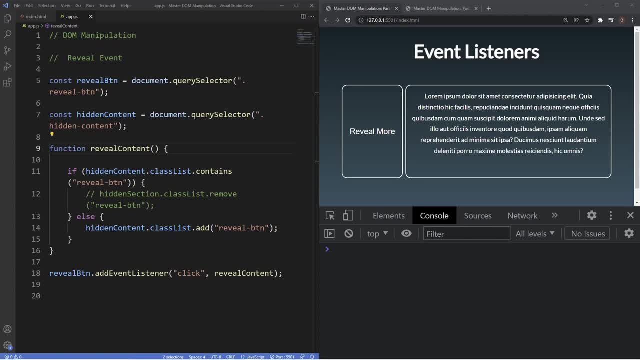 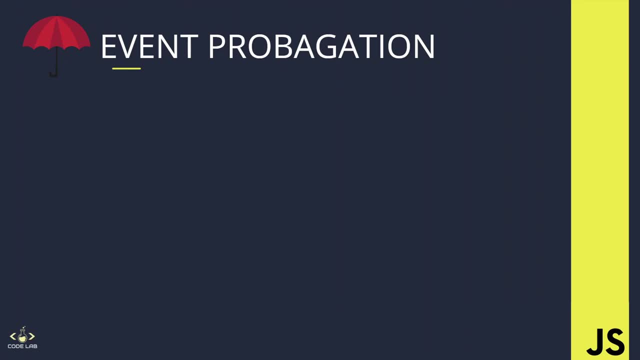 of event listeners, and that is event propagation and event delegation. let's first take a look at what event propagation is and what it means now. event propagation refers to how an event travels through the document, object, model or the dom tree, and you can think of event propagation. 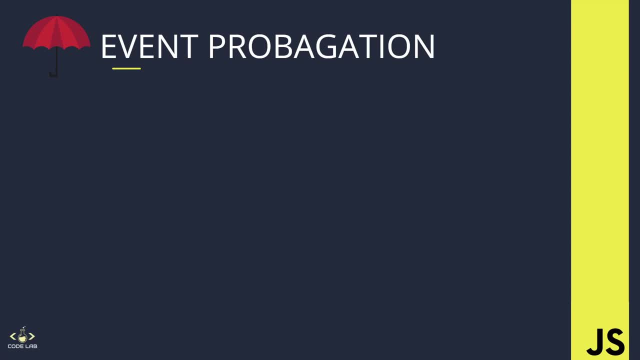 as electricity running through a wire until it reaches its destination. now, as we're fully aware, the dom is full of nodes and when we're referring to event propagation and events, the event needs to pass through every node on the dom until it reaches the end, or it's forcibly 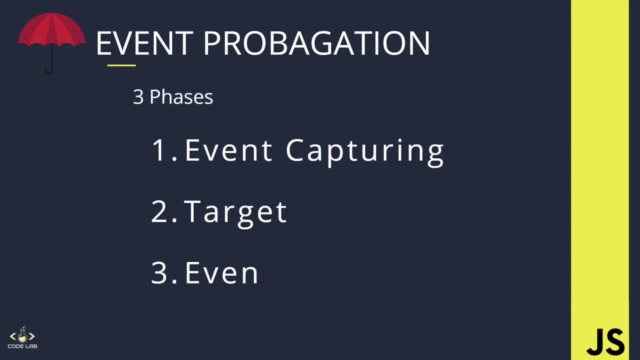 stopped now. event propagation is also the umbrella term which is used to cover three phases when dealing with event listeners. you first got the event capturing, then you've got the target and then you've got the event bubbling. now, in the simplest definition, the capturing phase starts. 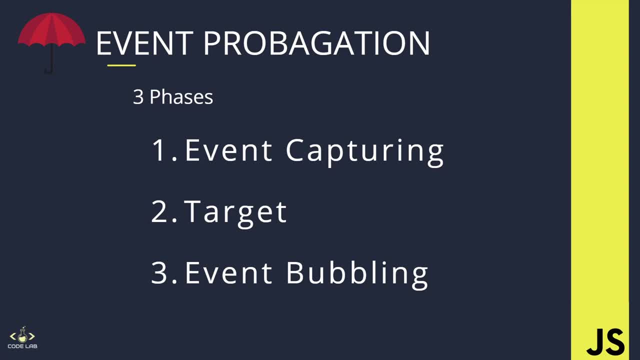 from the root and travels all the way to the target. after it's reached the target, it goes into the bubbling phase, which travels back up from the target to the route. so to better understand this, let's take a look at a visual representation of the event propagation. 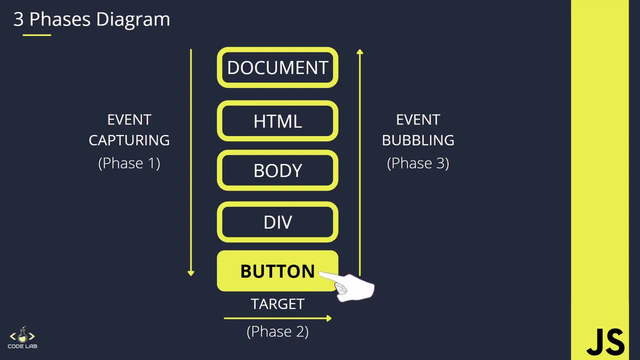 so in this slide you can see we have a basic diagram of our three phases. now imagine that our button at the bottom here has a click event attached to it and is being clicked. now, when this happens, javascript behind the scenes starts three phases. first it begins with the capture phase. 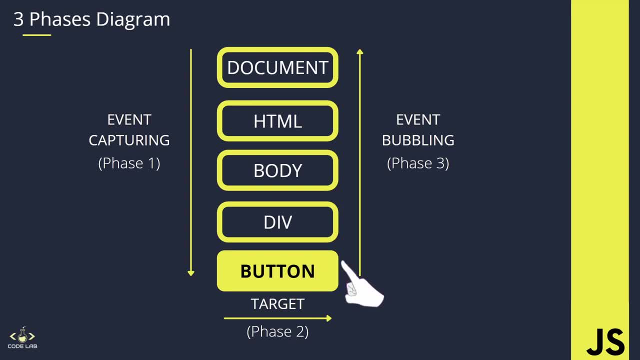 where it starts, at the highest level of the dom, and it will trickle all the way down. i will notify each element. so it will notify the html element, the body and the div and tell it that something underneath it is being clicked. so again going back to that analogy of electricity, 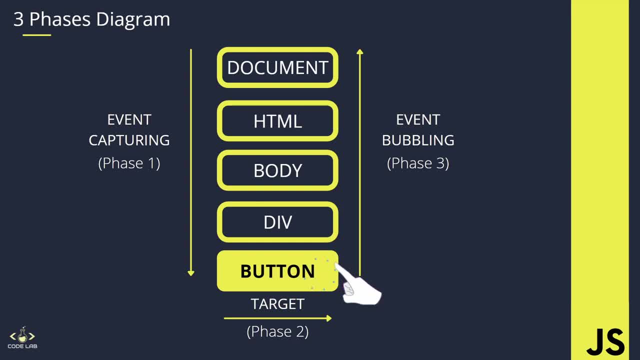 running through a wire, so this will trickle until it reaches the target. and then, when it reaches the target phase, this phase is a dom node in which we click. so in our example, the button here at the bottom has a click event attached to it. so this would be the target and essentially our target. 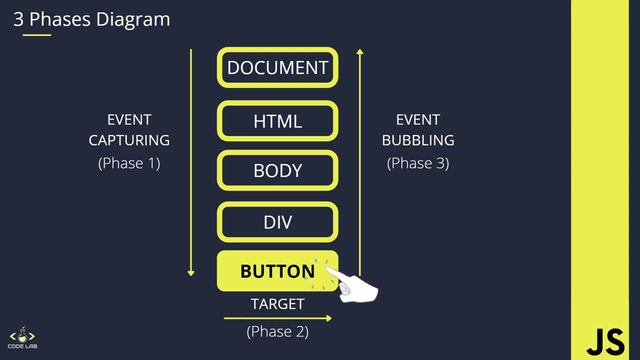 phase. so once this target phase is triggered, the next phase is what we'd call the bubbling phase, which is essentially just the opposite of the capture phase. this travels back up the dom and notifies every element, so the div, the body, the html, the document, all the way up to the highest. 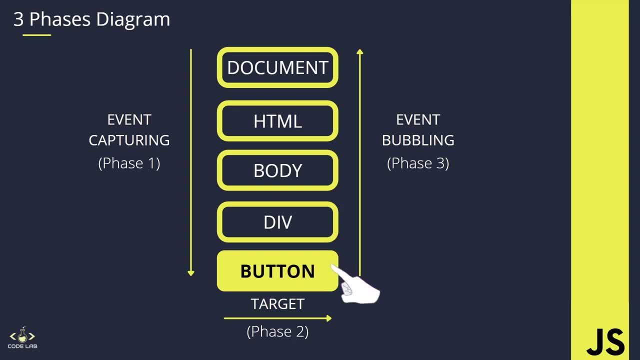 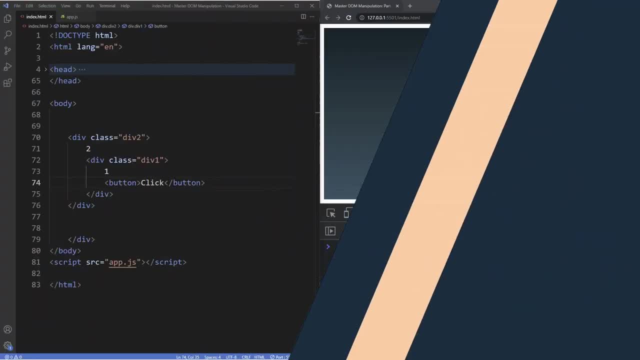 level parent of the target. again, this is all happening behind the scenes and is almost the same as the previous phase, so we're going to take a look at what this looks like in the browser and the console. all right, guys, so we're inside vs code here and you can see in our example here: 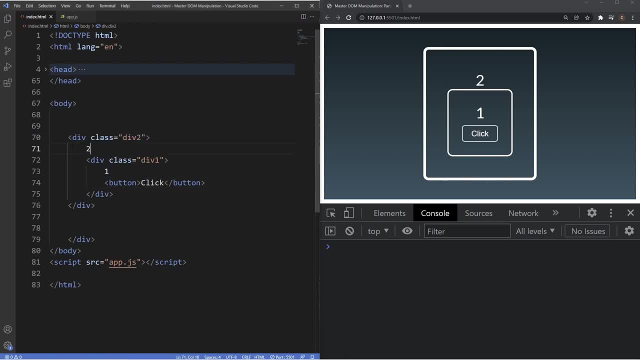 we have several elements nested inside of each other. if you take a look at the html, the markup is pretty simple for this. so we've got our div, which has a class of div2. inside of that we've got another div with the class of div1 and then, inside of that, div, 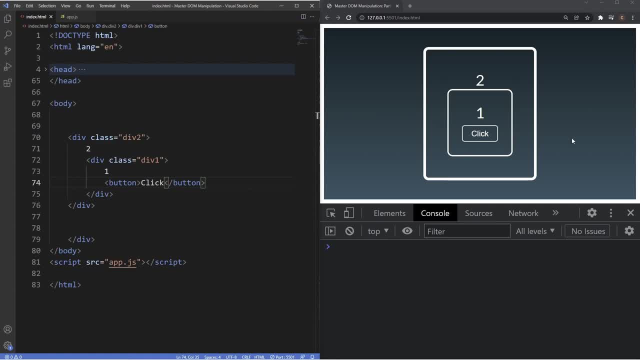 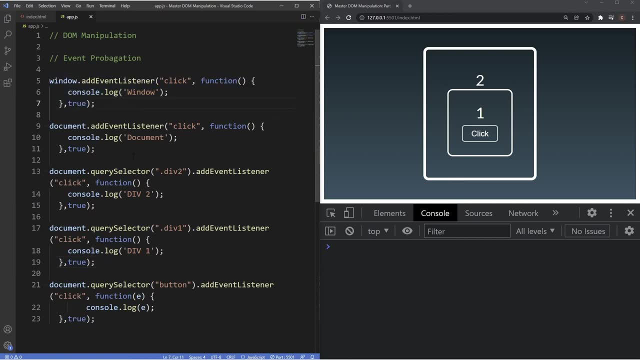 we have a button element, so this is what it looks like in the browser and, as you can see, it just has some basic styling. now, if we head into the javascript here, you can see we have event, the dom tree. so we've got one for the window, we've got one for the document, we've got one for the. 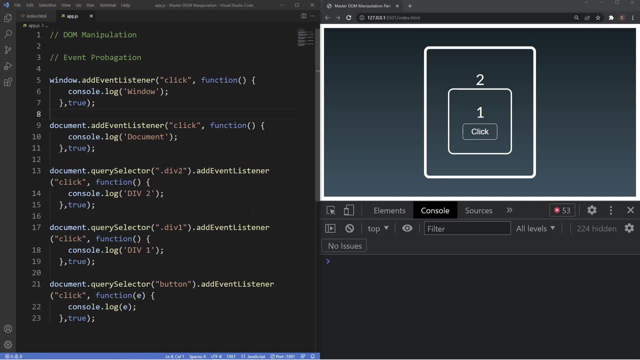 div 2, div 1 and then the button here. now, as you can see, i've set this up a little bit differently in regards to the event listeners. instead of creating a variable for the window, the document as well as the elements here, i've just added the event listeners directly after now creating a. 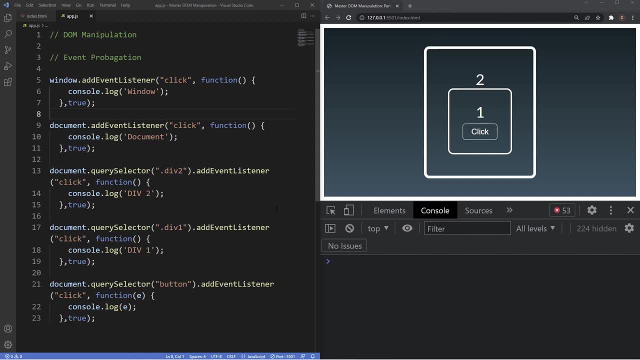 variable and doing it this way both work perfectly fine, but for this example, there's less code here and it just saves me scrolling up and down a bunch of times, which can be a pain for people. now in regards to the events themselves, you can see here, we've got a little bit of code here and we can 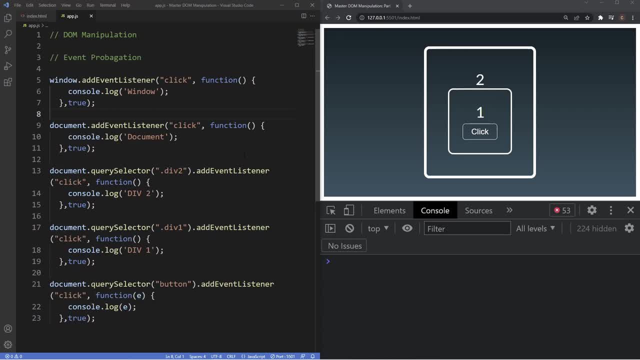 see their click events. and as for the functions, they just simply log in their respective name in the dom tree, except for the button here. now, instead of the text you can see we've included the e inside of the functions parameters as well as the inside of the function. we're logging in that e now. i will. 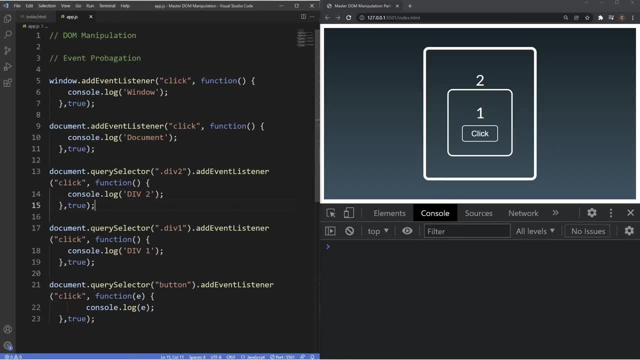 explain what this is in just a moment, but first i just want to draw your attention to the third parameter inside of all these event listeners. so if i highlight them all for you now, you can see they all have a boolean value of true. now, if you guys remember, back to a bit earlier in the video. 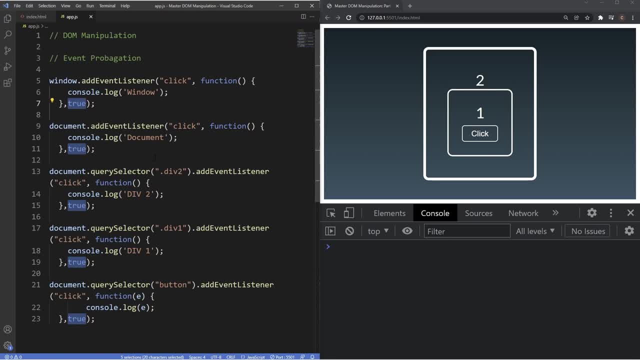 when we were learning about the ad event listener method, there was a third optional parameter we could include. well, this third parameter dictates whether we want to use event capture or event bubbling. so let's go ahead and click on the button here in the browser and see what this gives us in the console. so, as you can see now in the console, 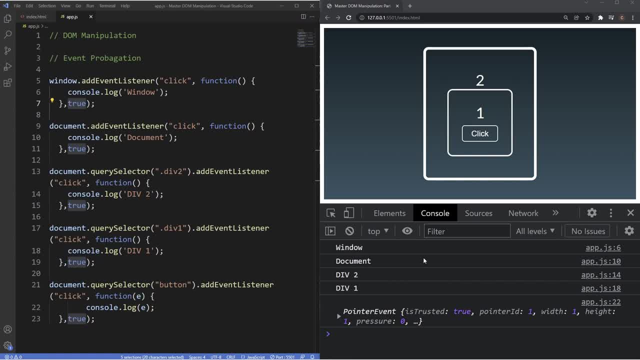 it's giving us the first phase, which is the capture phase. so it's starting from the window and then it's going down and notifying all the other elements it comes across all the way down to the target, which is saying: is this pointer event? now the stuff that you see here represents all. 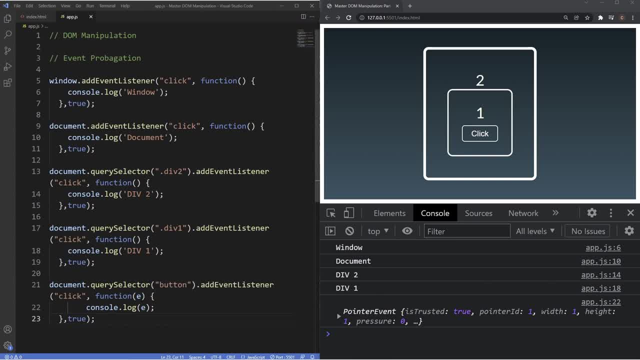 of the information about that event. so this is exactly what that e means inside of our function here, which is inside of our button. so this e represents the event object and, again, this is exactly what you see here in the console. all this information is about that event that has. 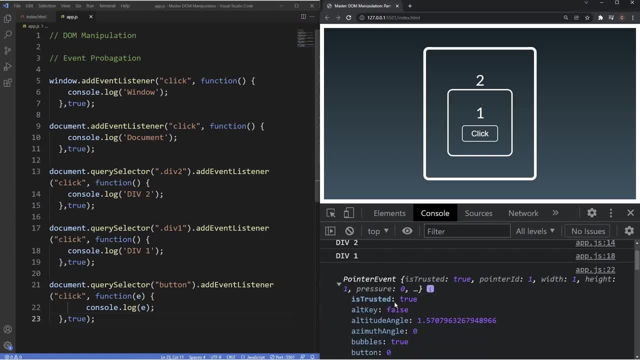 occurred on this button. so if i open this up, you can see all the different properties and information about our event here. so we've got all sorts of things we can take a look at and utilize so we can find out what type it is. we know it's a click event. we can check out where exactly that. 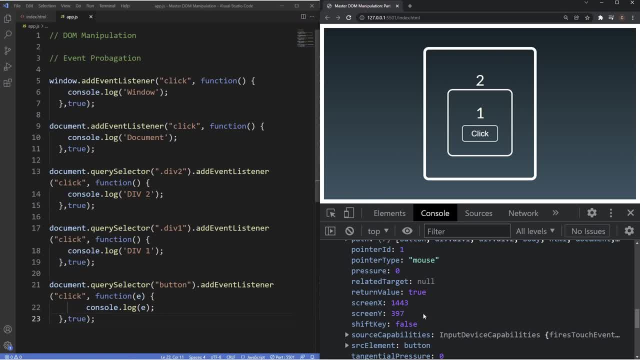 button is exactly on the screen in a browser, on the x and y axes. we can also check things like whether the shift key here has been pushed down, saying false because we didn't use the shift key. so all sorts of things that we can use here and utilize. now, the main property i want to bring. 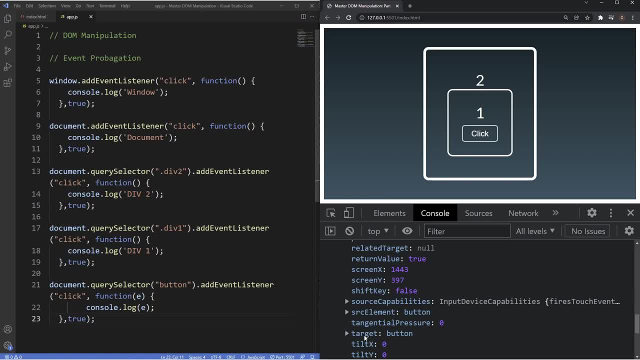 your attention to, and the relevant one to the three phases, is the target property here. so this, here you can see, is saying the button. so this property represents the element that the event is actually on. so again, it relates to our target phase. so if i actually go into our console here, 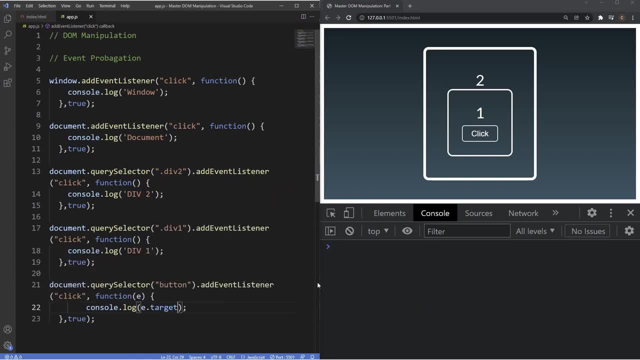 and i type in here, dot target, and i'll just refresh this and i click on the button again. you can see now it's starting from the window going to the document: div 2, div 1, because we're using the target property to show us what element the event is on. which again, is our button now again. 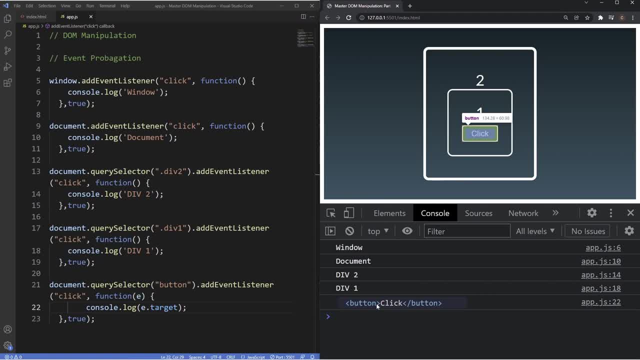 we can do some other cool things here. so let's just say, for example, when we click on this button, um, we'll just change the text to say clicked. so after the target we say dot in our text and set this to. let's equal it to say clicked. so what should happen if i click on the button? 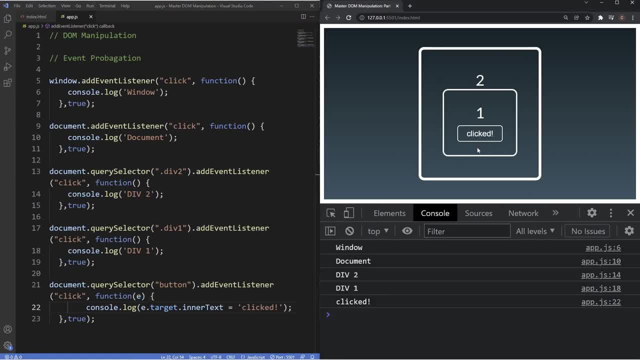 it should change the text to clicked. so, as you can see now in the console, when we've clicked the button, it's changing the text to click, because what we've done is use the event object to grab the target, which is the button, and then from there we use the inner text property. 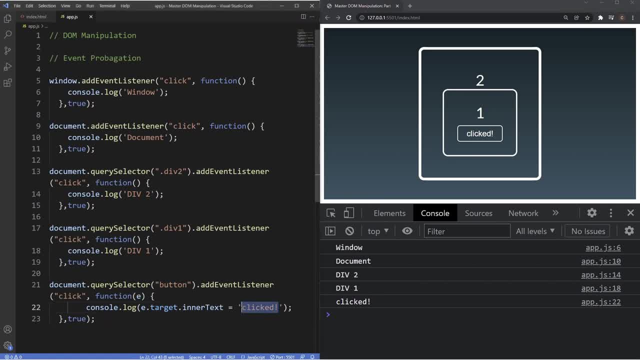 and then change it to click. so when this function fires off the button, text change to click. so, as you can see here in the browser and if you also take a look at the console, you can see we also see phase one, so the capturing phase. so we start the window document div 2, div 1, and then click. 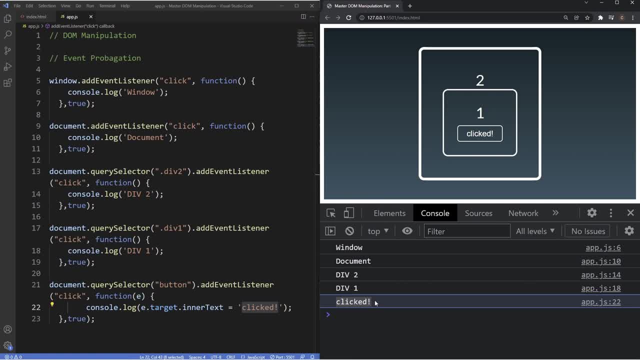 which is the button. so that's the first and second phase. how do we now initiate the third phase, which is the first phase? well, to do that, all we need to do is just grab all of the true values here for our third parameter and just change them to false. now, these are actually false by default. 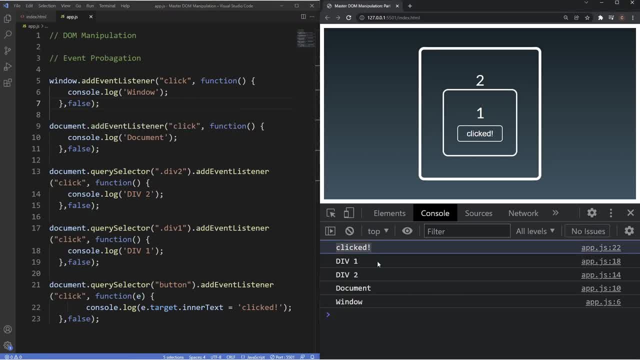 and if i click on the button now, you can see it's starting from the button and then it's going to div 1, div 2 document and then the window. so it's bubbling upwards, hence the term event bubbling. so from the target it's bubbling up to the highest position in the dom tree. now there are ways we can. 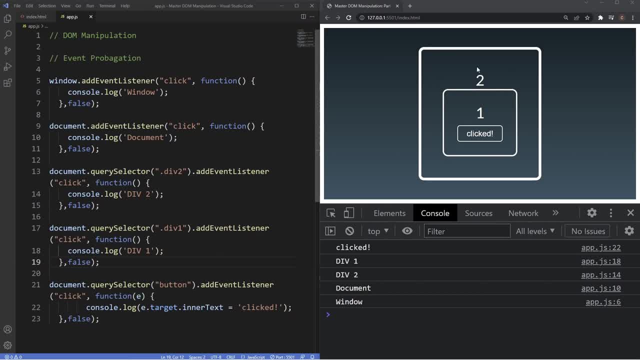 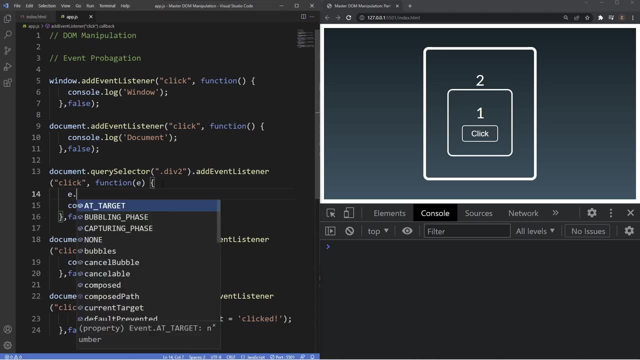 actually stop event propagation. so let's just say we wanted to stop the bubbling um to have the second div. we can do that with the stop propagation method. so let's go to the second div here include our event object. then inside of here we'll just say e dot, stop propagation. so what? 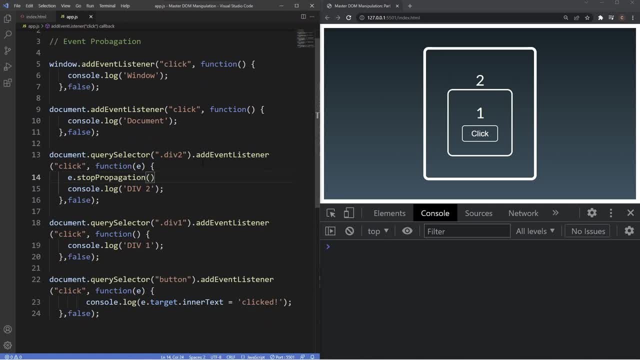 should happen now is when i click on this button once it reaches the second div. we want the propagation to stop so we'll no longer be able to see the events on the document and the window. so if i click on this, you can see it's going from click to div 1, div 2, because we've stopped. 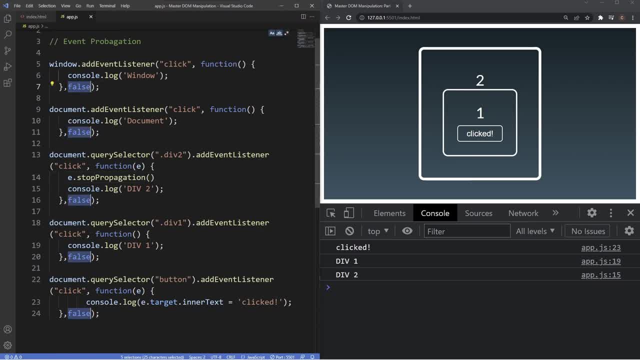 the propagation at step 1 and we've stopped the propagation. now let's take a look at the third parameter here and see how that changes. so i'm going to go to the third parameter here now. this also applies to event capturing. so if i grab all of the third parameters here and change, 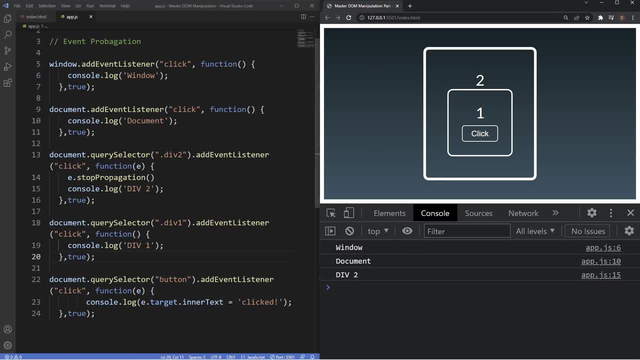 them to true. so we're in the capture phase and then i click on this button. you can see the opposite is happening, because we're starting from the window where the cap, where the capture phase, begins, then go to the document and then go to div 2 and then stops at div 2 because we've stopped. 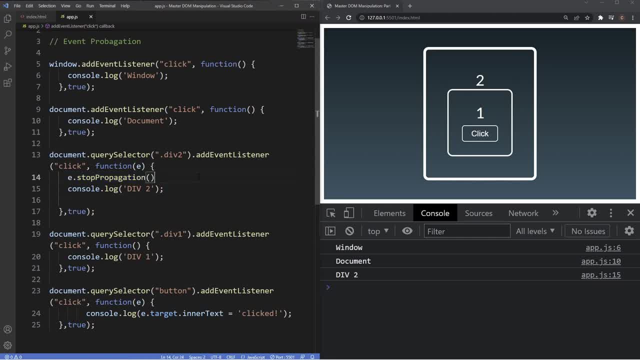 the propagation. so that's how we can stop event propagation happening for capturing and bubbling. and i'm just going to comment out the stop propagation method there. take out the e and then change all these to false, even though they're false by default. we'll just keep it like this. 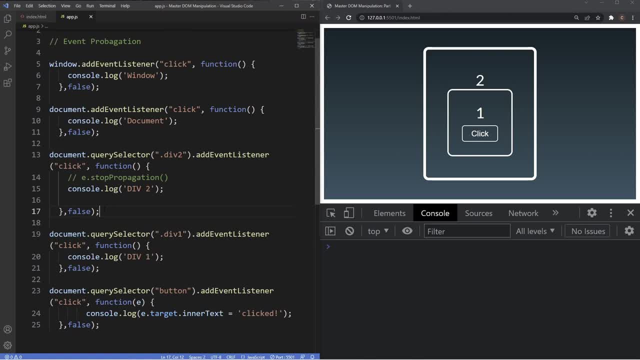 for consistency. so again, if we only want div 2 to fire off once for our third parameter here, what we can do is grab the once property and set this to true. now, if i click on this button, you can see it fires it all off as normal. so it starts from the click and bubbles up all the way. 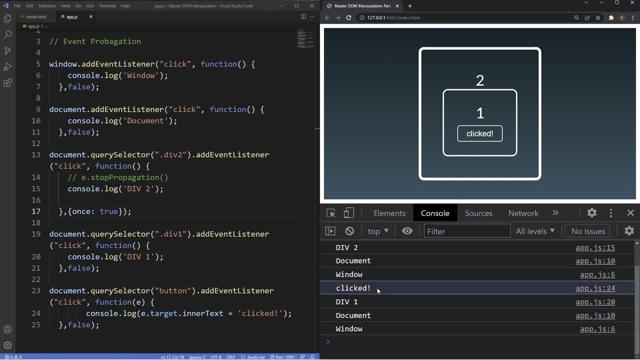 to the window. if i now click this button again, you can see it's starting from the button or the target going to div 1. but now div 2 is no longer firing. and then it goes on to the document and then the window and then again, if i click this again, you can see the div 2 event isn't firing. 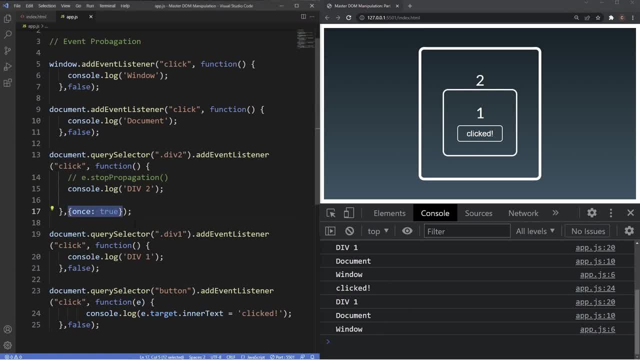 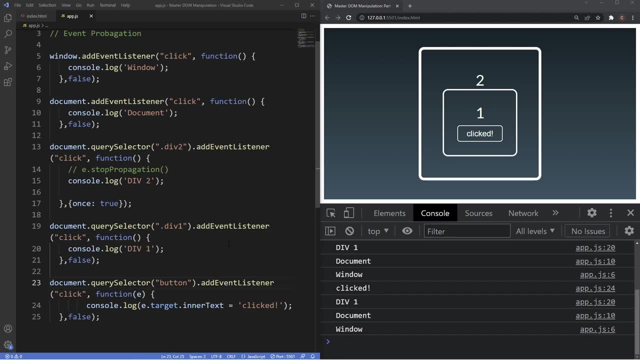 off because, again, what we've done here is define that we only want this event to fire off once. now another common method you likely run into is the prevent default method. now, what this method does is pretty self-explanatory really. it just prevents any default behavior that might. 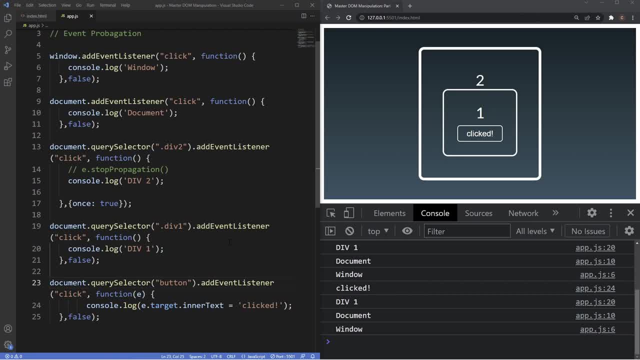 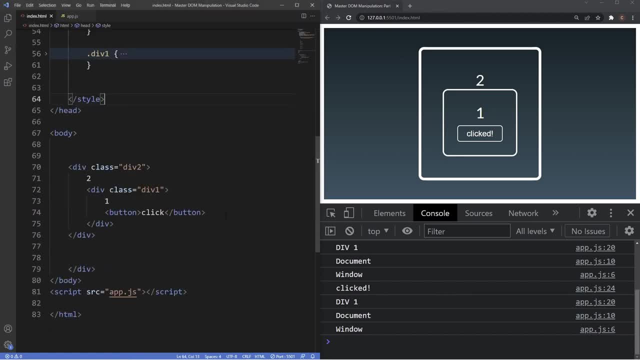 occur in the event. so if i click on this button again, you can see it fires off all the way to an element or an event. so this is quite dependent on the type of element involved in the context of an event. so to see example of the prevent default method, what i'm going to do is go into the indexhtml. 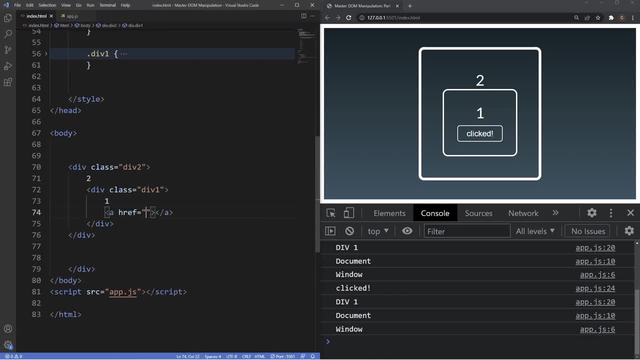 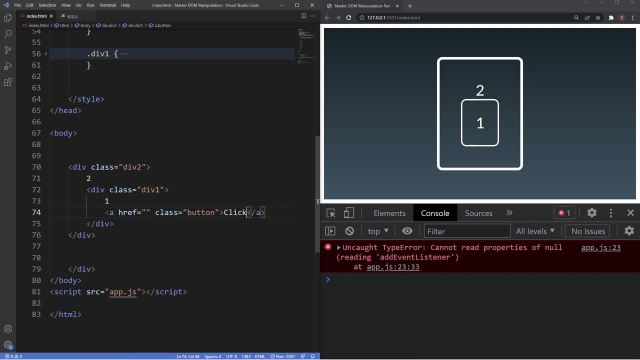 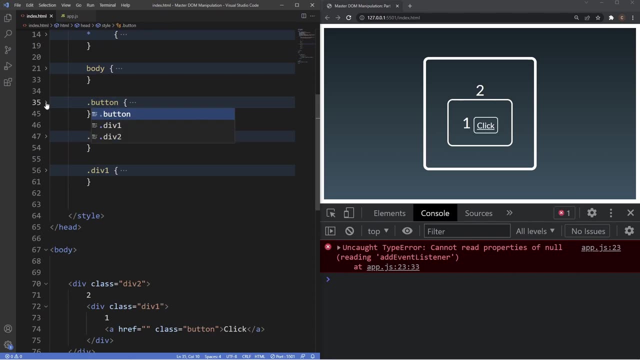 and i'm just going to change the button to an anchor tag and i'm going to give this a class of a button and i'm just going to put in here: click, and then we'll go where the styling is for the button and we'll make this a class, and then what we'll? 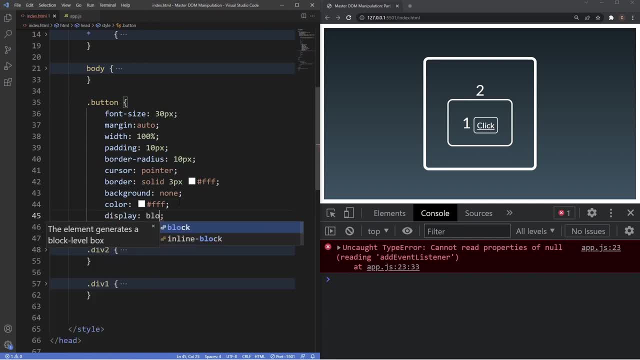 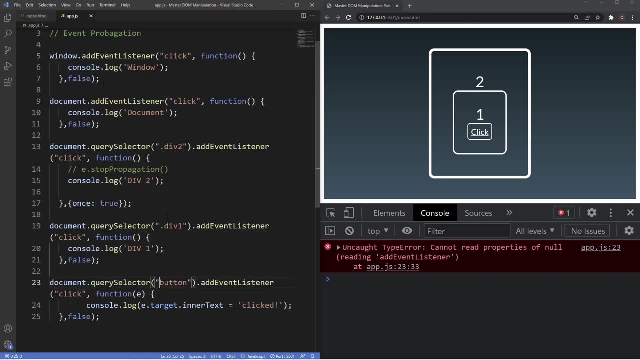 also do is just put it on a new line. so we'll say display block, because anchor tags are inline by default. so we'll head into the appjs file and what i'll also do is just make sure our query selector here is targeting that class of button. so our anchor tag now in this event: listener here. 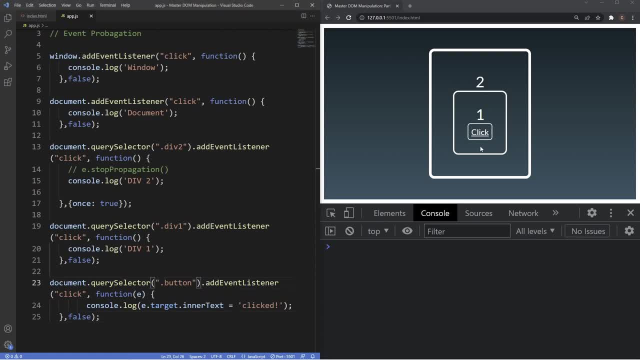 is now the target and the event and because we've changed the button to an anchor tag. if i click on this now, you can see it's firing off all the events, but they quickly refresh and the reason it's doing this is because the default behavior of an anchor tag is to try and 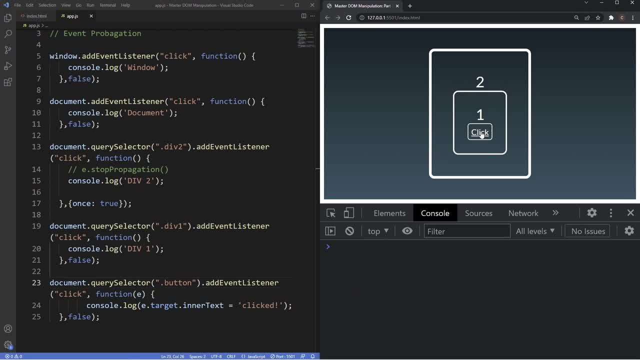 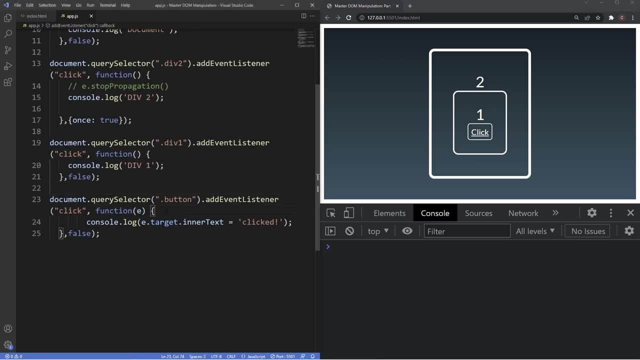 redirect us to somewhere else, and this is what's causing this quick fire off of all the events and then a refresh. now we can stop this from happening with the prevent default method. so to do that, we'll go inside our button here, or the class of button, and we'll grab the event: object: prevent. 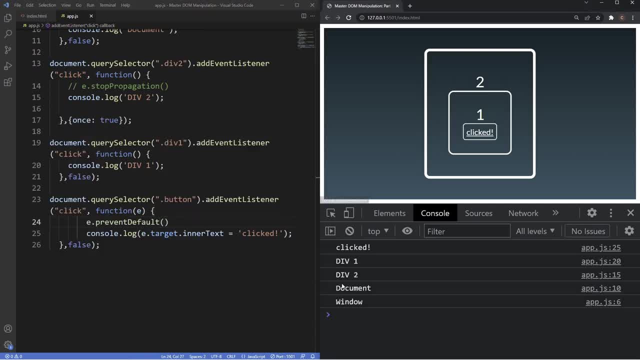 default and if i click on the button now, you can see it's showing us the bubbling phase. the content has changed the click, that it's staying and we can see that the content has changed the click there. and all this has happened now is because we apply the prevent default method onto our anchor. 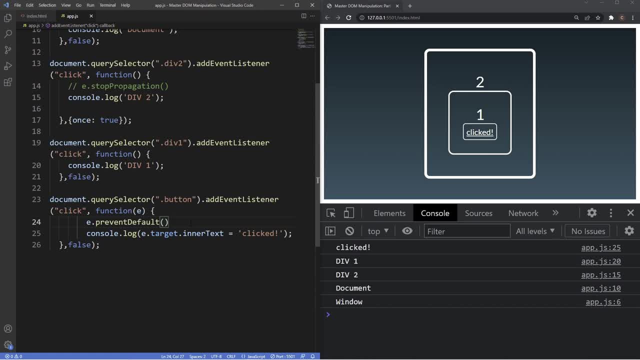 tag so it's no longer trying to direct us to somewhere else. now we will see a more practical example of all the methods we just learned. so the prevent default, uh, the stop propagation in part two of the tutorial where we look at practical examples and projects. but i just wanted to make 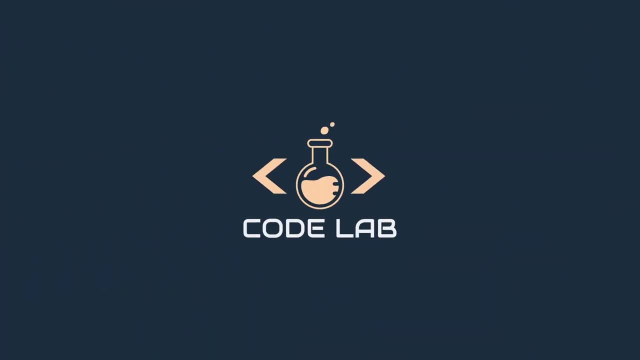 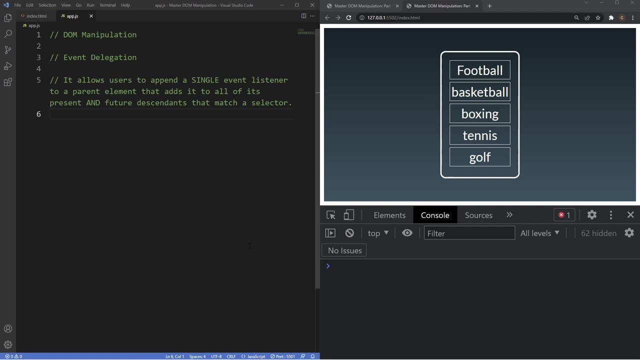 you guys aware of these, um, so they don't confuse you in that subsequent video. now, the last thing i want to mention in this tutorial, guys, is event delegation. now, event delegation is one of the most potent event handling patterns inside javascript, and the best way to do that is to. 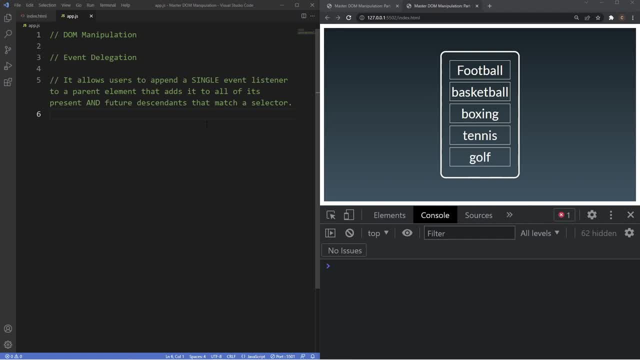 use the event delegation to do a single event listener to a parent element that adds it to all of its present and future descendants that match that selector. now what we'll do is actually break this definition down to show you guys, exactly what it means. now the first part here, where it says: 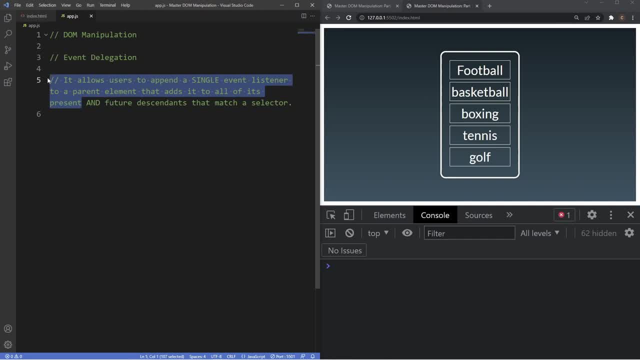 it allows users to append the single event listener to a parent element that adds it to all of its present children. to find out why this is useful, let's actually just go back a few steps and see how we get to event delegation. so if we head back into the indexhtml file, you can see: 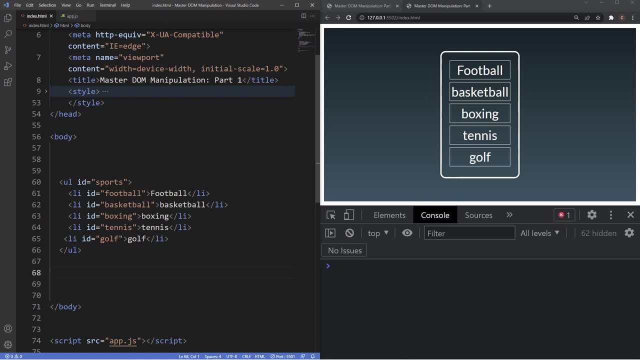 we've got a lot of different things here, so we're going to go back into the indexhtml file and we're going to go ahead and unorder list, which has a bunch of different sports inside of it. now this unordered list has an id of sports and then each of these list items have their own id, which is: 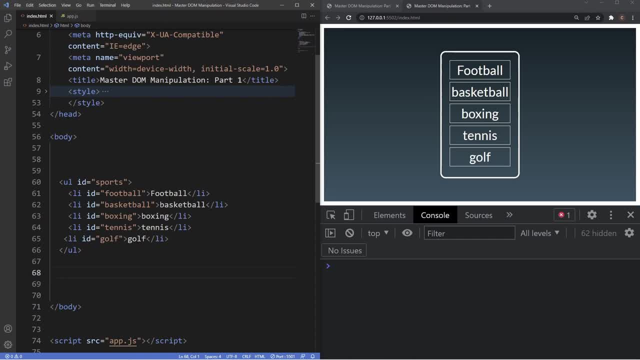 equivalent to the content that you see inside of each of the list items and this is what it looks like in the console. now, if i click on one of these list items, you can see it's showing us in the console that football's click and it also changes its background to a light gray, again to highlight. 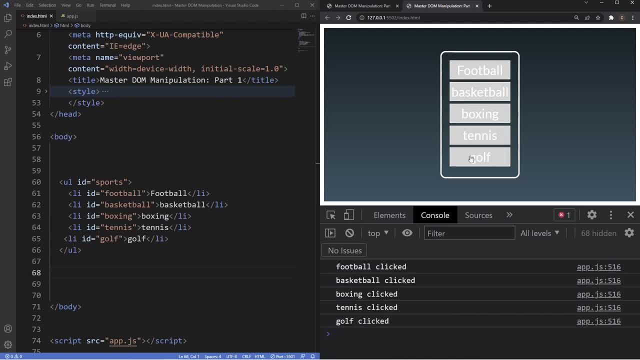 that it's been clicked and again, this is going to be the same for each individual list item. now, to achieve this, what we can do is apply event listeners to each individual list item that we have inside our unordered list, so we'll head into the appjs file. 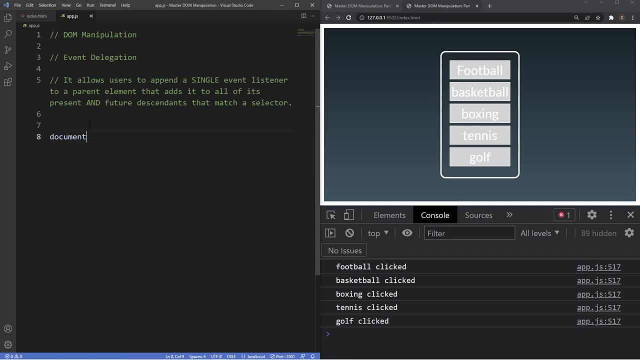 and we'll grab the first list item. so we'll say document dot, query selector. grab the id of football, add the event listener and we're going to look out for a click event. grab a function. inside of the function we'll include the event object and then inside of this function what we'll? 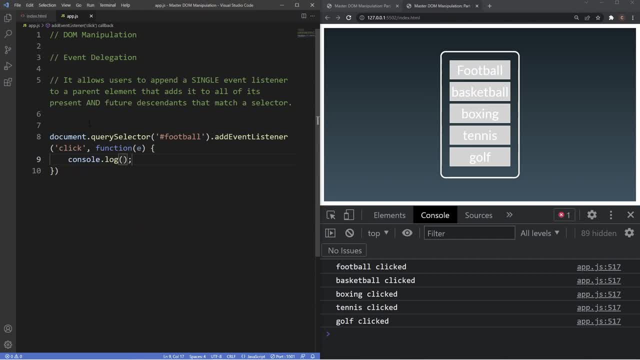 want to do is first just console log in. let's say, say, football is clicked, and then the next thing i want to do is change that background color when we click on the actual list item. so to do that, we're going to first need to create a constant. so we're going. 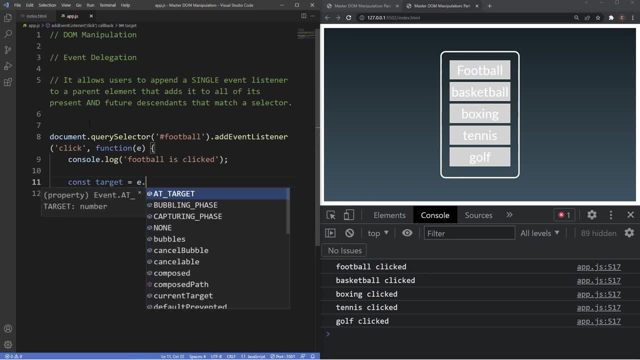 to say: call this target and this is just going to equal e dot target, which is that list item. if- and the condition we're going to put in here is if target matches. so matches is just a method, basically, which essentially checks of the target which, in this case is the list item, matches with. 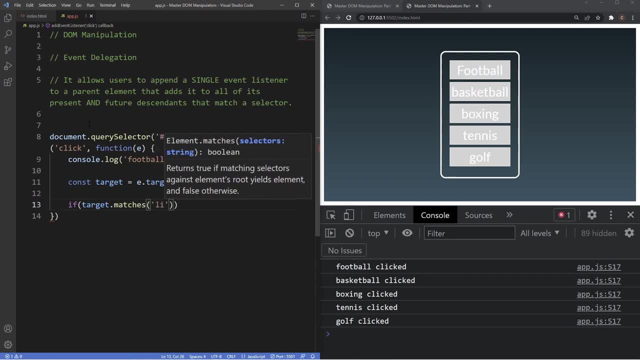 our css selector, which is going to be li. this is going to return true and then, when it returns true, it's going to change our background color. so, after a condition, we want to include the code that we want to execute. so we're going to say target dot style. 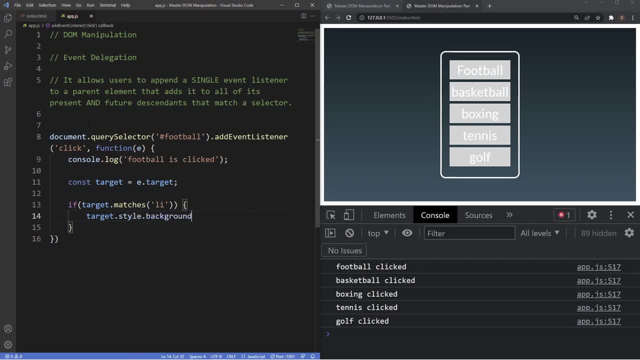 dot background color and we'll set that to light gray. and if we head into this folder's live server here you can see we have the exact same layout and what should happen now. if i click on the football list item, the background should change to a color of light gray and it should also show here in the console. so if i click on 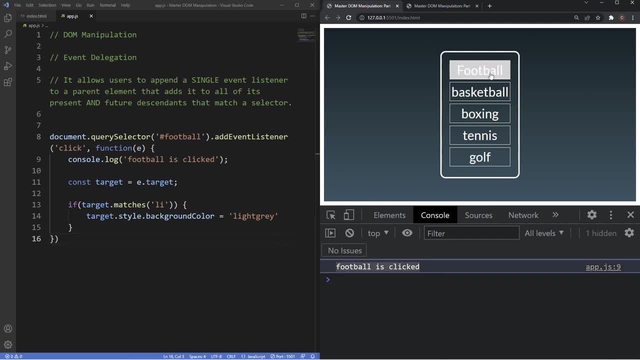 this you can see it's saying football is clicked and then it's changing the background to a light gray because we've just created an event listener for it inside the appjs file. now again, if we wanted to do it for all of these, what i'd need to do is just duplicate this four more times. 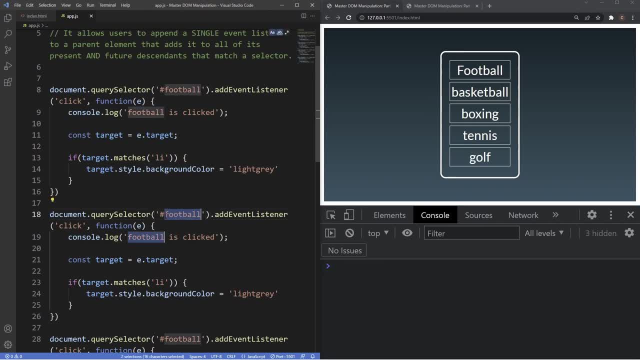 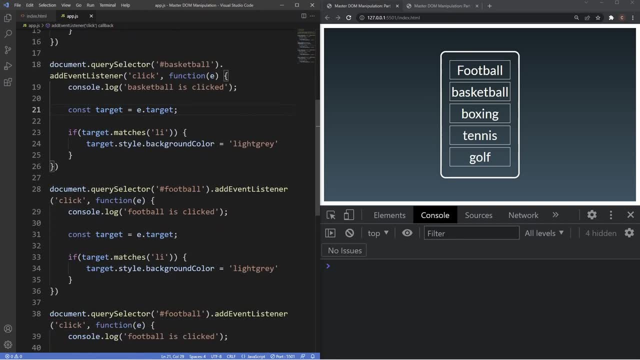 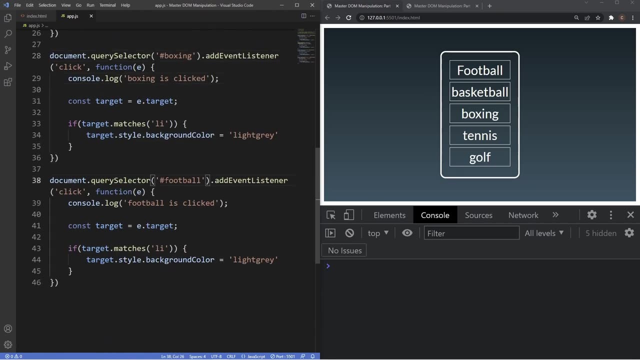 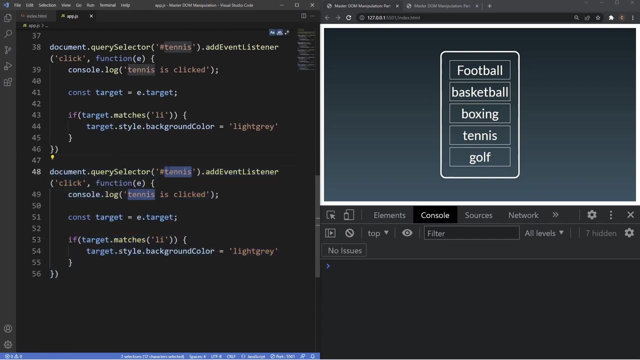 so instead of football here we have basketball, and then for the third one we have boxing, for the fourth one we have tennis, and then we'll create one more for golf, and now all the styling and the console logs should be working for each of the list items. 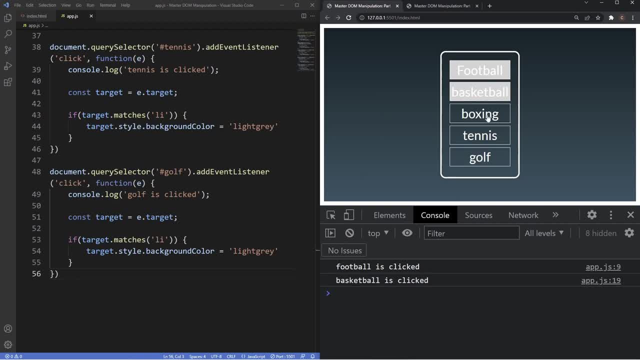 so we'll start with football. see, that's working. basketball's working, boxing's working, tennis and golf are also working. so we're getting the exact same thing as our draft example here, except the text is a little bit different, but again it's the exact same styling. 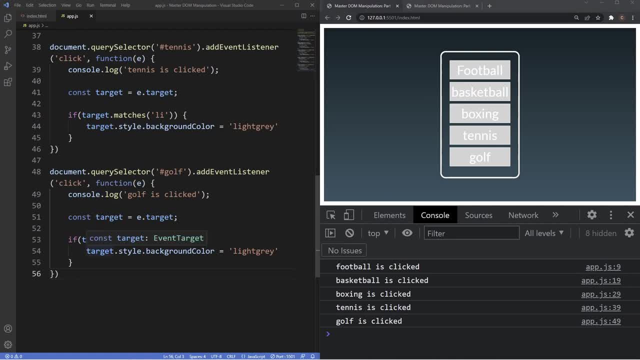 and you can see it's working perfectly fine. now this is great and works fine. there's no real issue with the code here because we're getting the exact same result as our draft example. but, as you'll learn throughout your code and journey, there are always questions to ask when you have written out. 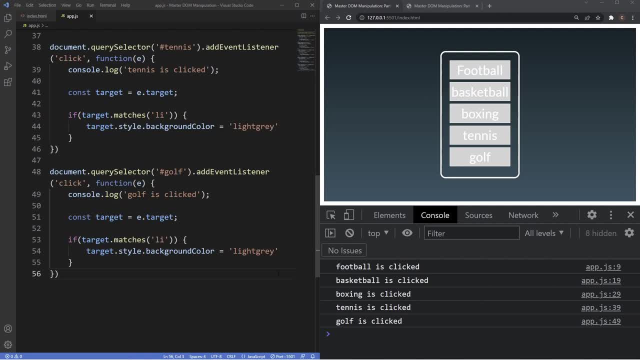 your code to help improve it. so you can ask yourself things like: can we remove some of this code? can we remove some of the event listeners and still achieve the same result? can this task be done writing less code instead, or can we even optimize this code? and the simple answer, really. 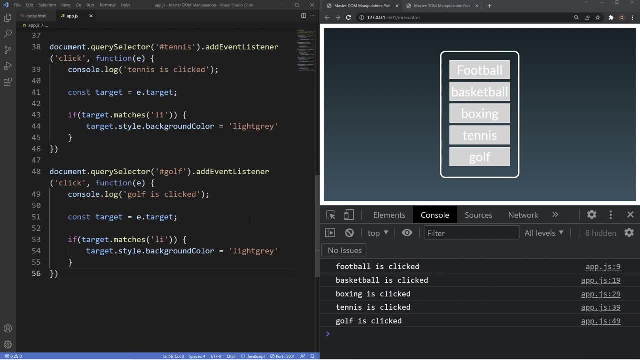 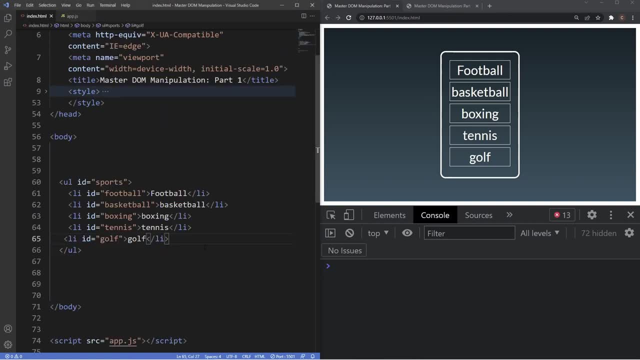 is that we can. we can write less code here and achieve exactly the same result using event delegation. so the idea of event delegation is pretty simple. instead of attaching the event listeners directly to each of the list items here, we can delegate the listening to the parent, which. 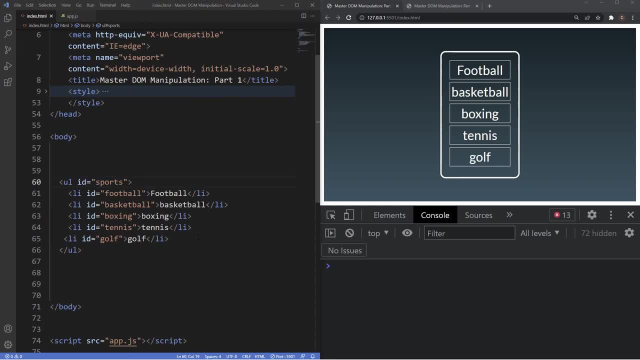 is the ul here which has the id of sports, so that when the li is clicked, the listener of the parent element catches the bubbling event and the performs our task, which changed the color of our background to light gray when we clicked on one of the boxes and also showcased some text inside of our console here. so what we're going to do to 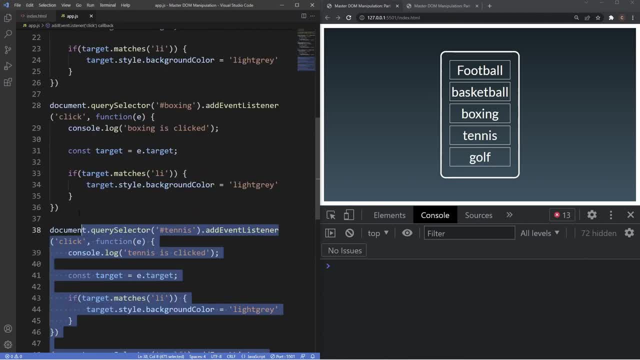 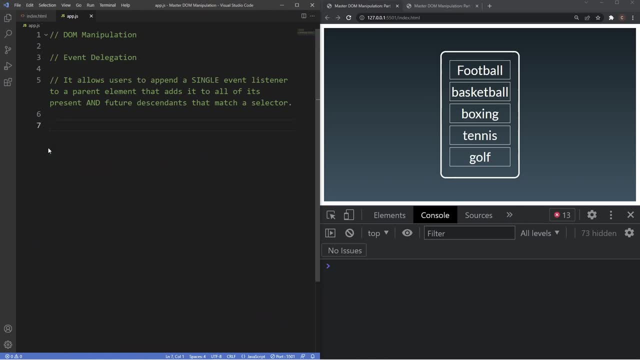 achieve this now is go back to the appjs file and get rid of all this code here, and then we're first going to grab that unordered list element which has the id of sports. so we'll say document dot, query selector, and then we'll say we'll grab the id which is sports. 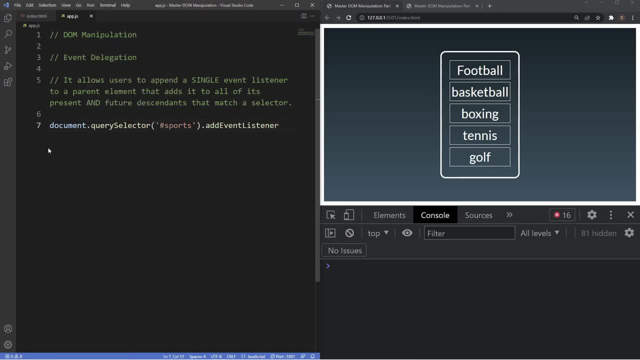 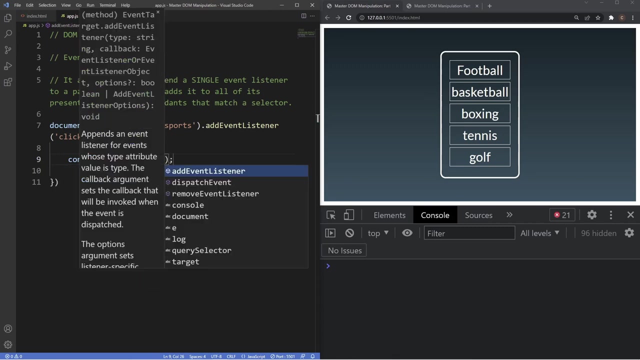 and add the event. listen to this. so a similar process, it's going to be a click event. include our function which has the event object inside its parameters, inside of our function. here we want to say: let's console log that bit of text. so we'll say e dot target, dot get. 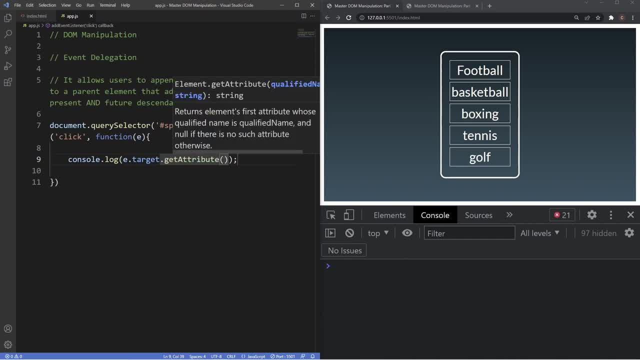 attribute, method of get attribute and we want to say e dot, target dot, get attribute and we want to get the id and then we want to say plus, we'll put in here is clicked. so what we're saying here is that when the target, which is our list items, has an id attribute, 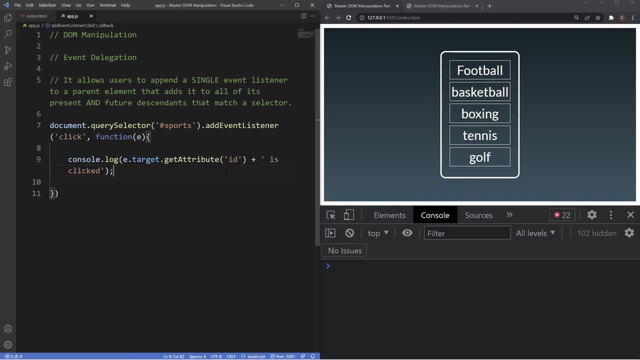 which all of them do. whichever one that we click on will display that specific sport plus the extra bit of text here of is clicked. so if i go ahead and click on one of these now, you can see it saying football is clicked. if i click on tennis, you see tennis is clicked. 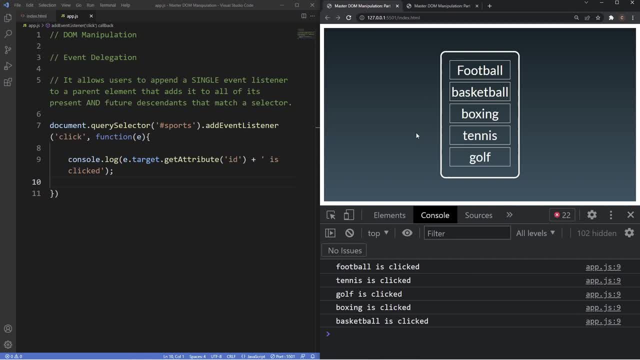 golf, boxing and basketball. so you can see all of these now are working because we've attached that one event listener to the parent element, which catches the bubbling event and then performs our task, which we've written in here. now we also want to change the background color when we click on these. 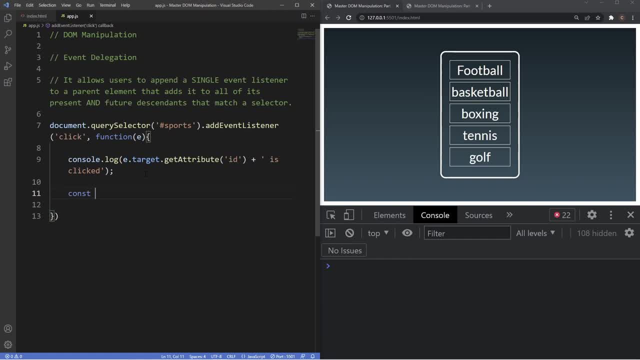 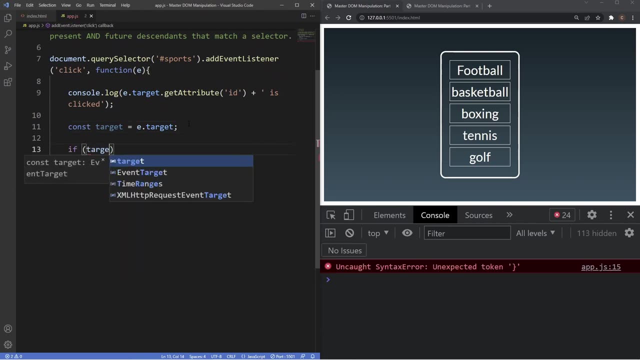 so to do that, first going to need to create a variable of the target. so we're going to say: target it's going to equal e dot target, which is those list items. and then we're going to say if the target variable there matches our css selector, which is our li, we're going to want to change the background, so say: 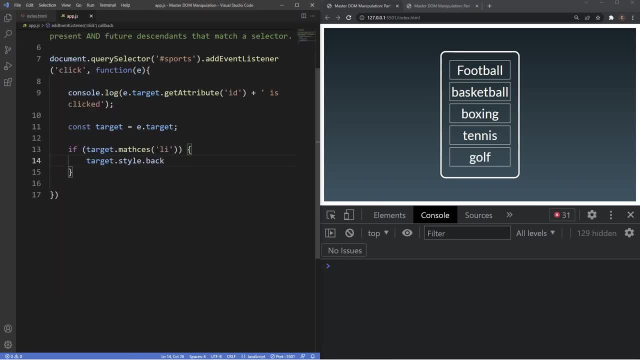 target dot style dot: back ground color to a light gray. so again, if i click on one of these now, we get an error. that's because i spelt matches wrong. so again, if i click on one of these now, you can see the text will appear and the console. 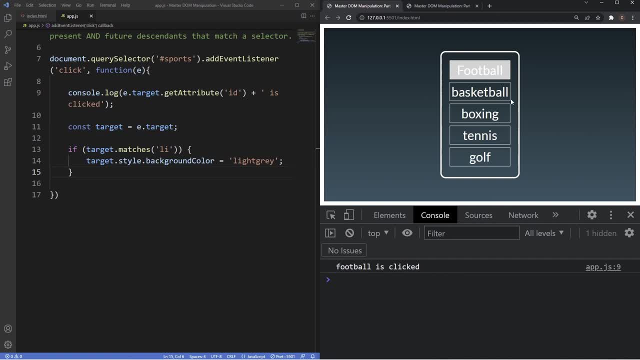 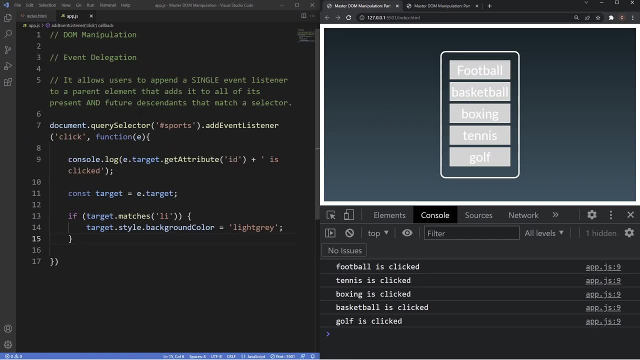 highlighting which one i clicked. and then we also now have the extra feature of where the background changes to a light gray for all of our list items there. now again, this brings us back to our first part of our definition, which allows users to append a single event listener to our parent. 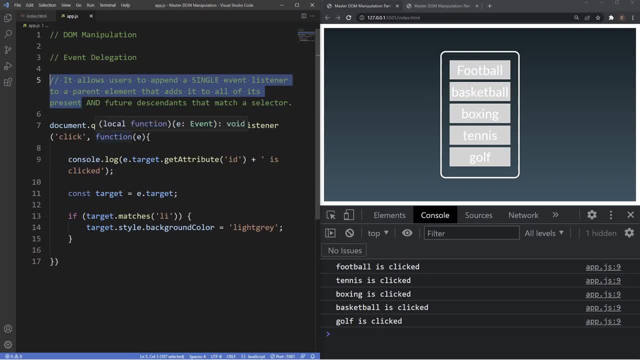 element that adds it to all of its present children and, as you can see, this has clear benefits, ranging from code quality as well as code maintenance, because, instead of having all those lines of code as well as code maintenance, because instead of having all those lines of code in the previous example where we attached an event listener to each of the list items, we now 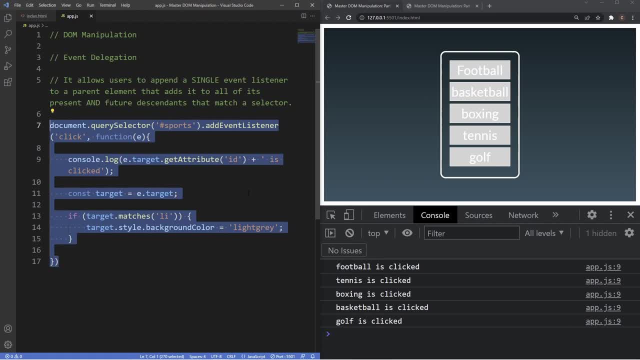 have it all inside one event listener here now we've also improved our performance because having more events in our code will take up a lot of memory, and using event delegation we're going to save a ton on memory, which again will vastly improve our performance inside of our projects. 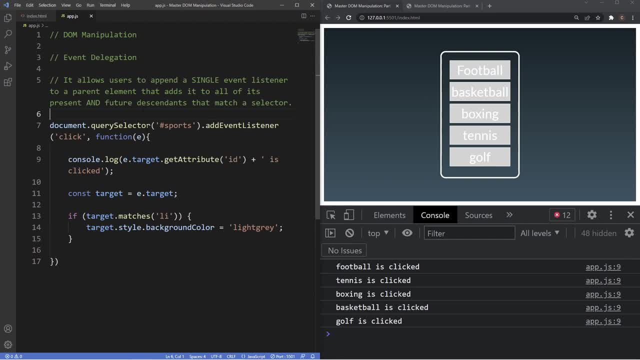 now, another crucial benefit of event delegation is the second part of our definition here. so the first part was it allows users to append a single event listener to a parent element that adds it to all of its present descendants. now the second part of this definition was that it also 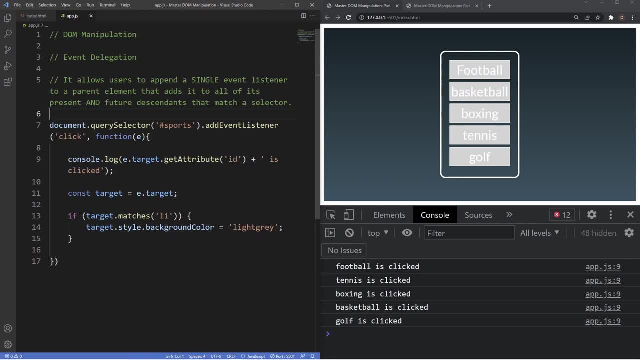 adds it to future descendants. that match, that selector, so this is actually in regard to dynamic elements. so let's just say we had an add button here at the end of this box where it allowed us to add another sport to our list. so let's actually just manually do this, um to show you guys exactly. 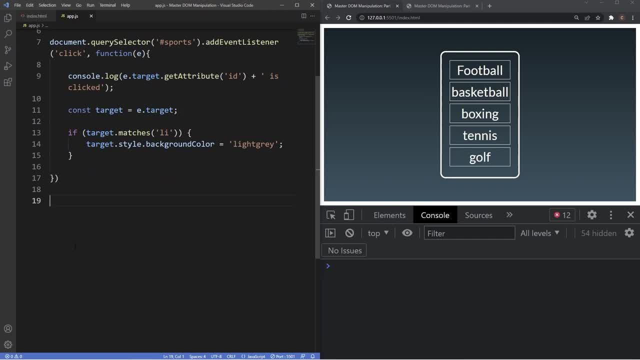 what i mean. so first we're just going to create a constant for our ul which has the idea of sports, so we'll say: const so: sports equals document. dot query selector. and then we'll just grab the id of sports again, which is that ul, and then what we'll also do is create another list item, so we'll say: const. new: sport equals document. 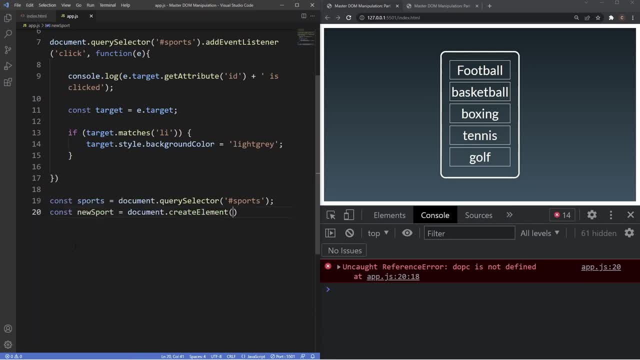 dot create element, and we'll create another list item. and then what we'll do is we'll say: new sport, so that variable, which is that new list item, uh, we'll give it uh in a text of: uh, let's say, let's make the sport rugby, and then we'll also give it the uh. 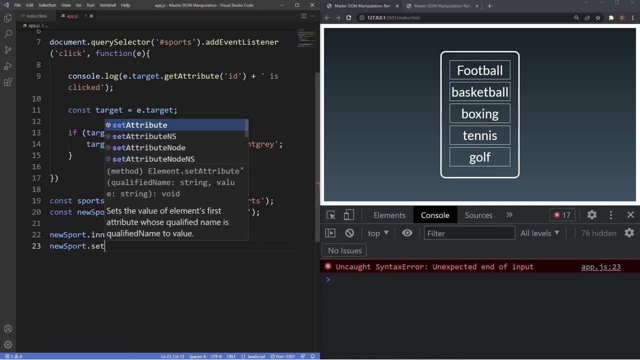 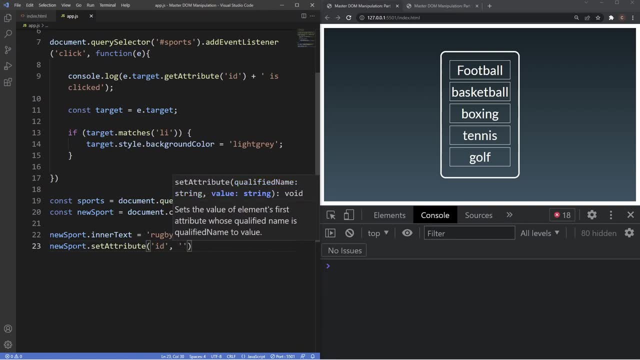 id of rugby. so we'll say set attribute- first an id attribute, and then we're gonna have the uh id of rugby, and then what we want to do is append this now to our list. so we'll grab the sports variable, which is the ul, and we'll say append. 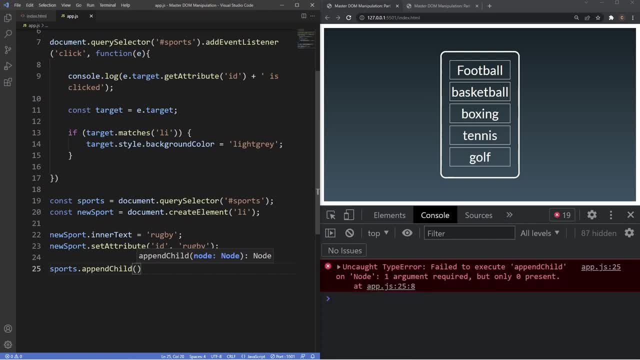 child. and then the child we want to append is, of course, that new sport. so when you say new sport, so as you can see now rugby has been added to our list here. so if i click on this, it's got the exact same styling and the output in the console, like the rest of the list items would. 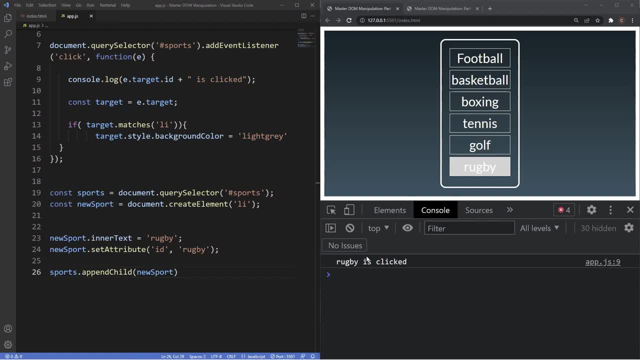 we now have an event listener to the parent, which is the ul, and, because of event delegation, we've delegated the event to the parent and, as you can see, this gives us the power to dynamically add new list items and those new list items will display the same behavior. so, again, without the 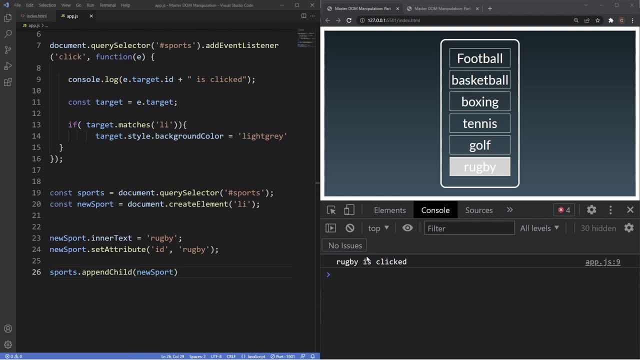 magic of event delegation. we'd have to use the method we previously used, where we'd have to include event listeners to each individual list items- and that includes any new list items that might get added on along the way, which will just clog up memory, effect performance and just create 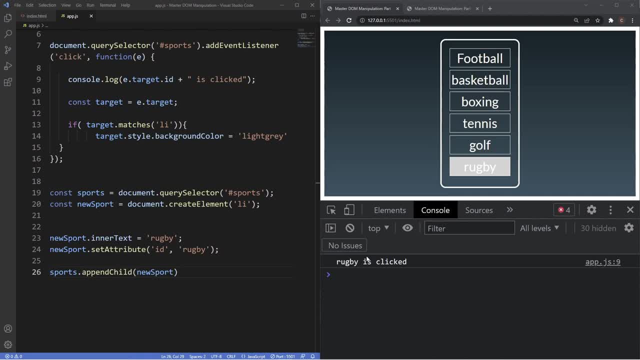 too much unnecessary code, so that's going to be it for this video. guys, i know it was a long one and there was a lot to take in, so well done if you made it this far. in part two of this two-part tutorial, we're going to be applying everything we learned now to practical examples, so i'll see you guys in the next video.